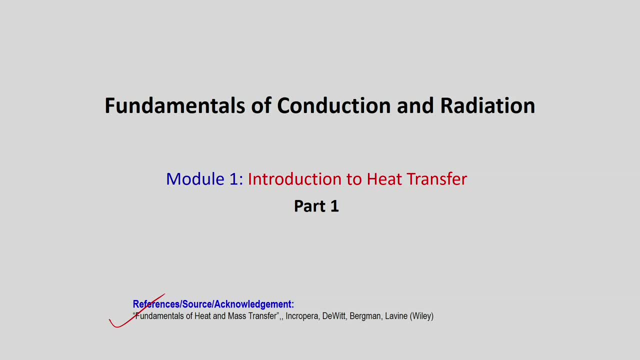 this particular textbooks and several of the illustrations that we are going to use while preparing these slides have already been taken from the soft copy of the same book. You must be knowing that heat transfer is one of the most fundamental and, at the same time, most applied subjects that you can identify in your entire course of mechanical engineering. 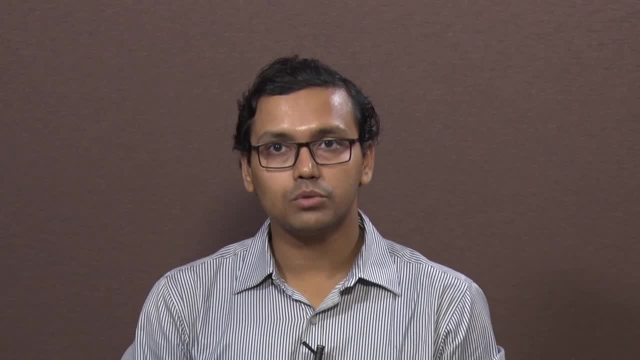 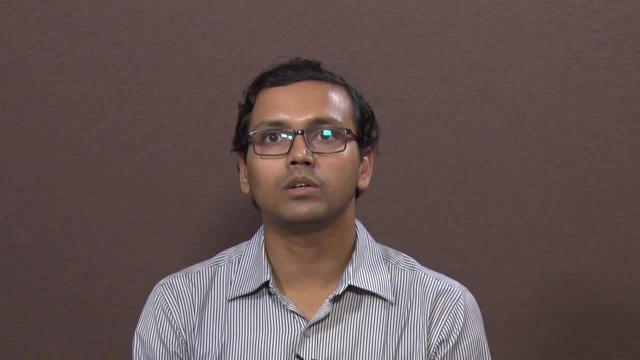 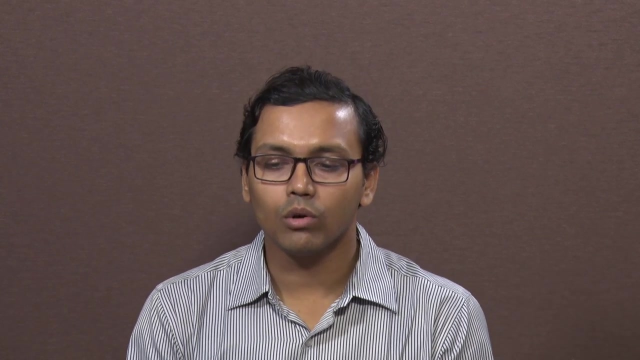 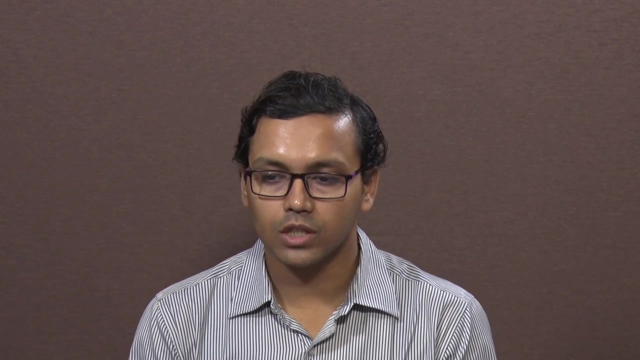 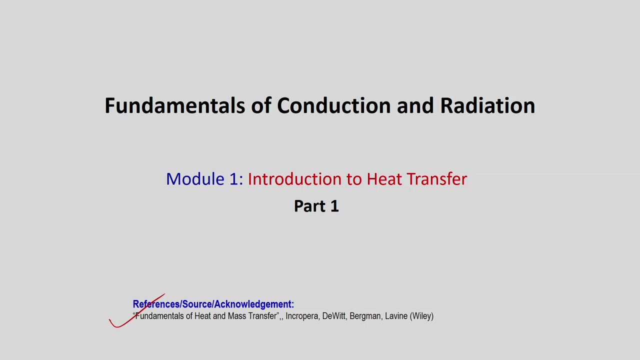 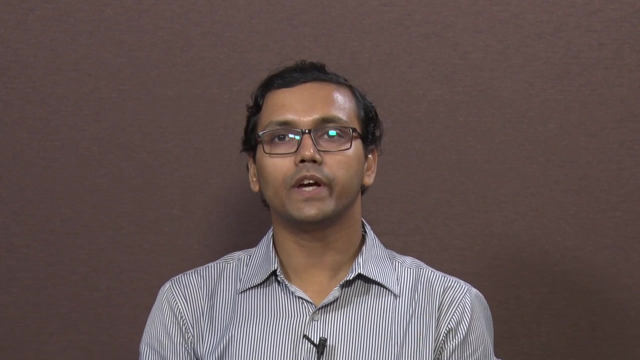 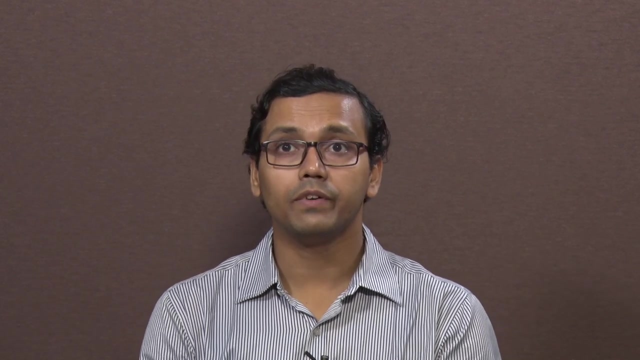 This course, I should clarify, is primarily aimed for the students of mechanical engineering, but students who are belonging to similar disciplines, something like power engineering or energy engineering, or maybe production manufacturing engineering or any such allied branches. All of those are still true, because both thermodynamics and fluid mechanics are the 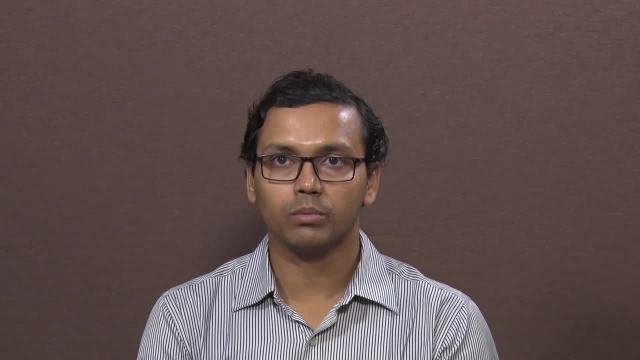 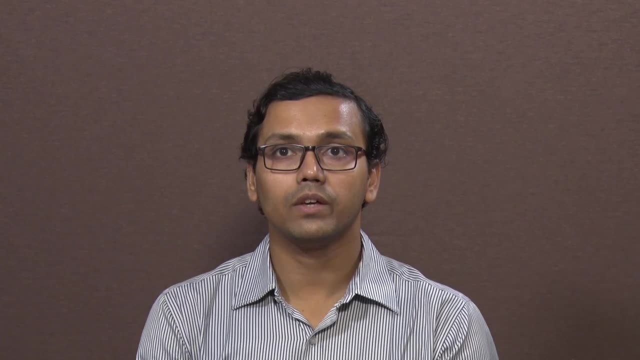 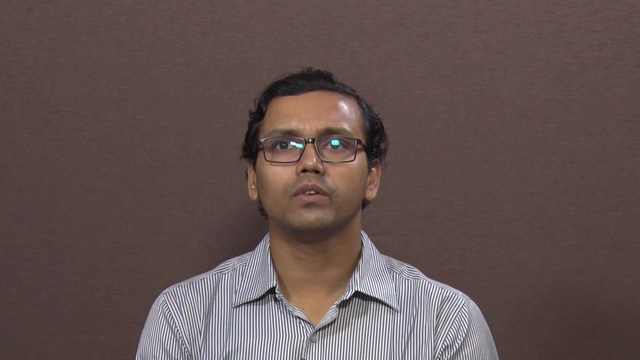 fundamental subjects, and heat transfer starts only with a background of thermodynamics, But still there are so many applications of heat transfer almost in every sphere of our life that you can also identify heat transfer as one of the fundamental subjects In every mode, starting from the mode of energy interaction that human body can have with. 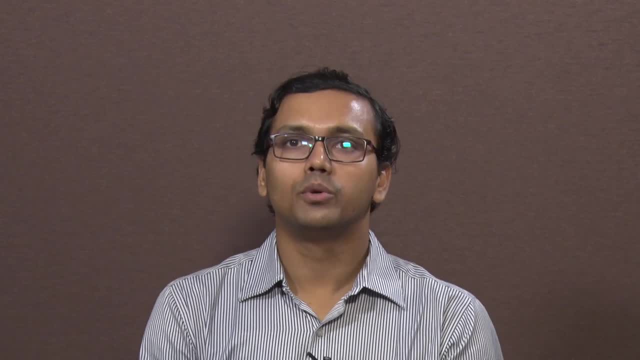 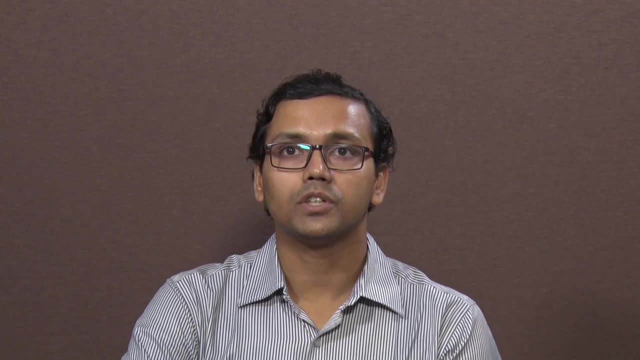 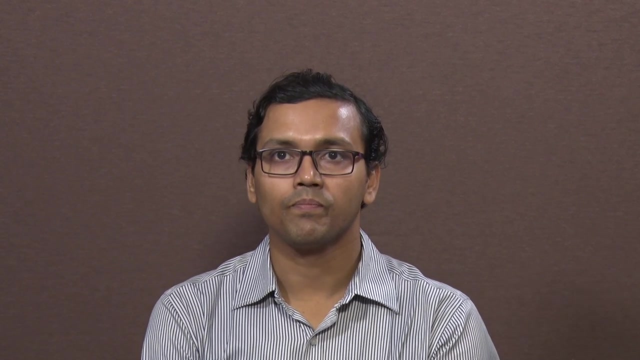 the surrounding to our day to day activities, like cooking, to very large scale industrial applications like nuclear power generations- everywhere you can identify some applications of heat transfer or to analyze such kind of systems. we need the understanding of different modes of heat transfer and that creates the backdrop for this course, where we are expecting 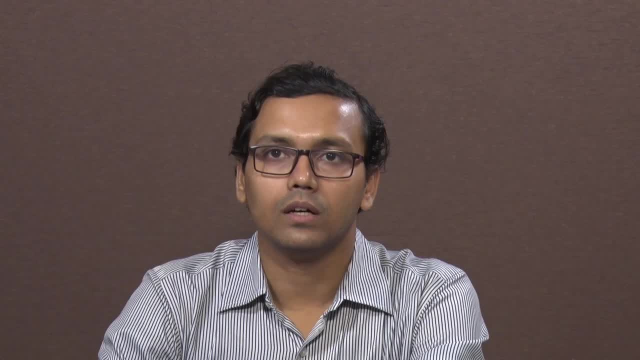 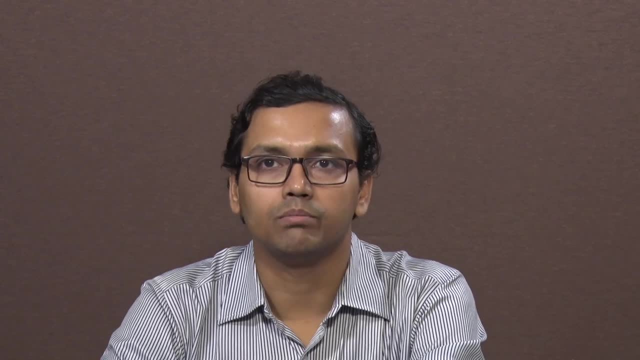 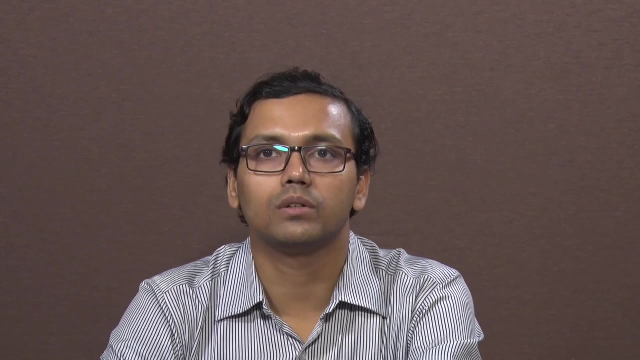 the audience to have a basic understanding of thermodynamics. Thermodynamics, you know that, is always taught either in the first year, or sometimes in the second year, maybe in the third semester of your engineering disciplines, and not only for students of mechanical engineering, rather students of several other disciplines also. 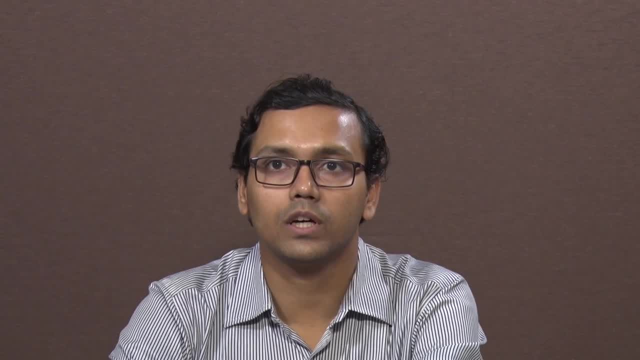 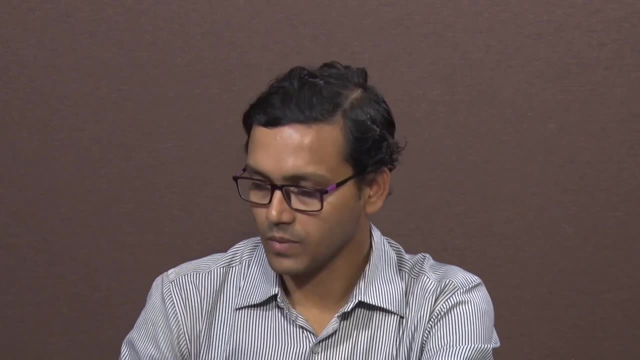 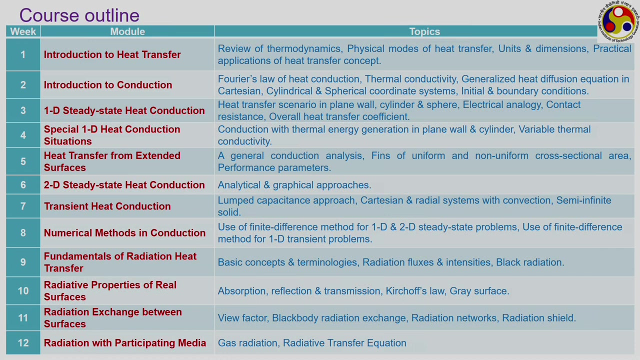 learn thermodynamics Now. once you have a brief background about the thermodynamics, then you can easily participate in this course, because we shall be starting from the very basics of the heat transfer. These are the course outline, which has already been displayed there. Now it is a 12-week course, 30 lectures or 30 hours. Accordingly, we have divided it into two parts. The first part is the heat transfer and the second part is the heat transfer. The second part is the heat transfer and the third part is the heat transfer. The third part is the heat transfer and the third part is the heat transfer. 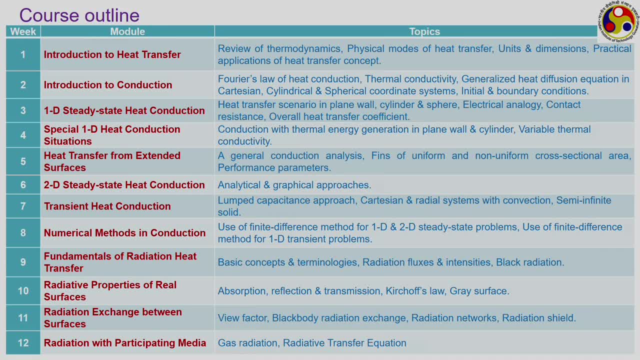 We have divided the entire syllabus into 12 modules. Out of them, module number 1 to 8 belongs to conduction, and the last four modules belongs to radiation. So up to this we have conduction, heat transfer. This is how we are going to go for in the first week, that is, in this week where we are. 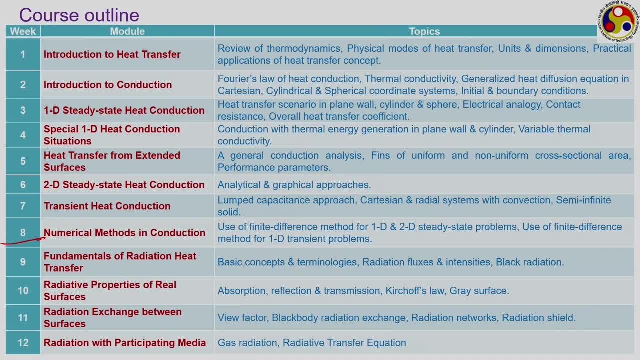 going to have just two lectures, two maybe a bit brief lectures, where we are just going to give you the introduction, reviewing the basics of thermodynamics, then mentioning about the physical modes of heat transfer, Possible units and dimensions and some practical applications of heat transfer concepts in 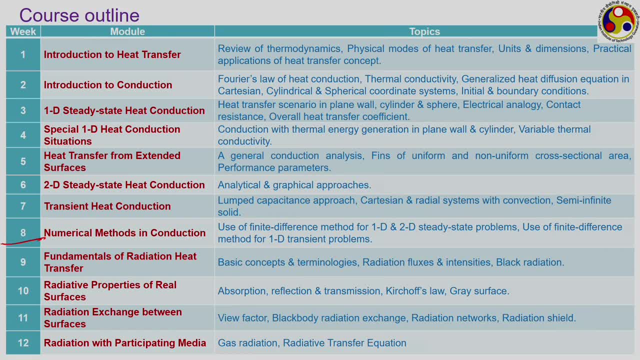 terms of practical applications and also some numerical examples. Then in the next week I shall be moving into the conduction, heat transfer, starting with the Fourier's law of heat conduction, mentioning about the thermal conductivity as a property. Then we shall be developing the generalized heat diffusion equation in all three possible 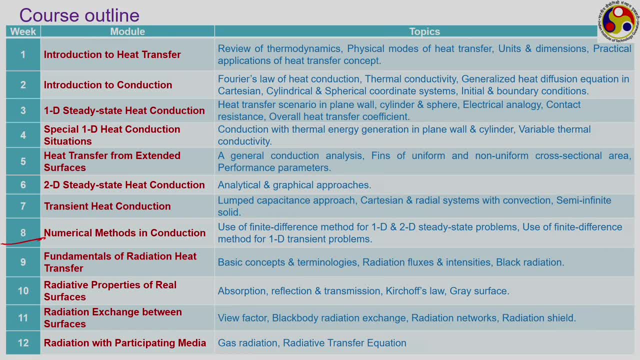 coordinate systems like Cartesian, cylindrical and spherical coordinate systems, and also we shall be talking about the boundary conditions required to solve such systems. Then in week number 3, we shall be using the one-dimensional versions of those equations under steady state. So in this 1D steady state, heat conduction, we shall be solving different heat transfer. 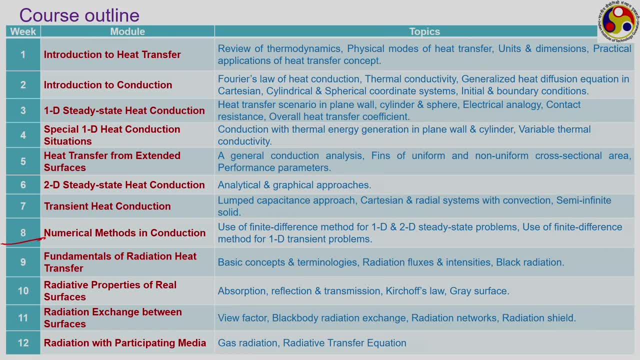 scenarios like heat transfer through plane walls, cylinders or spheres. We shall be seeing the electrical analogy of heat transfer. the topic or concept of contact resistance and also the overall heat transfer coefficient will be introduced. Then some special scenarios of 1D heat conduction situation will be discussed in week number. 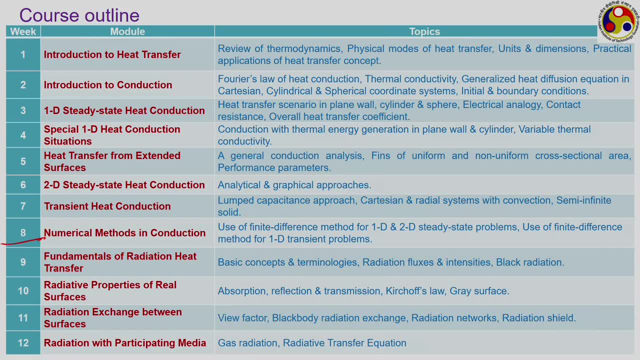 4. So thermal energy generation is involved in both plane, wall and cylinder, or where we are talking about a variable thermal conductivity system or a few more. let us see what we can go through. Then, week number 5,, we shall be moving to another application of 1D steady state heat. 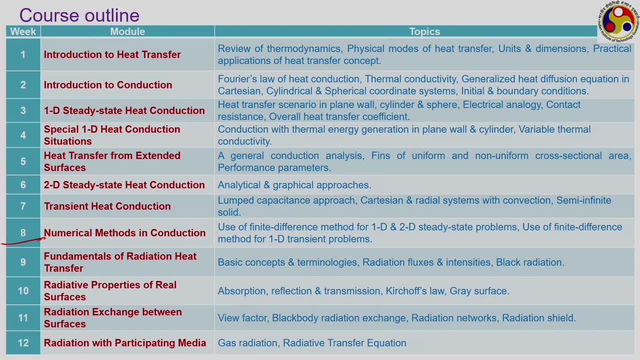 conduction, that is in terms of the extended surfaces or fins where a general conduction analysis will be given. Then different kinds of fins will be introduced. fins of both uniform and non-uniform cross-section areas will be analyzed. Then, in week number 6, we shall be moving to the two-dimension steady state heat conduction. 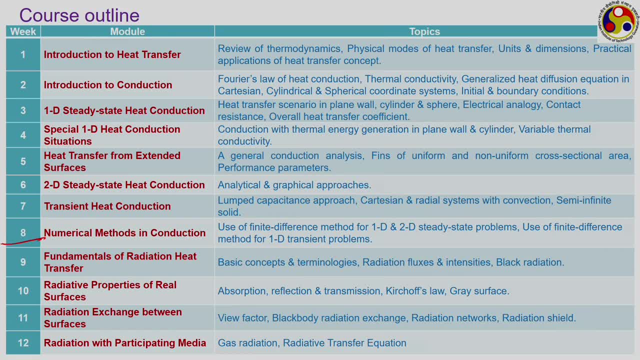 in terms of both analytical and graphical approaches. Week number 7, we shall be talking about the transient heat conduction, primarily in one dimension, where the lump capacitance approach will be followed, Then Cartesian and radial systems with convection and very important concept of the semi-infinite. 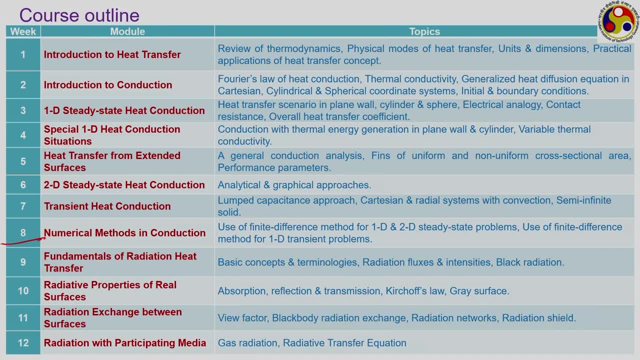 solid will be introduced and in week number 8, we shall be reviewing some numerical methods which are associated with the conduction heat transfer simulations. Thank you, Primarily, the finite difference method for both 1D and 2D steady state problems will 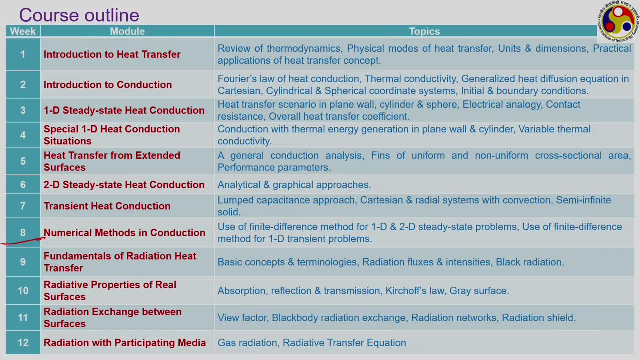 be discussed in terms of numerical methods or numerical problems. Then use of finite difference method for 1D transient problems will also be discussed. That will cap up our discussion on conduction. Then, in week number 9, we shall be moving to radiation, where first the fundamental concepts, 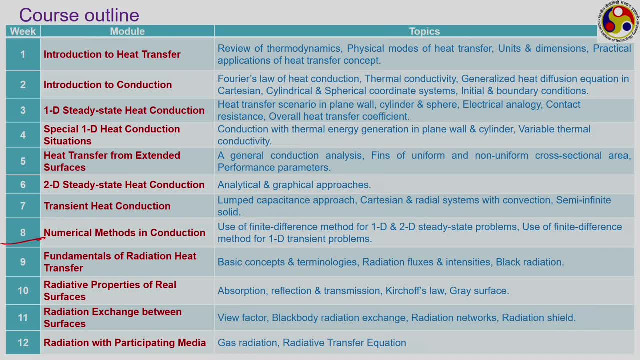 of radiation will be introduced in terms of different terminologies, different kinds of radiation, fluxes and intensities, And also the concept of binomia, black body or black radiation, and also the grey surfaces will be introduced. Then, in week 10,, we shall be talking about the radiative properties of real surfaces. 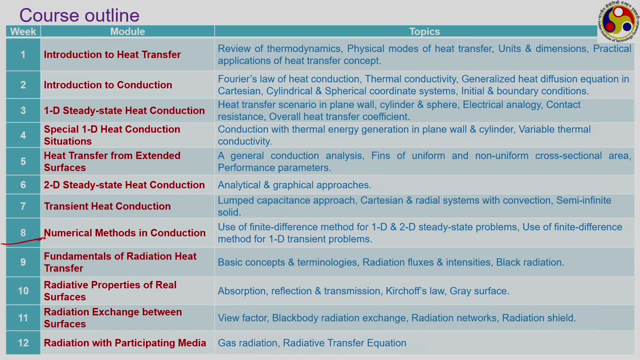 like absorptivity, reflectivity and transmittivity, The Kirchhoff's law also will be coming into picture. Grey surface I have just mentioned in week number 9 we can cover, or we can also cover this one in week number 10, because that is more a property of real surfaces. 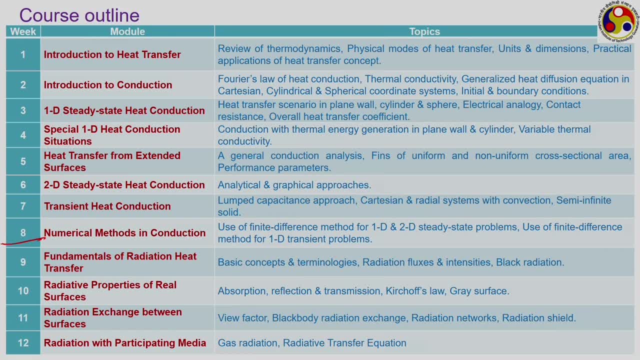 Then in week number 11, we shall be talking about the radiative exchanges between surfaces. as we already have discussed about the properties that individual real surfaces can have, Then it is much easier to discuss about the exchange that multiple surfaces can have, the concept. 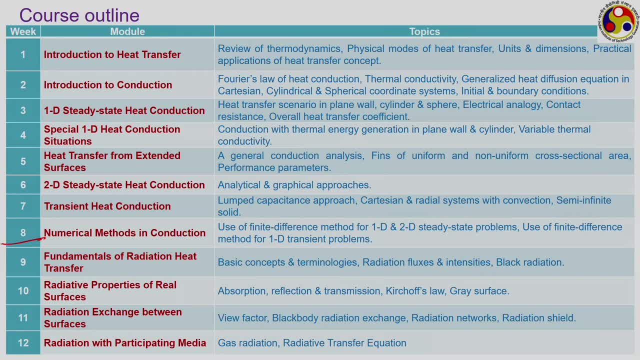 of view factor, black body radiation exchange and the concept of radiation network will be introduced. And finally, radiation with participating media, in terms of gas radiation and radiative transport equation will be discussed. to round off the entire course Here, as there are 12 weeks, both of your instructors will be participating. 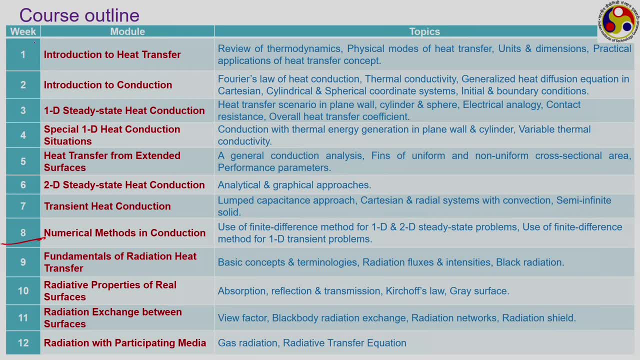 Participating in 6 of the weeks. like I, shall be your instructor for week number 1 to 4.. Then Professor Dalal will be talking about week number 5 to 8.. Then I shall be back with the fundamentals of radiation in week number 9 and 10.. And Professor Dalal will be discussing. 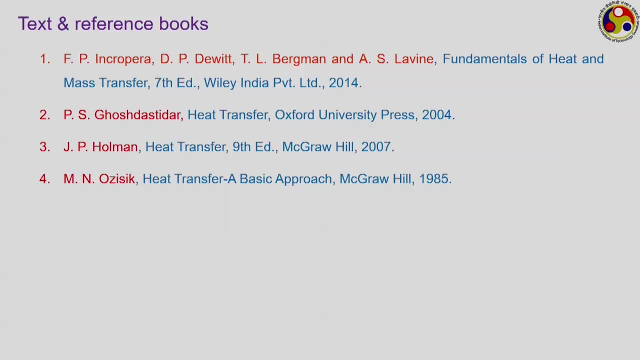 about week number 11 and 12 to round off the course. These are the text and reference books that we are going to follow in this course. As I have mentioned, the first one is the most important book followed worldwide by Professor Dalal. 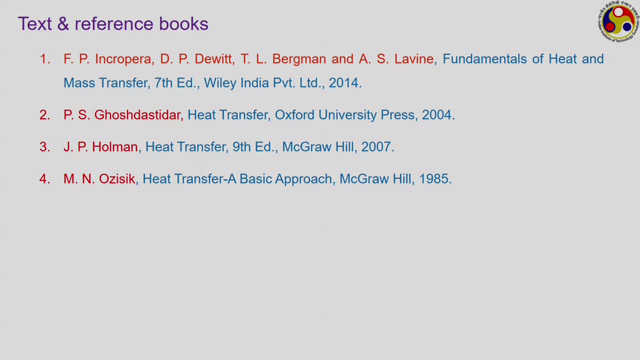 I have mentioned here the seventh edition, but probably there is a higher edition already available in the market or you can go to some older edition also. just see whatever you can have, And this is one book which probably you should have in your personal collection as well. Cheap Indian versions, or I should say not so expensive Indian versions, are available. 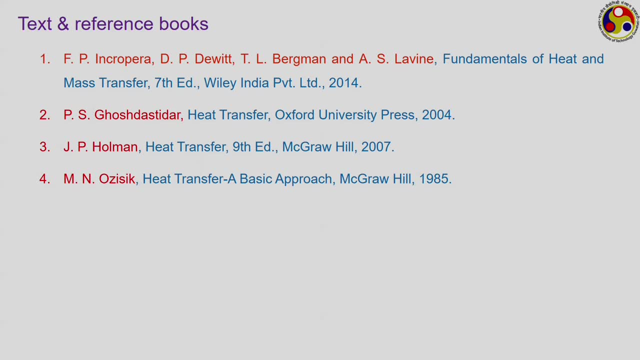 So probably you can have a copy of this book for your own collection. The other three are also very good. book on fundamental of surface. Want to get to know more about my particular books about the height of temperature and snow cloud. your operationalization in shooting. this series can continue till the end of the 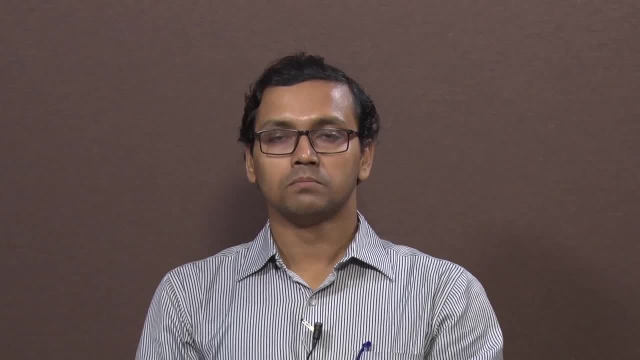 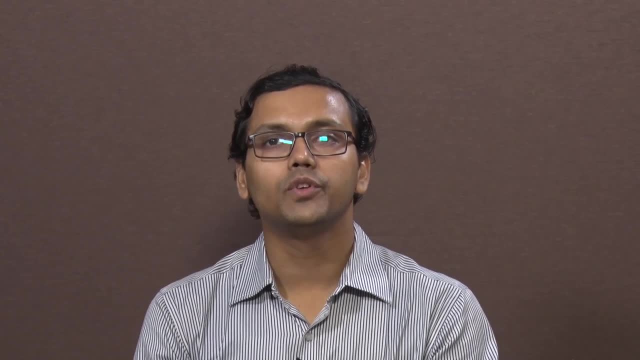 course, if you want to know more about what will happen, that have been discussed. Now the major project in our쪽 page which we want to discuss is theire. more volume earlier than the lecture we have seen right from doing the same picture, So please do read. 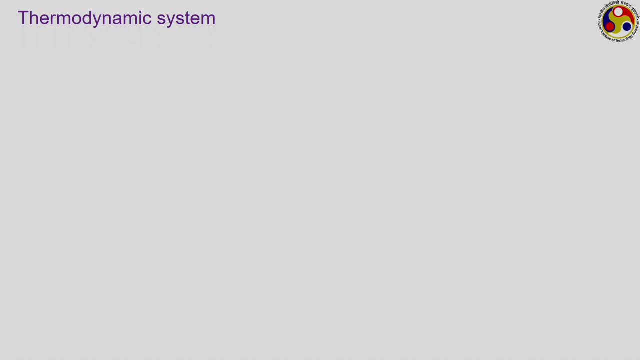 that and make sure to know that, above that, I have inc прив покues here for the first session which is neccesarily compiled Now. takoикse viene bye is an introduction video about source analysis in thermal energy. Number 6, thermal energy integration system. You all may or may not believe that there is a 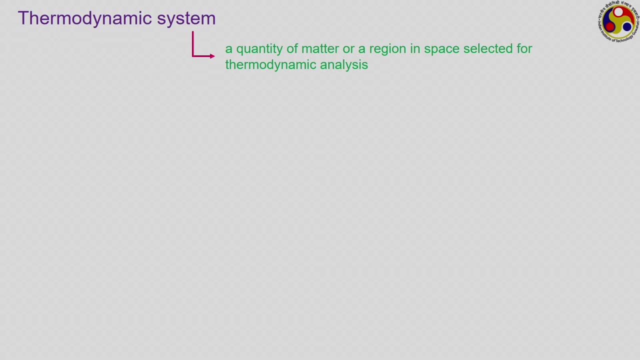 whole range of 사고lau discussable technologies used at that level, and that one thing may not be of matter or a region in space selected for thermodynamic analysis. That is, this is basically the object where we want to perform the analysis. Now, your object can be a quantity of matter. 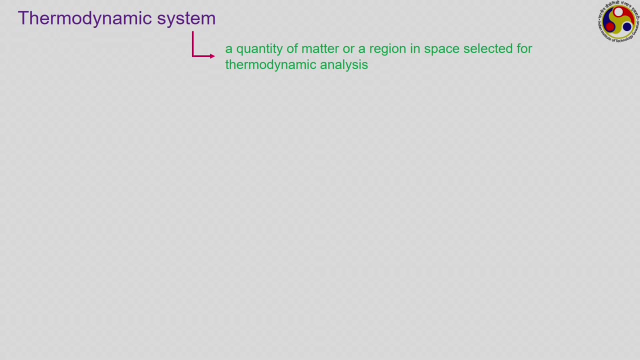 or mass, or it can be just a space, Just like an example that is given here. Here, the one identified by the blue color is the system, because that is our focus. The dark purple line which is surrounding the system is known as the boundary. So this is a system, boundary and everything outside the system. 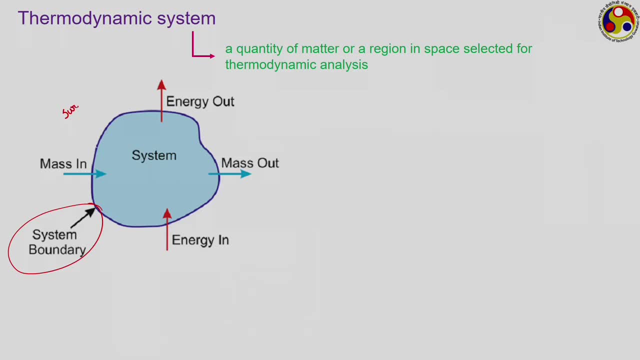 is referred as the surrounding, So anything outside the system is called the surrounding. Now, this boundary of the system can be real one or can be an imaginary one. Your boundary can be a fixed one, thereby fixing up the volume of the system, or it can be a movable one. 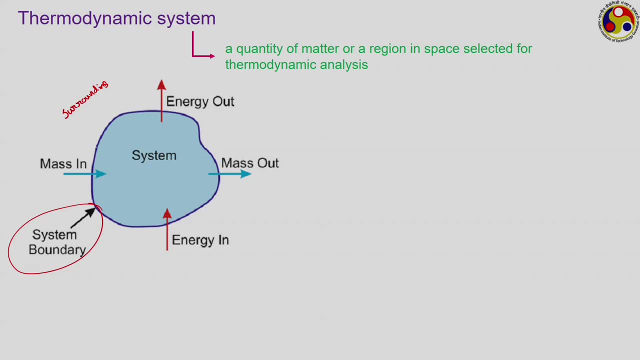 So that the volume of the system can keep on changing. It can be rigid or flexible one as well And accordingly, our choice of system can be quite flexible. and for the same system we can- or, sorry, for the same scenario we can- have different choices of system and depending upon your choice of 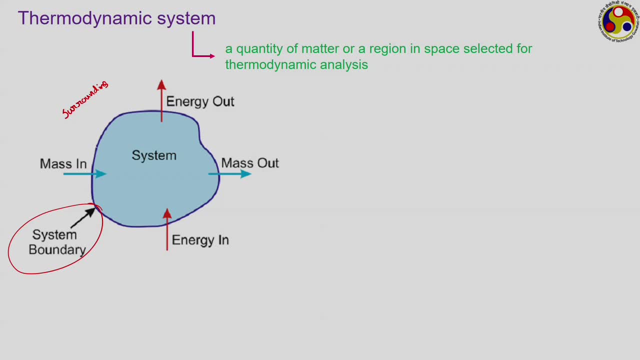 system. the interaction between system and surrounding can vary. And what are those interactions? The interactions are primarily in the mode of either mass or energy, or maybe both. So mass can enter the system from surrounding or can leave the system to move to the surrounding. Similarly, energy can also move in or out of the system. Accordingly, 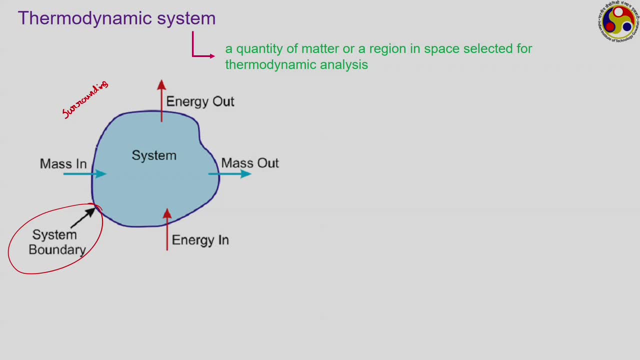 the total energy content and mass content of the system can change Now depending upon the nature of the interactions between system and surrounding. we can classify systems into two categories: closed systems or control mass system, and open system or control volume system. For closed system there is only mass interaction. sorry for closed system there. 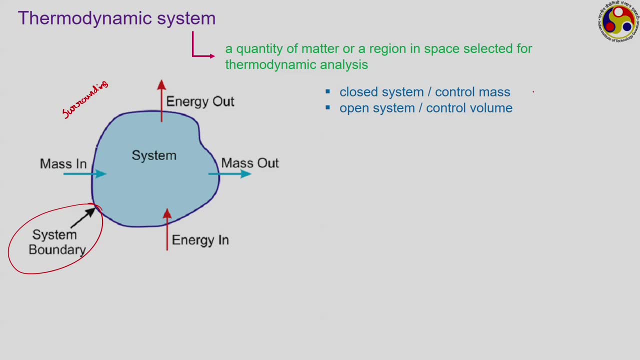 is only energy interaction. there is no mass interaction. That is, we can have energy interaction, definitely, but no mass interaction. for closed system, whereas for open system, mass is allowed to move in or out of the system. Therefore, for an open system, we can have both energy interaction and mass interaction as well. 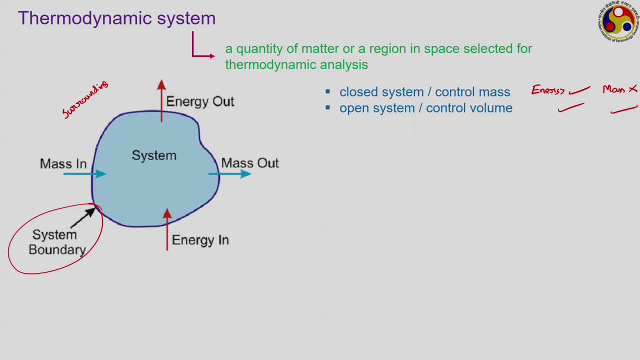 Now there can be another kind of system that can be defined. in certain textbooks of thermodynamics that is identified as a third kind of system But truly speaking it is not defined in the same way. So the third kind of system that that can be identified just as a special case of closed system, which is referred as the 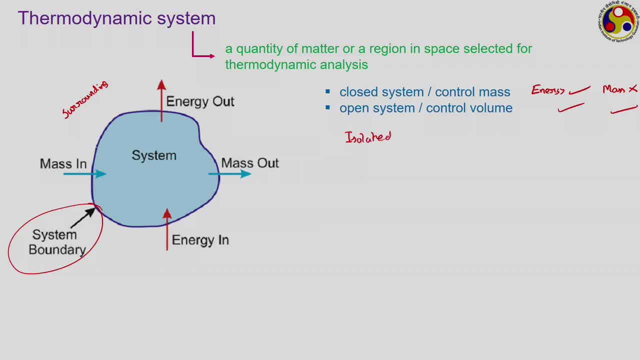 isolated system. An isolated system is a special case of closed system which does not have any energy interaction as well. Mass interaction is already not there for closed system. energy interaction is also not there. then we shall be calling it an isolated system. So an isolated system is completely. 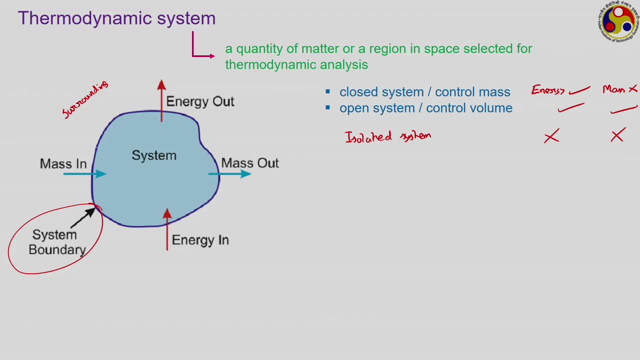 separated from its surrounding, it does not have any interaction at all the surrounding. Now for a closed system, as there is no mass interaction. so the mass of a closed system remains constant. so accordingly we call it a control mass also, Whereas for an open system, 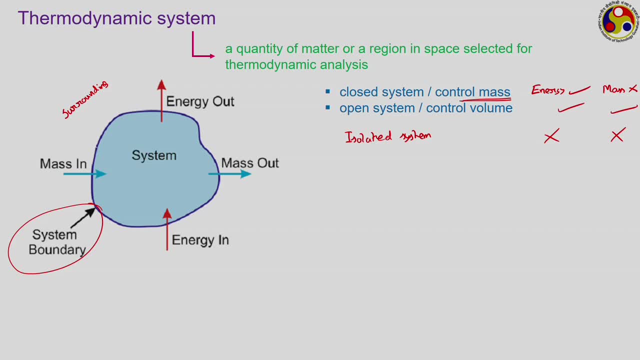 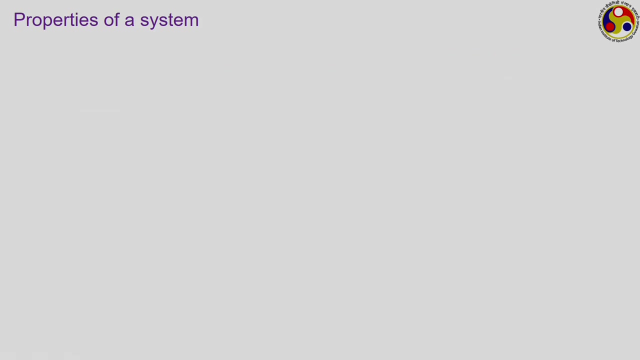 the mass of content of an open system can change, but generally not an universal rule, but commonly open systems are associated with a rigid boundary so that their volume remains constant, and that is why open systems are often referred as control volume systems as well. Now, to quantify, or rather to identify, the physical condition of a system, we need to 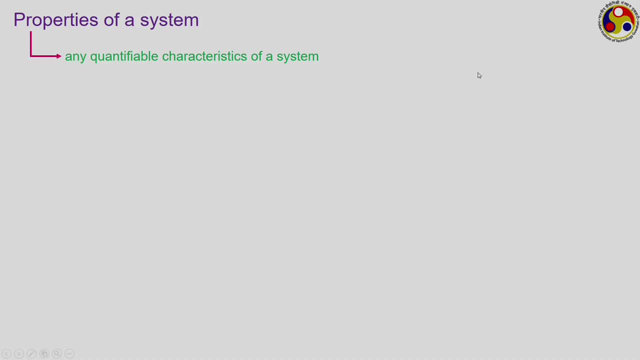 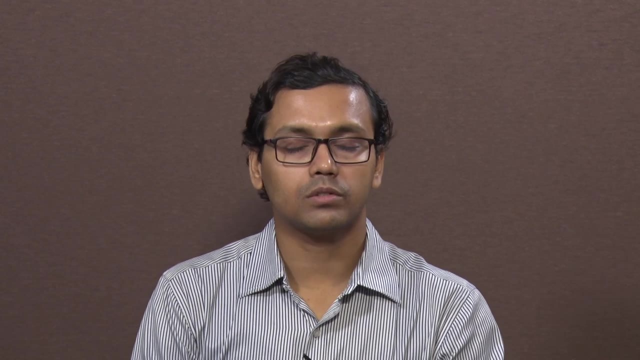 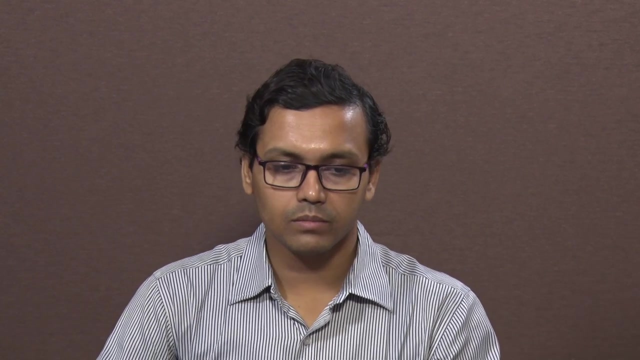 define the properties. Properties are any quantifiable characteristics of a system. So anything that you can visualize which can be or, sorry- anything that you can think about which can be quantified can be identified as a property. And properties can be classified into two categories: intensive and extensive. 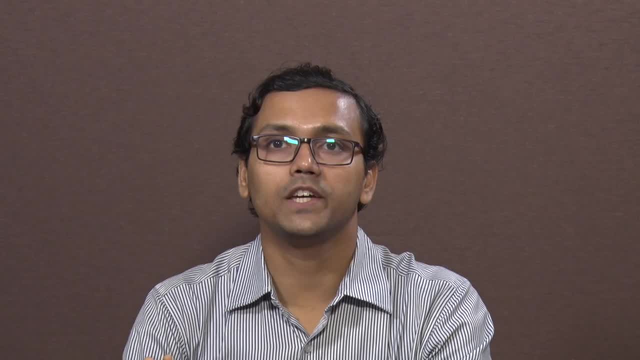 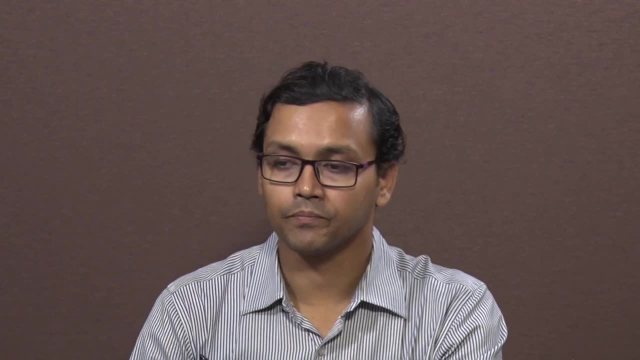 Intensive. So these properties which are independent of the mass or size or extent of the system, whereas extensive properties are dependent on the mass or size or the extent of the system. Now for a given property. how can you identify whether it is intensive or extensive? This 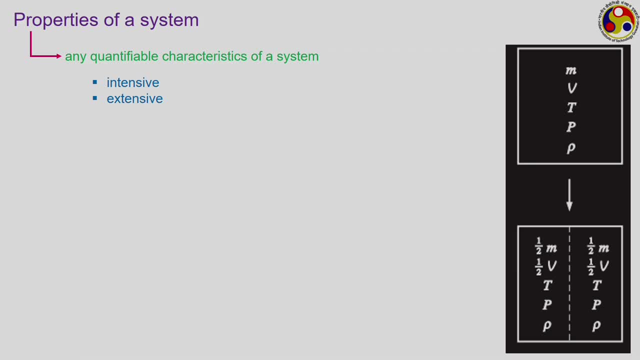 is a simple example. Suppose we have a system given for which there are several properties mentioned, like M for mass capital, P for the volume, capital T for the absolute temperature, capital P for pressure and rho for density. These are the 5 properties that are specified. 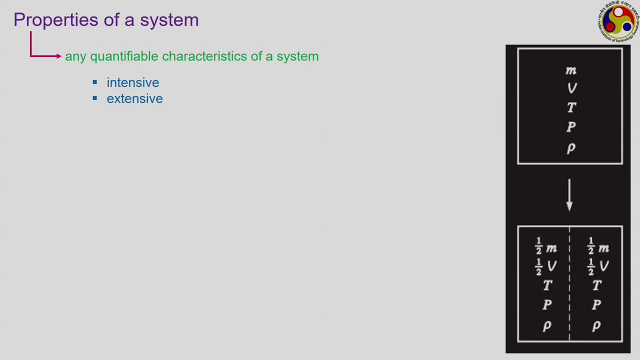 for the systems and we have to identify, out of this, 5 properties which are intensive in nature and which are extensive in nature. The easiest way of doing this is to divide the system into 2 subsystems of equal volume. I should say the system should be divided. 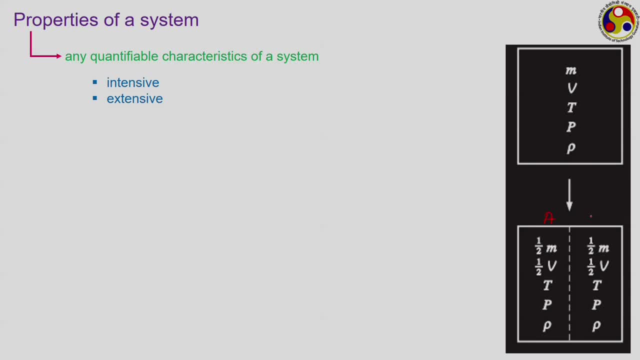 into 2 equal compartments. Let us say: this is your system A, this is your system B, and now we have to check the properties for both the systems. Now the, or you can just, instead of both of them, you can just look at any one of the subsystems as well. 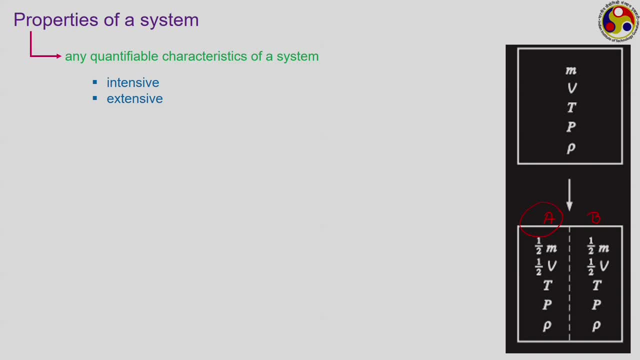 Let us just look at the subsystem A and compare which of the properties of the subsystem is the same as the original system: Temperature, pressure and density. these 3 remains the same. So they are intensive properties because they are independent of the mass or size of 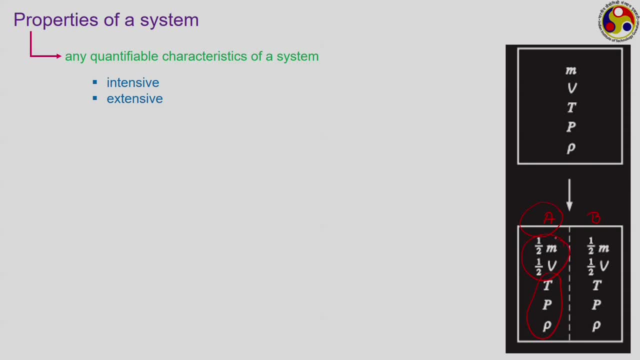 the system, Whereas mass and volume, they are intensive properties and because of that their values are changing, because of the, because of subdividing the system into 2 compartments. So examples of intensive properties. then we can write: as mass- mass itself is an extensive property- the small m volume which we can find here. 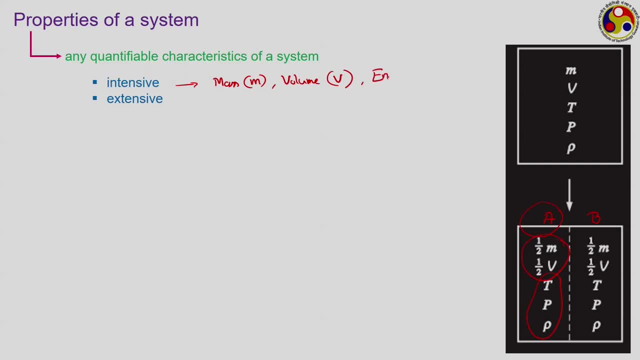 Generally capital V is used for volume. We can have energy as another very common property. Okay, So, as you have already done a course on thermodynamics, so you know terms like enthalpy, entropy. they are all capital S, they are all extensive properties, Whereas if we want to write intensive, 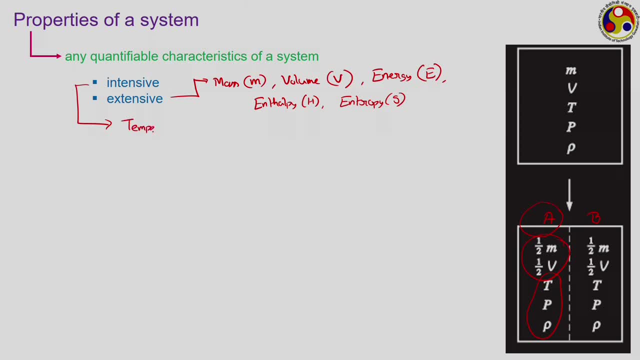 properties, what we can write. We can think about temperature, temperature, temperature, temperature. Okay, So it can be written like this. So if we want to write say pressure, say density, in the example these 3 are already there for intensive properties Generally used for. 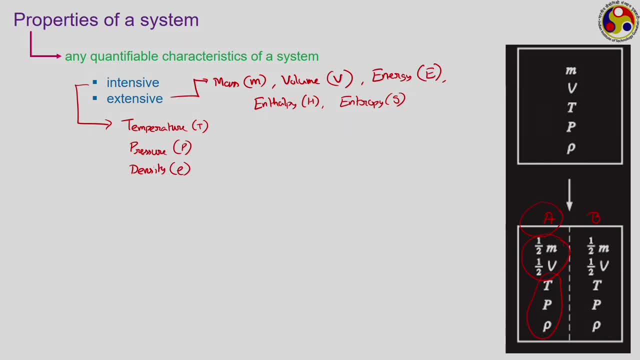 rho. You can identify several others also, like you have done course on sorry course on fluid mechanics. From there you can identify properties, something like say viscosity, which generally specified by mu. Okay, In thermodynamics. also you can identify specific heat Generally. 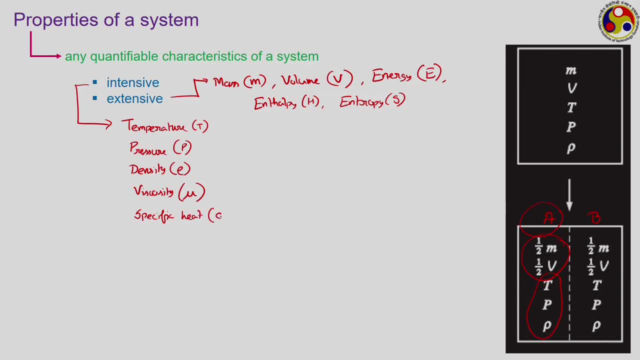 give you some details, So it can be written like this: Okay, So I have already given all the features of the system, So I think this is it. So this how we should discuss. generally given by small c, cp or cv, these are all intensive properties because they 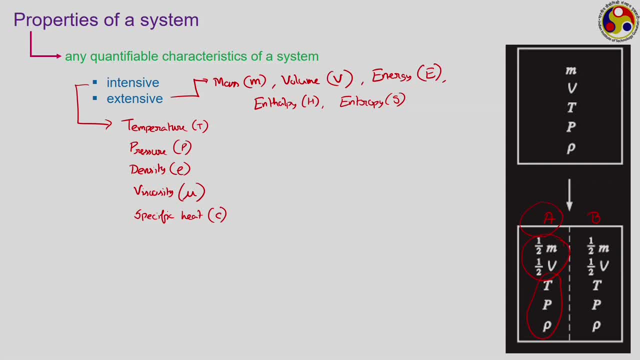 are not dependent upon the size or extent or mass of the system. Also another thing: you must be knowing by now: that any extensive property per unit mass is an intensive property. Say for example energy, total energy content of the system. if that is divided by mass, then 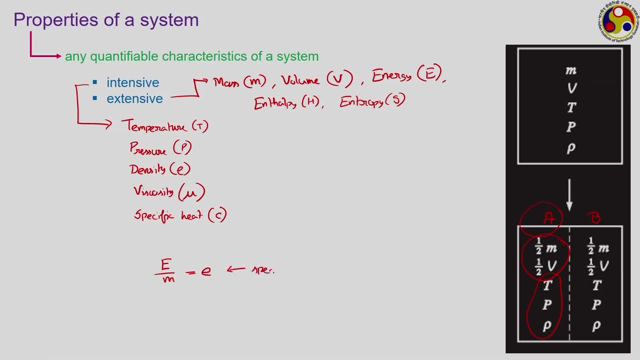 whatever we get, that is generally called specific energy. Any extensive property per unit mass is identified as a specific version of the same property, and this specific version of the properties are intensive in nature As it has already been divided by mass, so its magnitude will be independent of the mass. 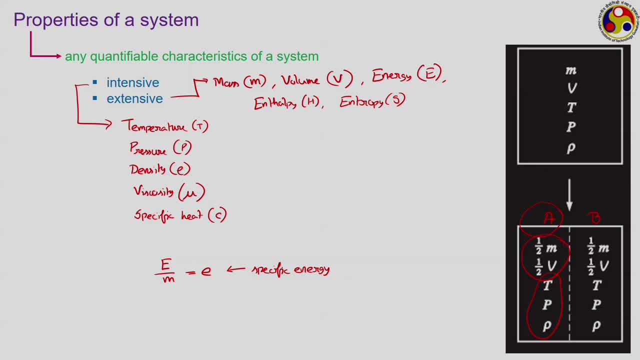 and therefore this is a specific property and an intensive property. Similarly, enthalpy per unit mass. So this is a specific property and an intensive property. So this is a specific property and an extensive property. The mass per unit mass, which gives us specific enthalpy, or entropy per unit mass, which gives 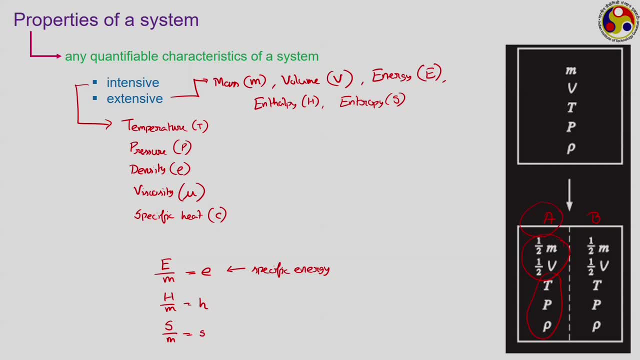 us specific entropy. they are all intensive properties. So extensive property per unit mass gives us intensive properties and also from the notations that we are using, you probably can identify that extensive properties are commonly written using capital letters, whereas intensive properties are commonly written. 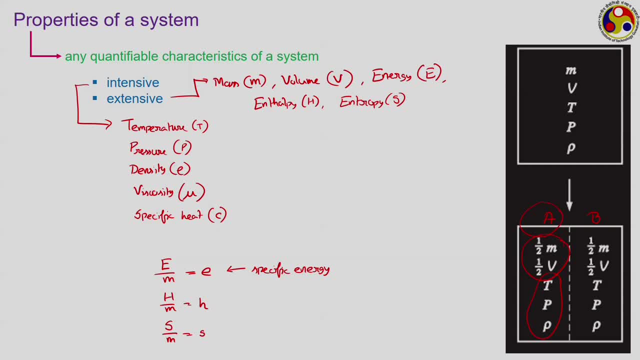 using small letters. Exceptions like mass: despite mass being an extensive property, we generally use small m to denote that temperature. they are intensive properties but still we use generally capital T and capital P respectively to denote them. But for other properties generally this rule is followed. 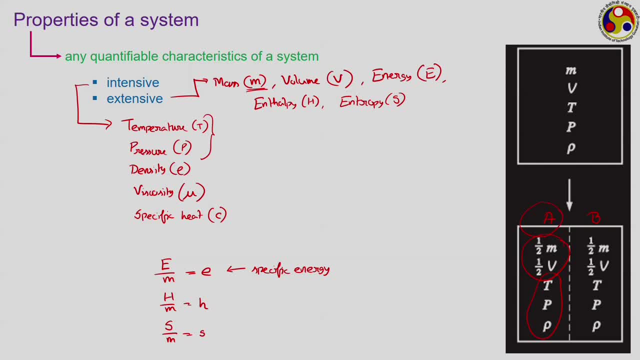 that is, capital letter to designate extensive properties and small letter to designate intensive properties. Now, among all this kind of properties, there can be infinite number of properties that you can identify for a given system, and also, I should mention at this particular point itself, this term quantifiable is very important for something to be identified as a property. 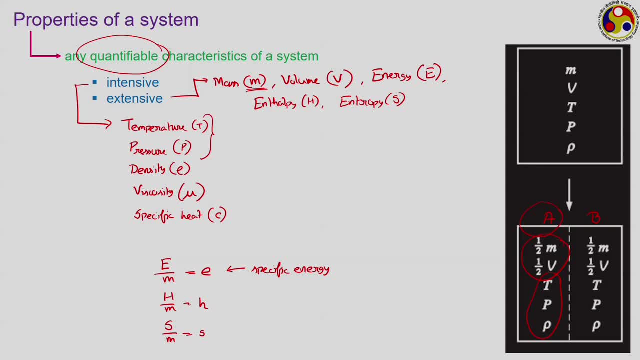 Like, say, if we talk about colour, is colour a property? Probably not from thermodynamic point of view, because colour cannot be quantified. that is more. that is something that can be realised more from perception or maybe taste of something. that is not a thermodynamic property. 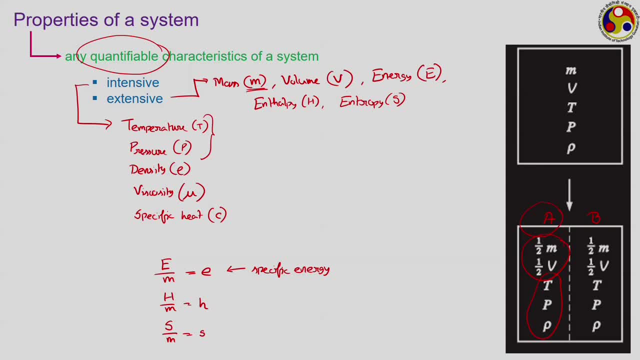 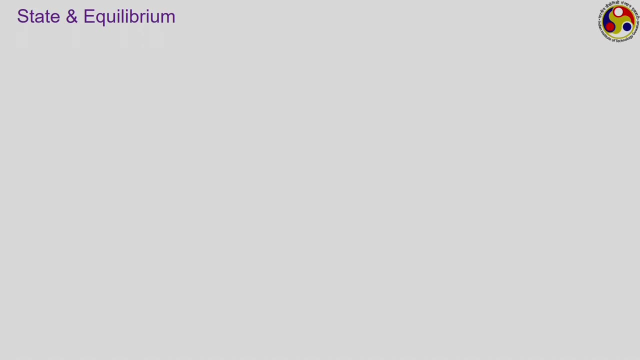 because these are more like perceptions, they cannot be quantified truly, So they are not properties. Now, among all these properties, one property is of particular importance from heat transfer point of view, that is energy. But before moving on, Now moving on to the energy, we have to mention about the state and equilibrium. Now, what? 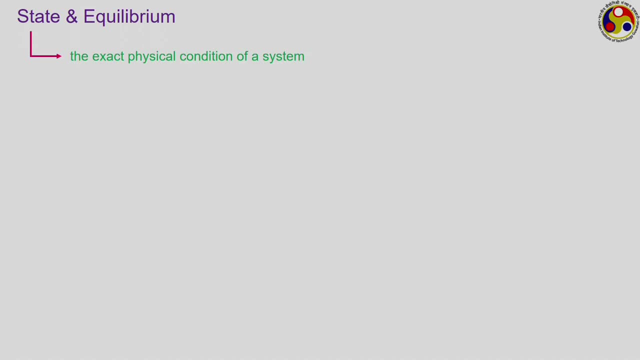 is state. State is the exact physical condition of a system, and to specify the state of a system we need to know all the properties of the system. Once we mention that a system is at a particular state, that means all the property values are known, or at least they. 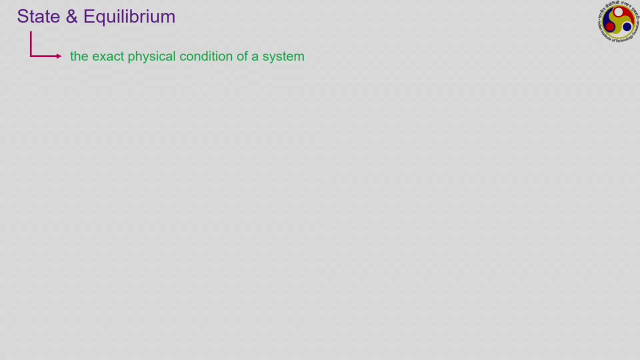 are fixed at a particular, at some concerned, magnitudes. If the magnitude of any of a single property changes, then the system moves to a different state point, And in thermodynamics we always deal with equilibrium states. Equilibrium state means there is no unbalanced potential. Now there are several kinds of equilibrium we can talk. 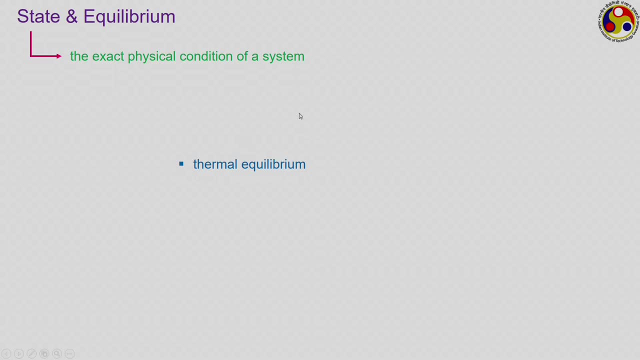 about. The first one is thermal equilibrium. Thermal equilibrium means within the system the temperature is same everywhere and therefore there is no heat transfer that is taking place. So thermal equilibrium is concerned with the equality of temperature. Similarly we talk about mechanical equilibrium. Mechanical equilibrium generally is associated with the pressure or 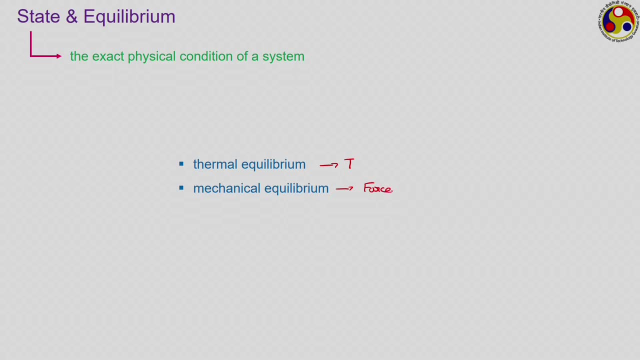 Or you can say it is associated with the equilibrium of forces. Mechanical equilibrium, however, does not mean that your pressure has to be same everywhere, Like if we talk about, say, this is a tank filled with liquid water. this portion is open to atmosphere. Now you must be knowing from your knowledge of fluid mechanics that, as we are moving downwards, 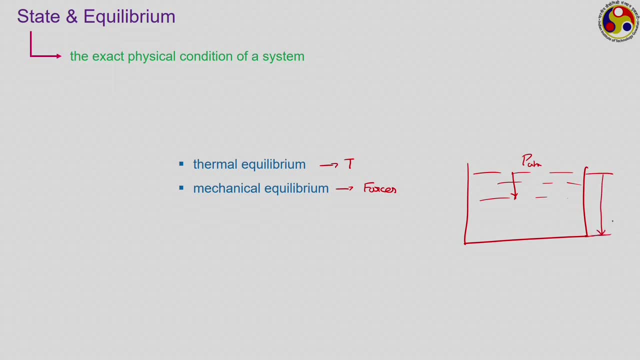 pressure keeps on increasing, and if the height of this liquid column is h, then the pressure at this bottom surface will be the atmospheric pressure plus rho gh. Now, as the pressure is changing in the vertically downward direction, then is the system in mechanical equilibrium. 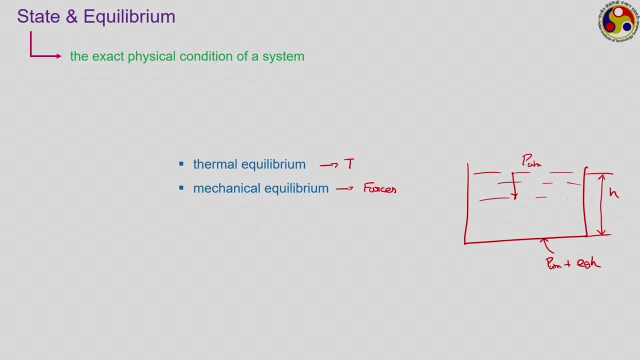 Probably it is, because here there is no unbalanced forces. The gravitational force is being balanced by this pressure distribution and that is why the system is in mechanical equilibrium. Third is the phase equilibrium. Phase equilibrium refers to the equality of phases, Like, if we are talking about the equilibrium of the phase equilibrium, then the equilibrium 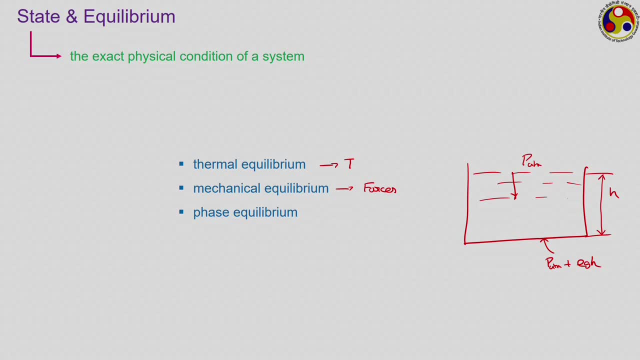 of the phase equilibrium remains constant. If we are talking about a system which is having multiple phases, none of the phases are changing or their proportions remains constant, then we call the system to be in phase equilibrium. Like: suppose you take a mixture of liquid water and ice at 0 degree Celsius and put 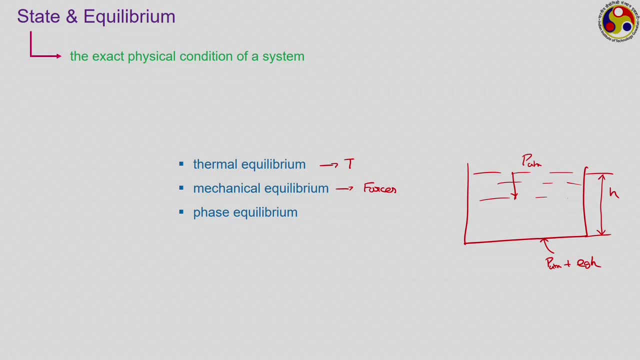 that mixture into a thermoflux which is perfectly insulated. Then we can expect that the fraction of mass occupied by the solid and fraction of mass occupied by the liquid that remains constant over infinite period of time. Then we should call that system to be in phase equilibrium. 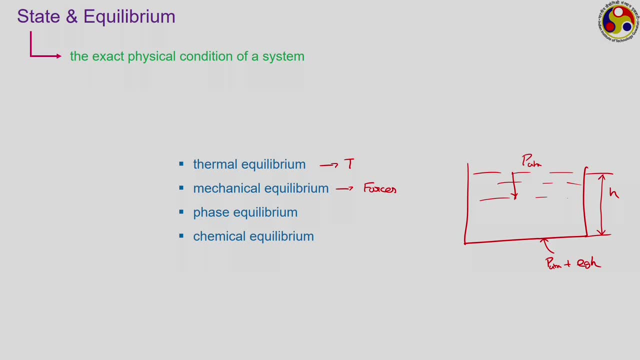 And finally in chemical equilibrium, Which refers that the chemical composition of the system remains unchanged. That means there is no chemical reaction going on, So there is no chemical reaction potential. And when all these are satisfied, then we call the system to be in thermodynamic equilibrium. 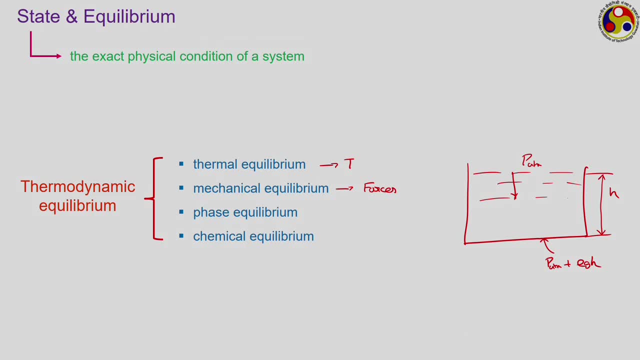 Now, whatever you have learned in thermodynamics, they are always concerned about the equilibrium state, Like when you represent any process on a property diagram. let us plot a property diagram where any standard diagram. So we have a PV diagram. So this is our state, point 1.. 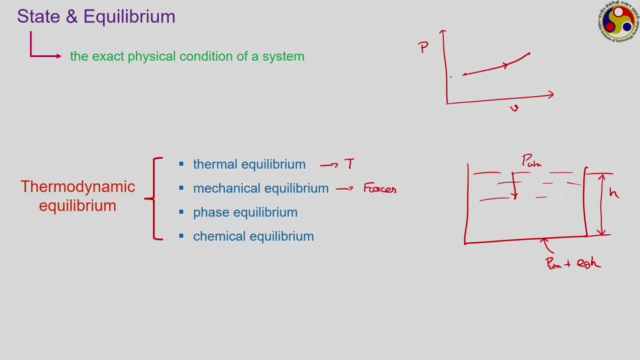 This is our state point 2.. And let us say this is a process that is going on from state 1 to state 2.. Now can you tell me under which situation we can represent the process by a continuous line like this? We can represent this one when, starting from point 1 to point 2, the infinite number of 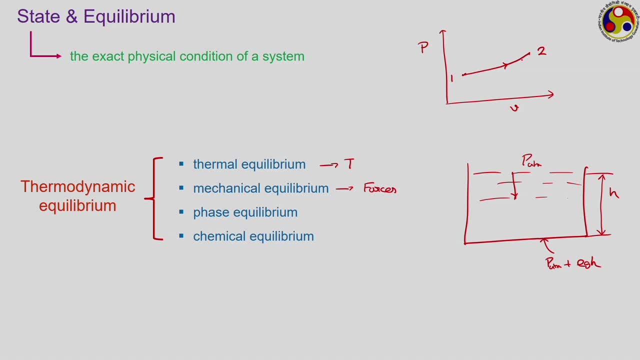 points, which constitutes this line. All of them are in equilibrium and we have complete knowledge about each of them. That is why the term generally quasi-equilibrium is used. So this is our state point 1.. This is our state point 2.. 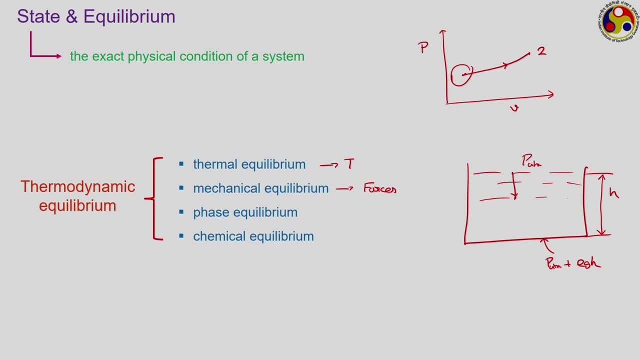 or quasi-static are also commonly used. So state 1 is an equilibrium state, state 2 is also an equilibrium state and all these intermediate states. they may not be in perfect equilibrium but they are in quasi-equilibrium condition, that is, they are very close to an equilibrium. 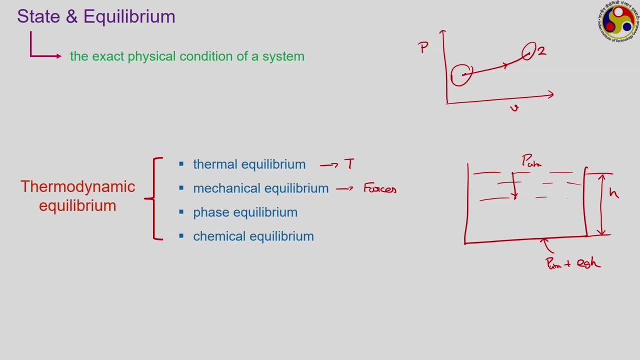 state. So your entire study of thermodynamics was based upon this concept of thermodynamic equilibrium, and that is where the difference with heat transfer comes into picture. If a system is in thermodynamic equilibrium, then it is also in thermal equilibrium. that is, the temperature everywhere in the system is constant. and if the temperature is constant, 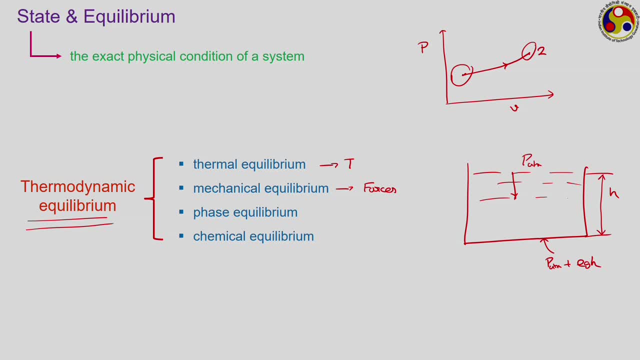 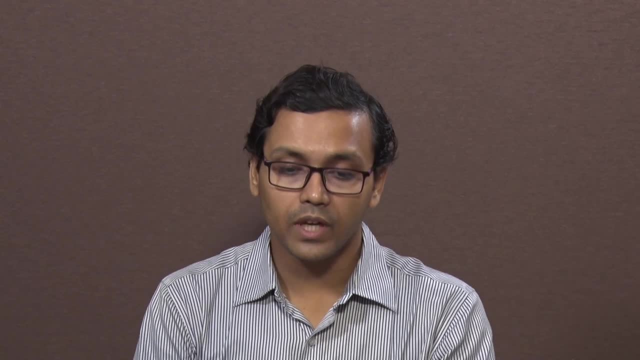 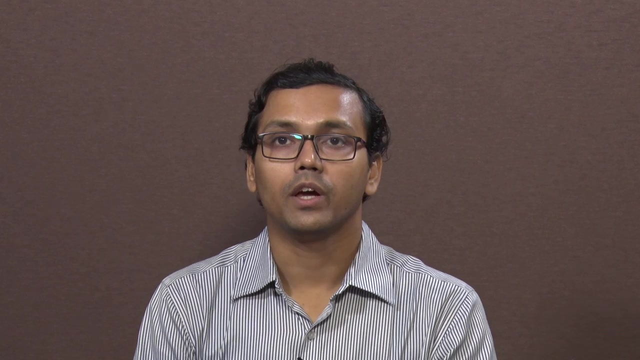 everywhere in the system, then there will be no heat transfer, because the primary consideration that we need to have heat transfer is the difference in temperature and therefore, if a system is in perfect thermodynamic equilibrium, or at least in thermal equilibrium, there will be no heat transfer at all. In order to have heat transfer, we first need to have 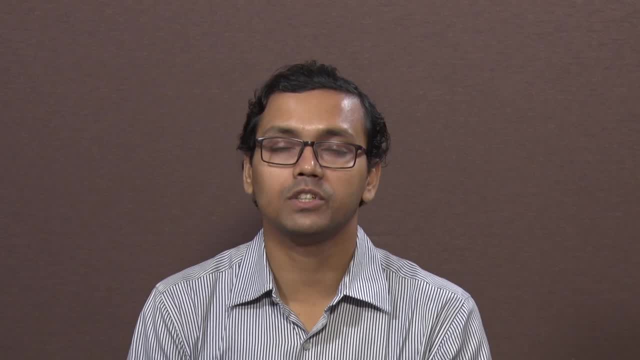 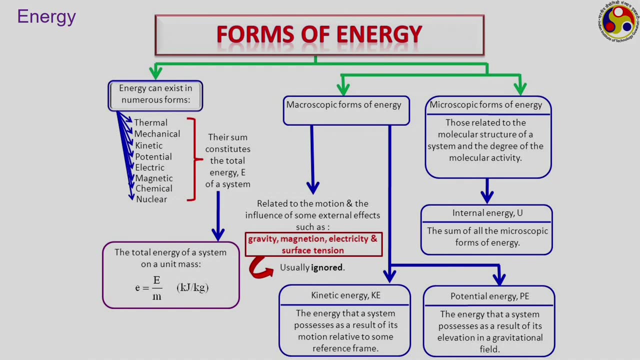 have a non-equilibrium and then only we can start discussing about heat transfer. Now the property energy which I was talking about can be classified following several types, Like one kind of classification can be just what we realize from our senses, like thermal energy, mechanical energy, kinetic potential, electric, magnetic, nuclear, chemical. 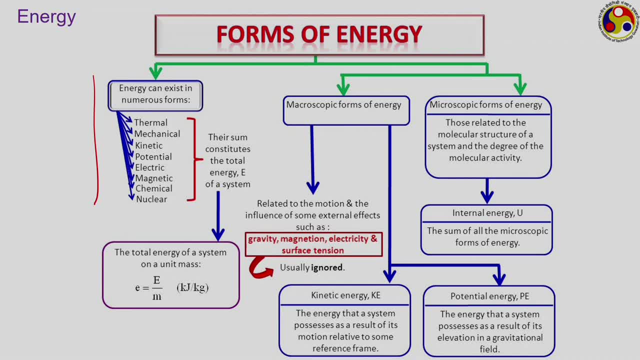 several types of energies. The total energy of a system is commonly given the symbol capital E, and small e is a specific energy which is an intensive property. But there is another kind of classification of the same energies, that is, macroscopic form and microscopic form of energies. The macroscopic form refers to the form of energy which are associated with. 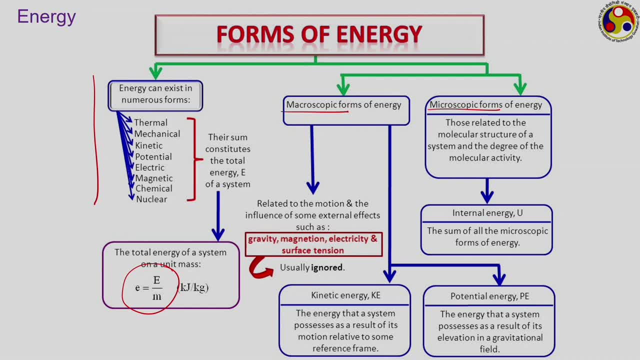 some external reference scale, like examples. So this again can be of two categories, One example, which are related to the motion and the influence of some external potential field, like gravitational field, magnetic field, electric field or surface tension. associated energies are associated with the. they are 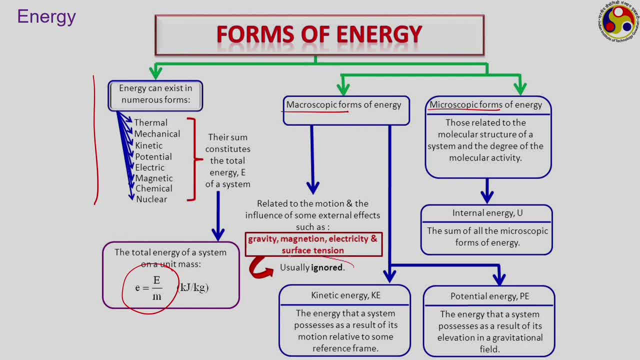 all macroscopic form of energy. Generally in analysis of thermodynamics they are ignored. only in certain special cases they may appear. But these macroscopic forms are associated with the presence of some external influencing field, like gravity being the most common one. So macroscopic form of energy is the kinetic and potential energies which are again associated. 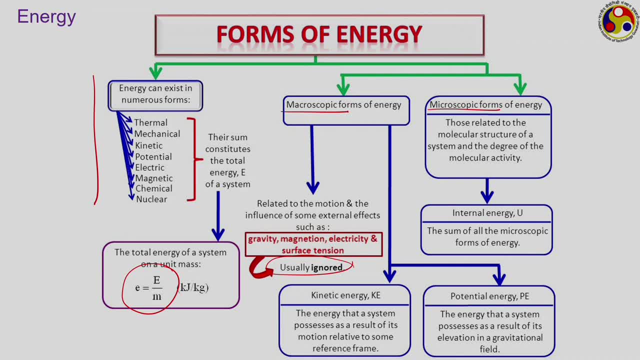 with the choice of some external length, scale or external reference system. Like kinetic, energy is measured in terms of the velocity of the system with respect to some external reference frame. Similarly, the potential energy is measured in terms of the elevation difference of the system with respect to some reference scale and the choice of reference. 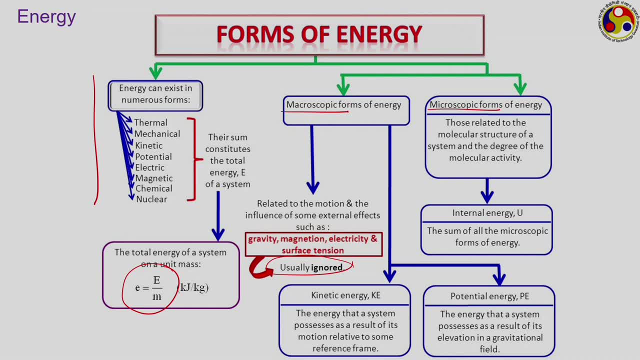 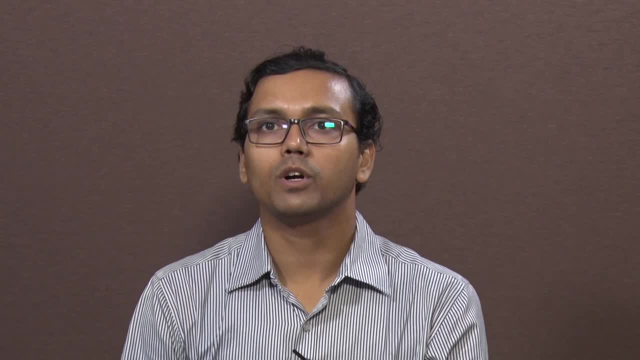 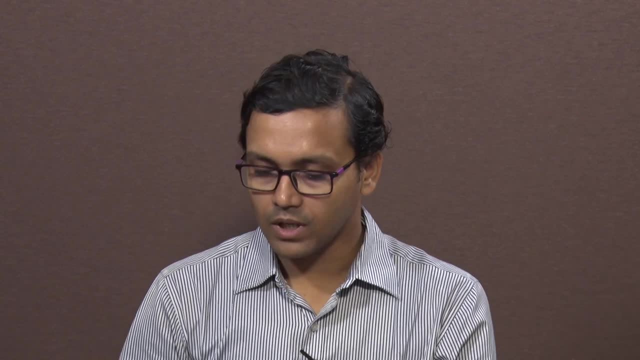 scale is always as per the convenience of the user, Like. suppose you are travelling in a train, so inside the train, if you start running from one side of the compartment to the other side, then how to measure the kinetic energy? One choice of reference frame can be the train itself, so your velocity then needs to be. 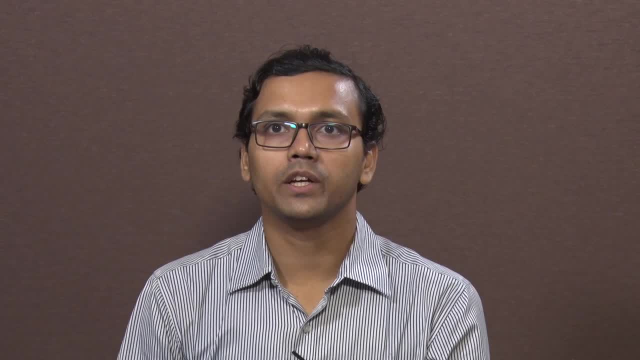 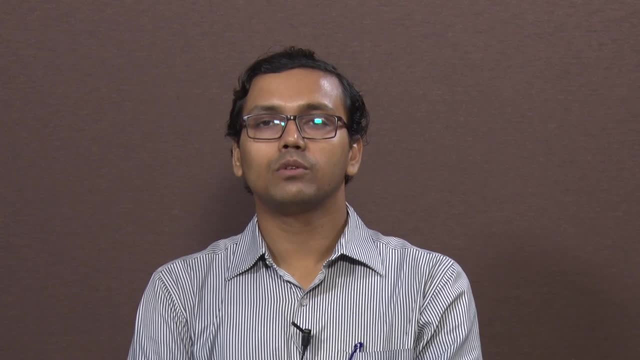 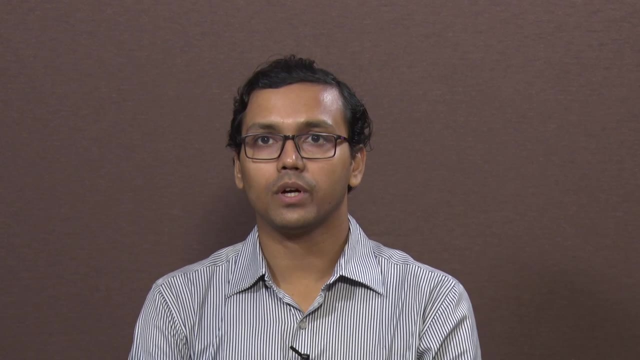 measured with respect to the velocity of the train and accordingly you can calculate kinetic energy. Another choice of reference frame can be the outside ground, which is stationary. then if you want to calculate the kinetic energy, then we need to take into account the velocity of the train and also your velocity with respect to the train into account. 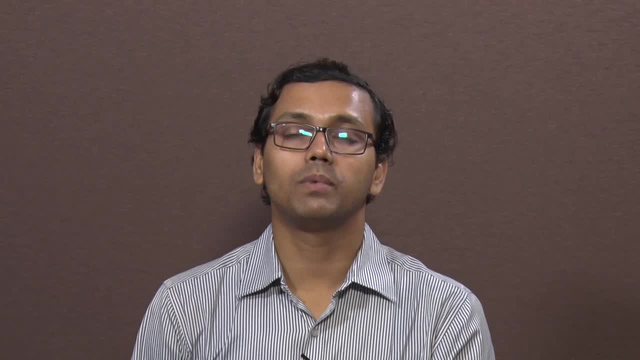 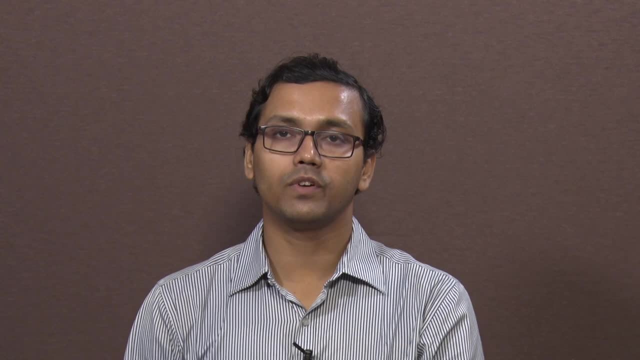 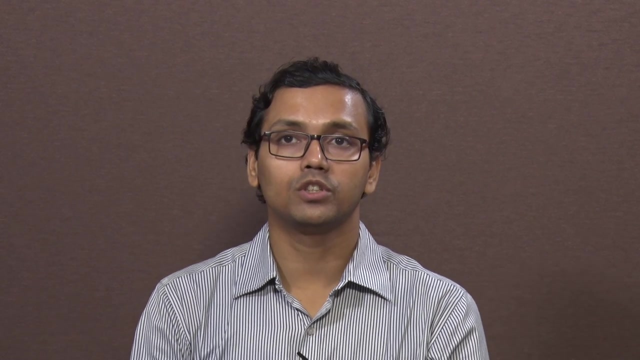 Another choice of reference frame can be may be some hypothetical frame which is placed outside the earth, because the earth itself is rotating. So if we want to calculate kinetic energy with respect to that particular reference frame, then the kinetic energy or the velocity of the earth also needs to be taken into account. This way the choice of reference frame can. 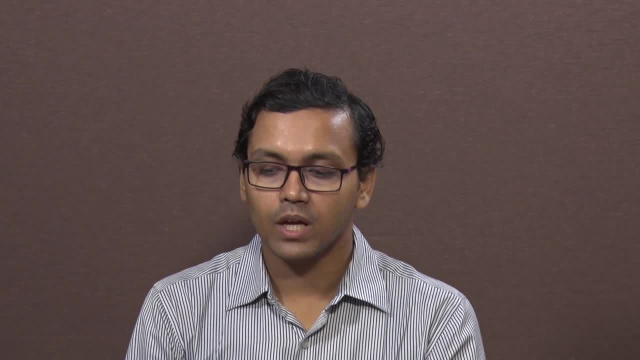 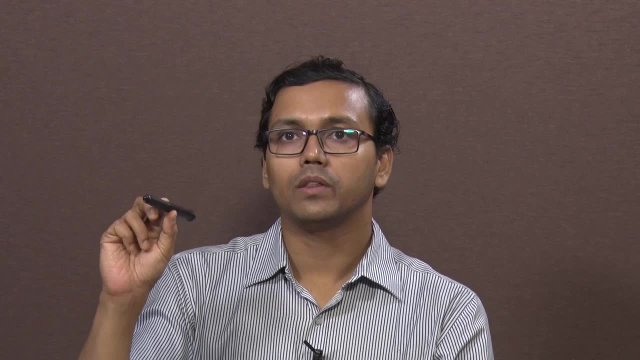 vary and accordingly the magnitude of the reference frame can be taken into account. The magnitude of kinetic energy can also vary. Same for potential energy, like if we want to calculate the potential energy, say, for this particular pen. now we have to choose some reference frame. What can be your choice of reference frame? One choice can be the. 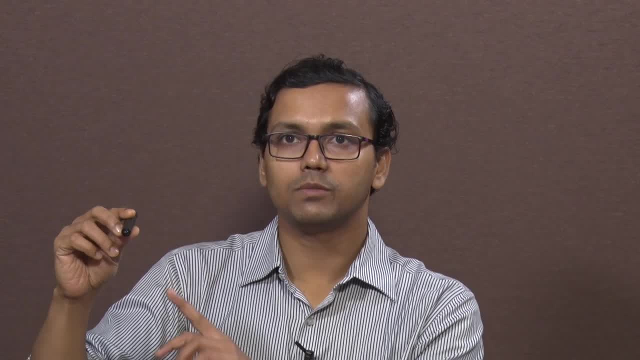 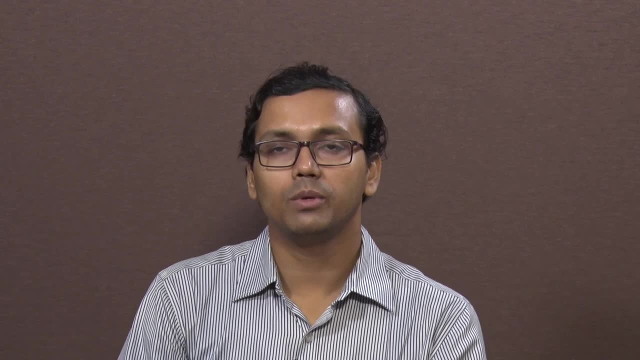 top of the table. then we just have to measure the elevation difference from this pen to the top of the table. But if we choose our reference frame as the floor of this studio, then the height will be larger. corresponding magnitude of potential energy also will be. 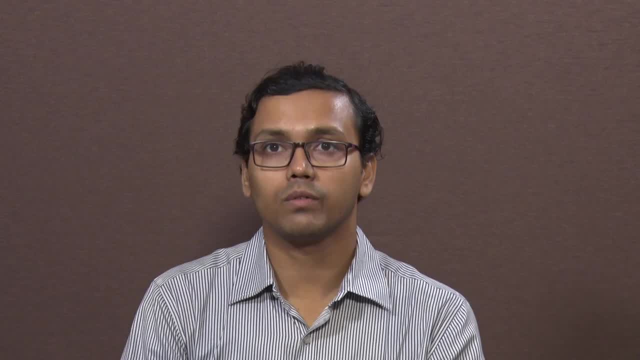 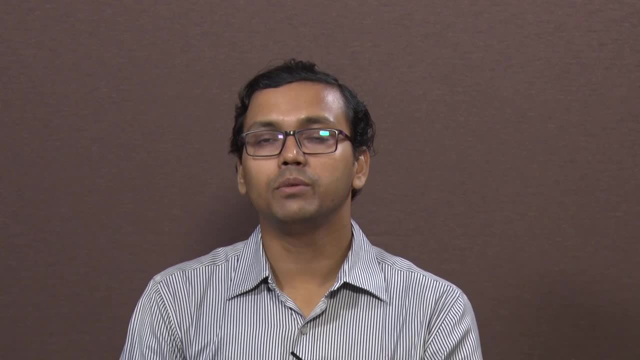 larger. So we are sitting in the studio which is on the third floor of our building. So if we choose the reference frame, which is connected to the ground floor, then there are 3 more floors or corresponding height. that needs to be taken into account. So accordingly, 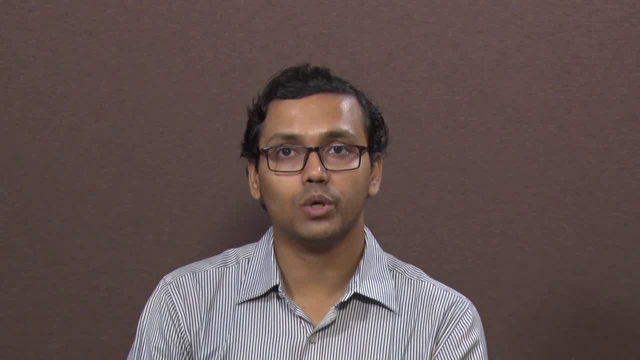 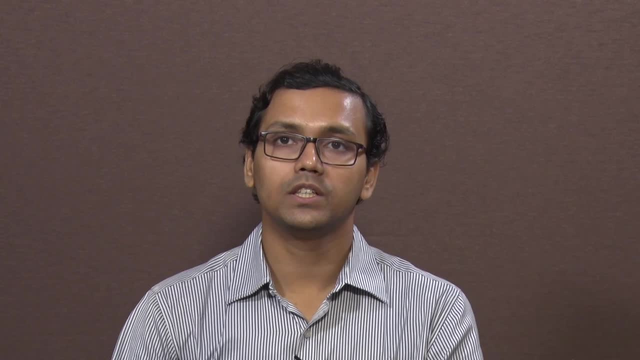 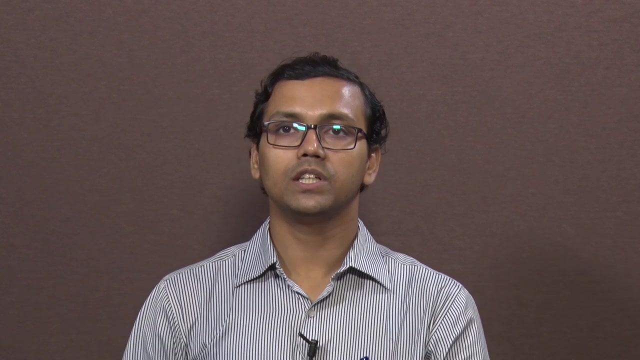 the magnitude of kinetic and potential energies can vary depending upon the choice of reference frame, But in thermodynamics generally we are always bothered about the change in the energy content of a system and accordingly we are always talking about the change in the kinetic energy and potential energy. and as long as we are doing this calculation, considering 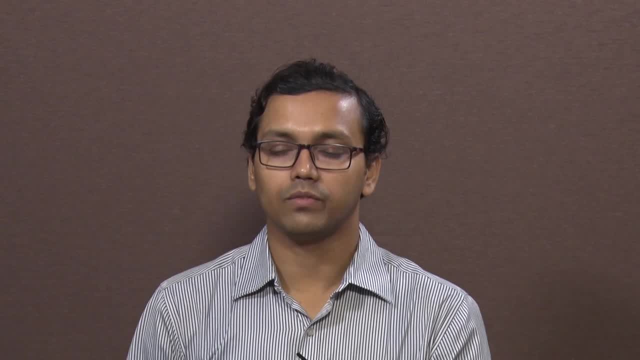 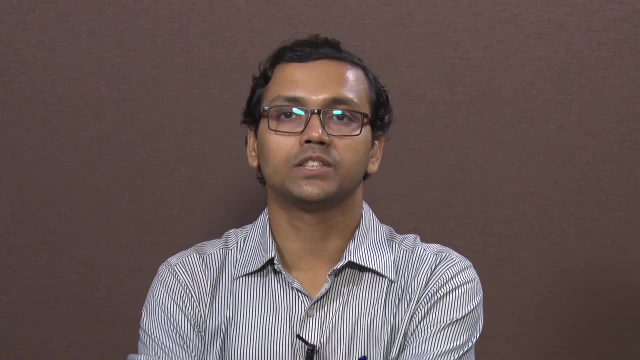 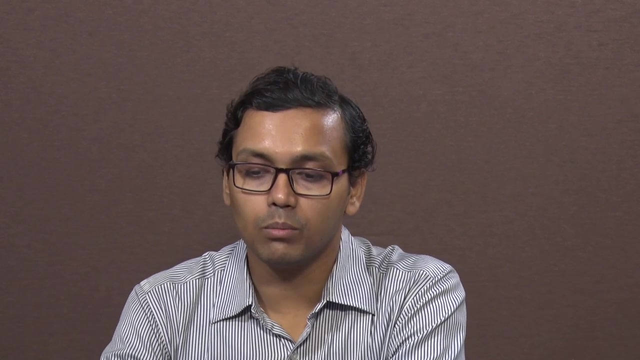 the same reference frame, then we do not need to bother about the reference frame itself. But these all are macroscopic forms because they all can be realized from our senses with respect to certain external reference frame or certain external influences. But there is a microscopic form as well which is associated with the molecular structure. 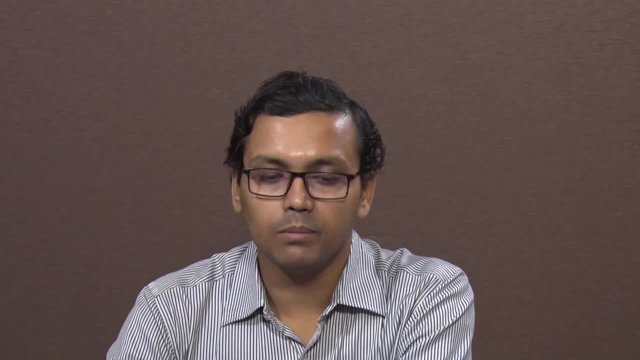 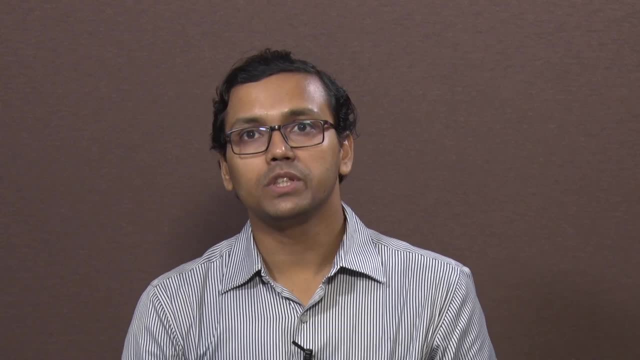 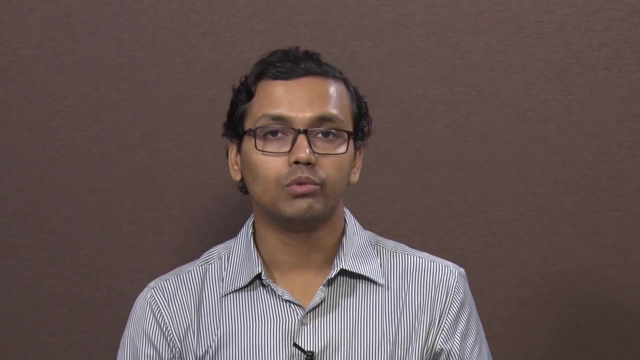 of the system and the degree of molecular activity. There can be several kinds of molecular activity. The molecules can have translational motion, rotational motion, vibrational motion. Also, we can have this molecular energy in the form of sensible and latent energy, where the latent energy is associated with the change of phase of a system and it is extremely difficult. 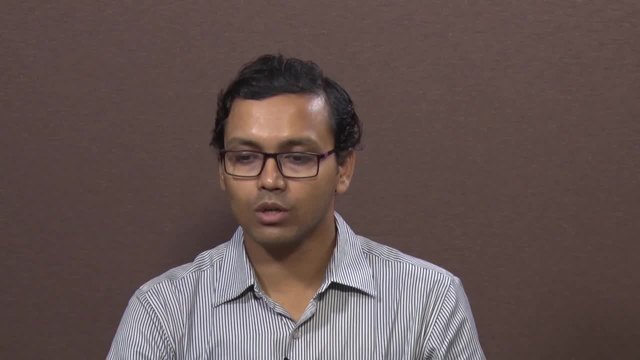 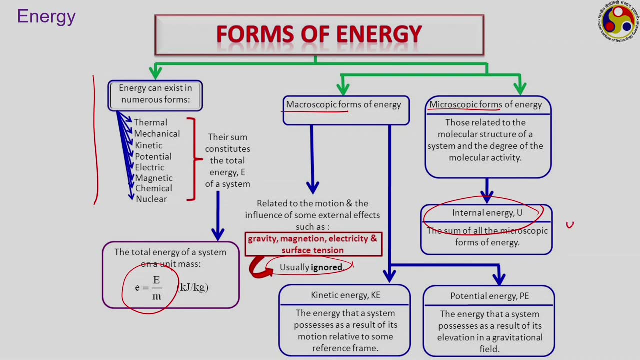 to get a perfect measure of all these individual components and therefore we club all of them into this term called internal energy, given the symbol capital U, The specific internal energy. Internal energy is denoted by small u, which is capital U divided by m. It is an intensive property, whereas total internal energy or just internal energy is. 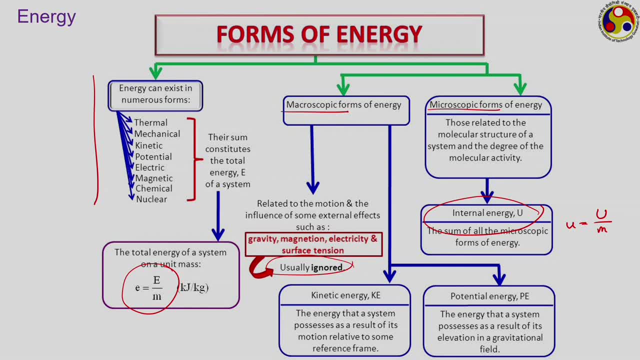 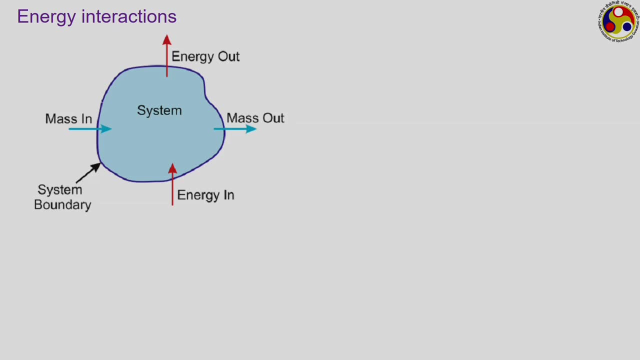 an extensive property. It is a sum of all the microscopic forms of energies. Again, perfect measure of the magnitude of internal energy is not possible, so we always get the measurement with respect to certain reference. and once we know about energy, then we need to talk about the energy interaction that a system can have with the surrounding. 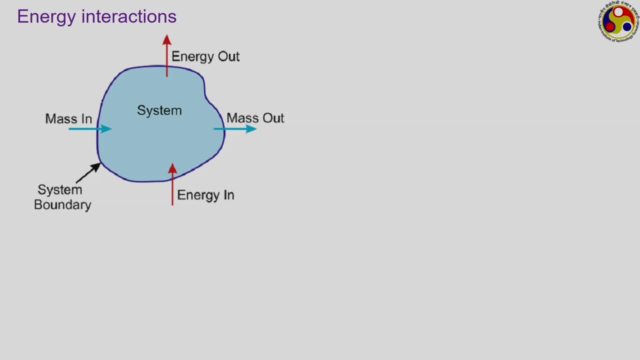 A system can have energy interaction with the surrounding across the boundary following three different ways. Generally, in thermodynamics, we are not bothered about the energy content of the system itself. rather, we are only concerned about the energy which is crossing the boundary of the system. That is why often, these energy interactions are also referred as energy in transition. 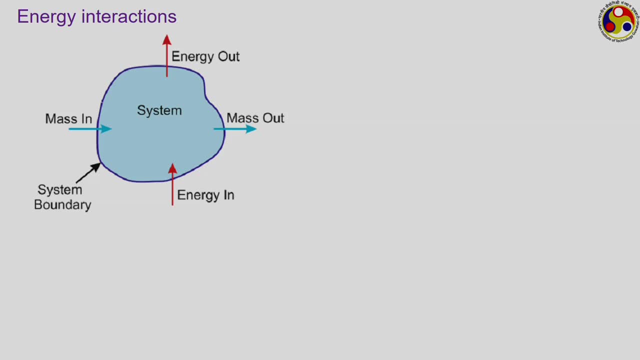 or as boundary phenomenon, whereas the energy content of the system itself is associated with the internal energy, Of course, for a stationary system only If the system itself is boundary. If the system itself is moving, then it can also have its own kinetic and potential energies. 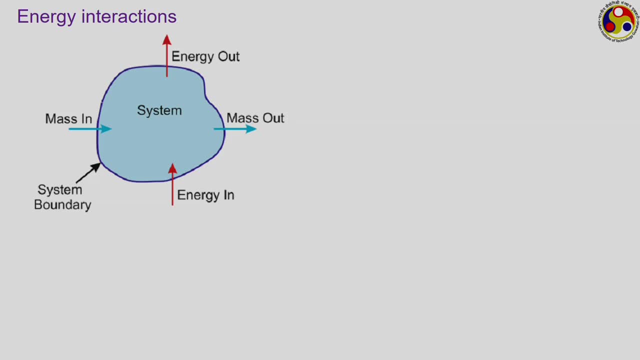 but in thermodynamics we are generally bothered only about the energies which cross the boundary of the system, or I should say they are realized at the boundary of the system. Then there can be three kinds of energy interaction. We can have heat transfer. Heat transfer refers to the energy interaction which is taking place because of a temperature. 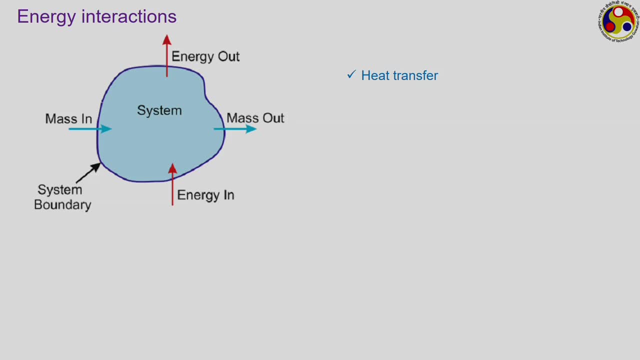 difference between system and surrounding or thermal non-equilibrium between the system and surrounding. Second is the work transfer. Work transfer refers to the energy interaction. Work transfer refers to the energy interaction between system and surrounding, which is not taking place because of any temperature difference, rather taking place because of some other. 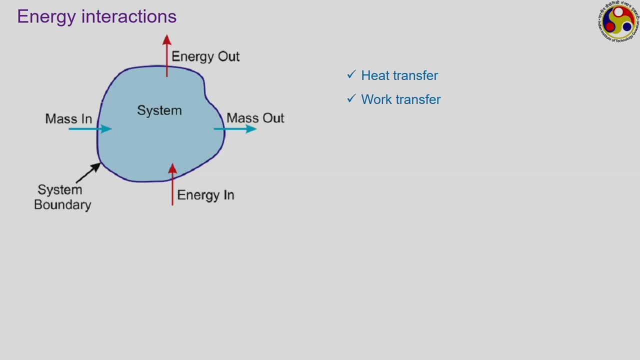 potential difference. The other potential difference can be a change in volume, can be gravitational energy or can be something else, but not temperature difference. So among all forms of energy interaction that a system can have with its surrounding, only the one that is happening because of temperature difference is classified under this: heat transfer. 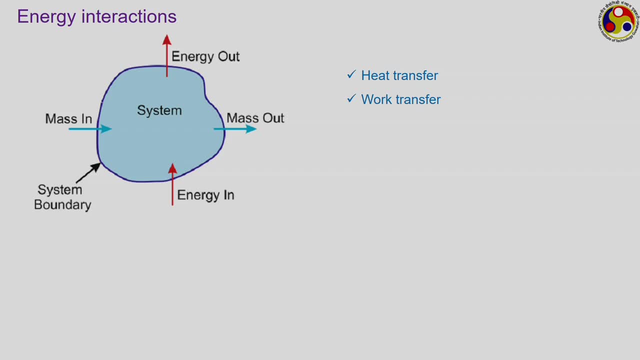 and everything else are classified, So these are clubbed into this work transfer. There is a third one also, which is the mass transfer, which is applicable- only one- for open systems, of course, because for closed system there is no mass transfer, But whenever mass flows into a system, it will also carry some energy with accordingly. 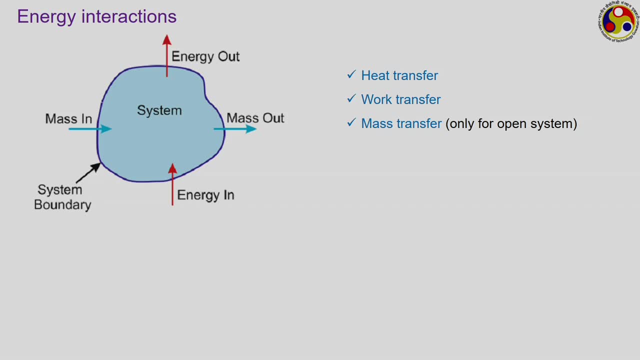 it will cause increase in the total energy content of the system. Similarly, when mass is leaving a system, crossing the boundary of the system and moving towards the surrounding, then it is taking some energy away from the system. So mass transfer is also associated with energy interaction. 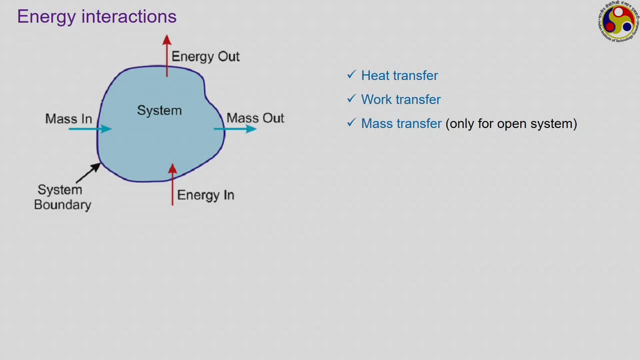 Outwardly you are. Wi будет Mon bary хот. the total energy transfer is on the high level And out of these 3, our interest in this course is in this heat transfer. So heat transfer is the energy interaction which is taking place because of the temperature. 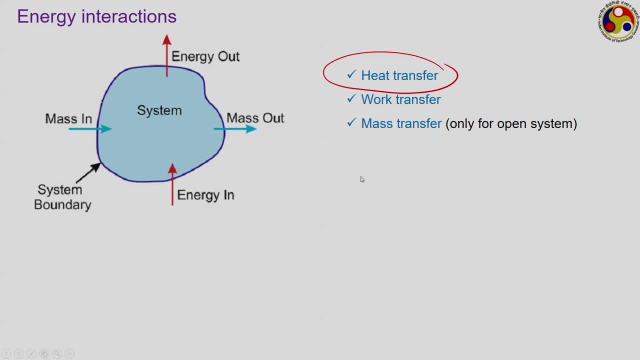 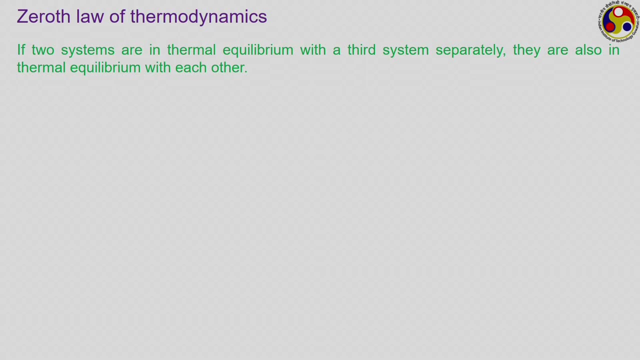 difference between system and surrounding. Now, before we define heat transfer into discuss very briefly about the laws of thermodynamics. You know, in conventional thermodynamics we study 3 laws. First is the zeroth law, which says that if 2 systems are in thermal equilibrium with 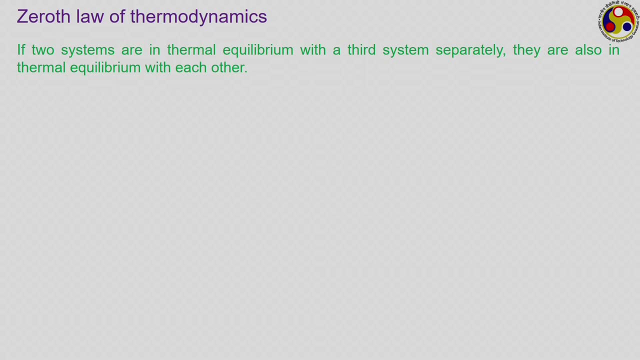 the third system separately. they are also in thermal equilibrium with each other, Like shown here. system A and system B are in thermal. system A and system C are in thermal equilibrium with each other and therefore system A and C are not having any heat transfer. 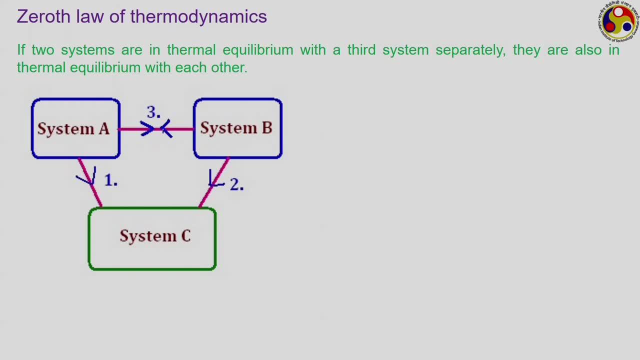 between them. Similarly, system B and system C are also in thermal equilibrium with each other and therefore they are also not having any heat transfer between them. Then system A and system B are also in thermal equilibrium with each other. and if we take system A and system B in contact with each other, 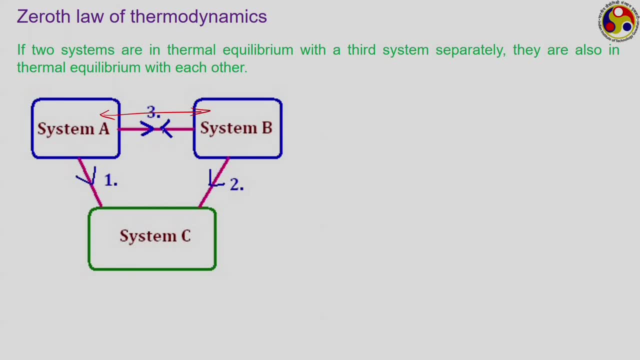 other, then they are not going to have any kind of heat transfer. That gives us two important concepts. one is that gives us the idea of measuring temperature using a thermometer. here I should mention that the term thermometer does not refer only to that mercury filled capillary tube that you use to measure body temperature, rather, 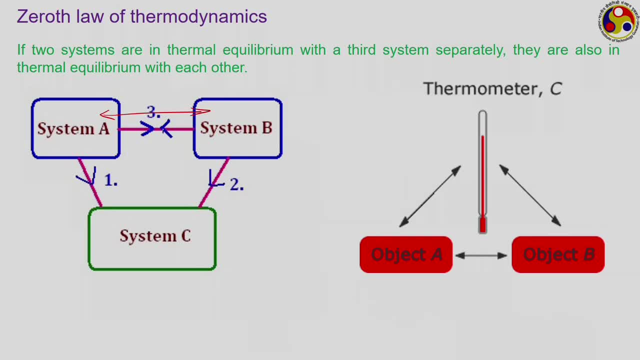 any temperature measuring device is a thermometer that one actually is a liquid in glass type of thermometer. So in a thermometer, the reading that we get by taking it in contact with our object A, which is the target, whatever reading we take, if we get the same reading when we 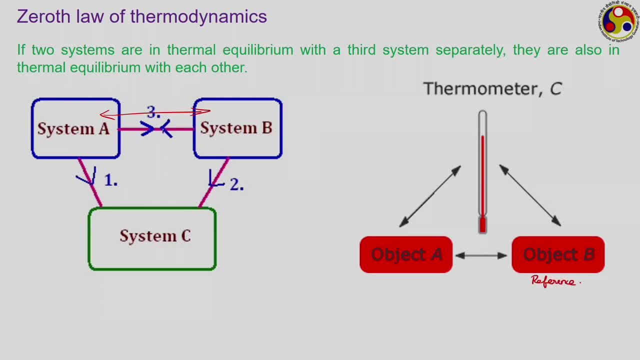 take this one into contact with some reference object with some known properties, then you should say that both object A and object B, that is the reference, are in thermal equilibrium with each other. So that is the first idea. The second idea is that we can measure temperature using a thermometer, So in a thermometer. 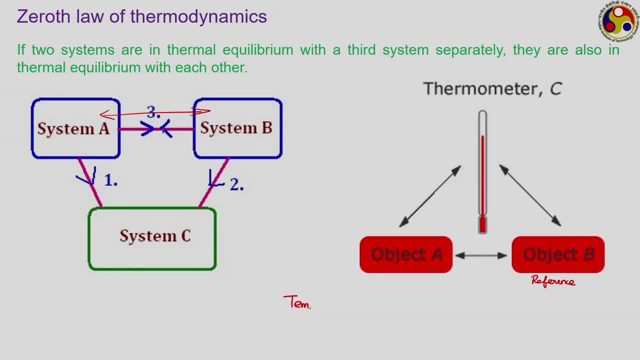 the second important concept that it gives is the concept of temperature. Temperature cannot be defined without the zeroth law of thermodynamics. we can only say that this one is hot, so it is at higher temperature. this one is cold, so it is at a low temperature. 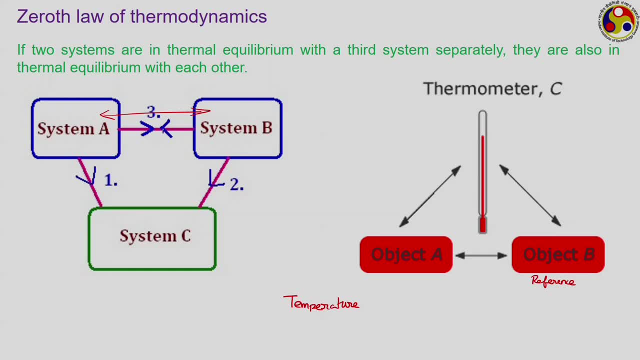 but that is only perception. But from zeroth law of thermodynamics we can say that temperature is the property which is essential to ensure the thermal equilibrium. or in other ways we can say that if suppose system A and system B are equal, If system b are in thermal equilibrium with each other, then the property that much be. 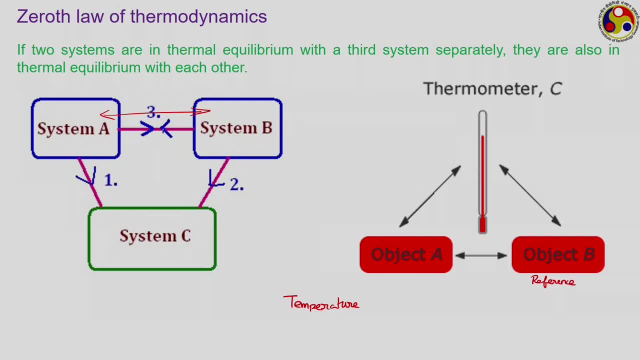 equal between them is temperature, Because the non equality of temperature is essential to have heat transfer and therefore only when the temperatures are different then the systems can be having heat transfer across them. So the concept of temperature comes from the zeroth law of thermodynamics. 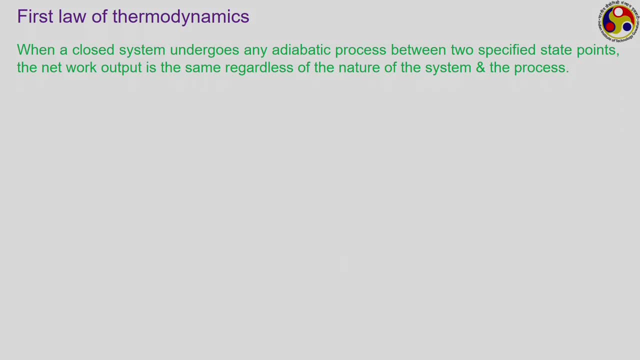 Next is the first law of thermodynamics, which gives us an idea about the energy interactions or the quantities, magnitude of energy interaction between a system and surrounding, When a closed system undergoes any adiabatic process between two specified state points. then the network output. 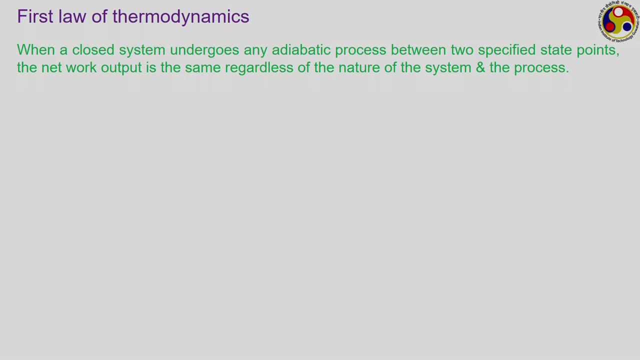 is the same, regardless of the nature of the system and the process. So if we identify a closed system like this, if it is undergoing any adiabatic process between two specified state points, like if we draw a diagram, let us say a PV diagram- 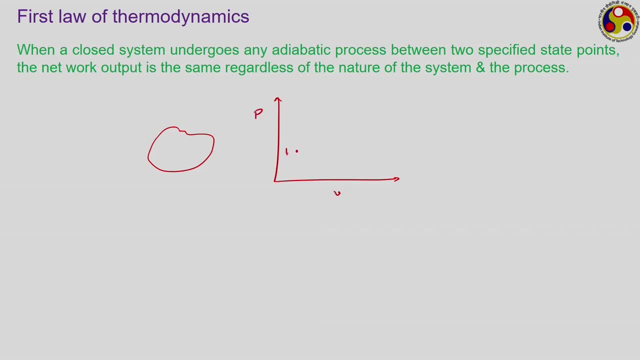 we are drawing. So this is the first state point, the initial state of the system. this is the final state of the system, that is, 2.. So system has gone through some adiabatic process between these two state points 1 to 2.. 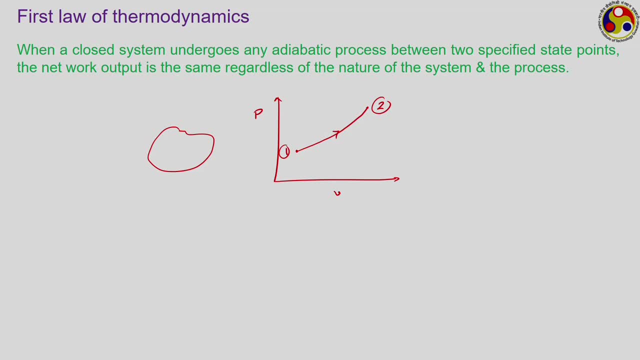 Then the first law of thermodynamics is saying that as long as this process is adiabatic- and we are fixing up these two endpoints- 1 and 2, then the network output will be always the same, regardless of the nature of the system and the process. That is because point 1 and 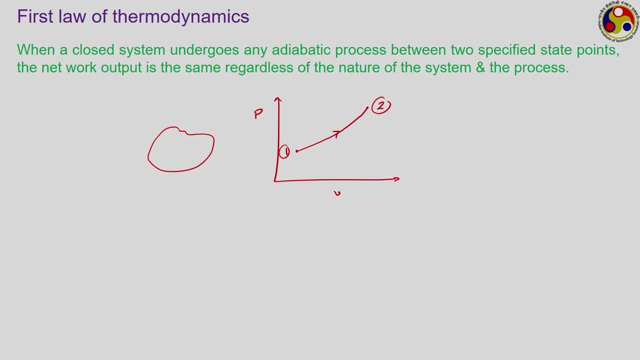 2 are two given state points, so they have fixed property values accordingly the adiabatic process. So the energy content of the system, the E1, and at state point 1, energy content of the system, that is E2, they are always same. So the change in the energy of the system E2-E1. 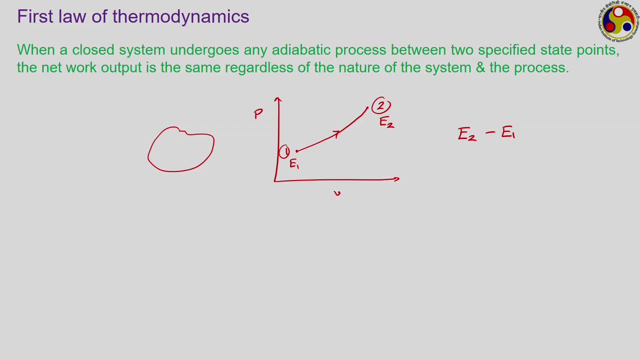 that is over this process will always be the same. that does not depend upon the nature of the line, whether we are following this line that is shown here, or a line something like this, or a process something like this, This change in energy content will always be equal, and from there we can derive that 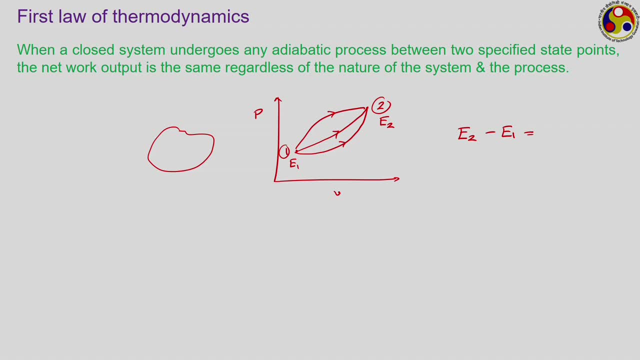 this is equal to the total energy content of the system. So this change in energy content is the energy interaction that has taken place, and for a closed system we can have only two kinds of energy interaction. One is the heat transfer that has taken place during. 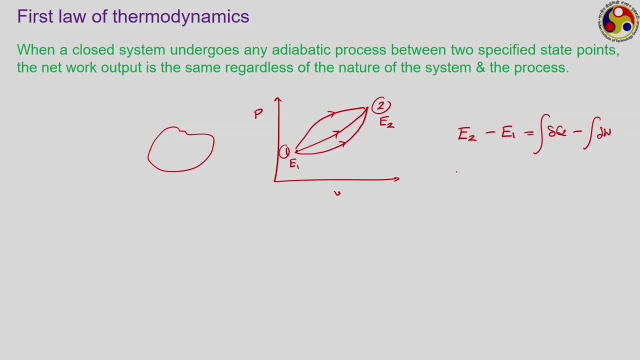 this process and other is the work transfer that has taken place. or if we write in differential form, we can write that dE is equal to del Q-del W. Here of course we are following the standard convention, that is, heat added to the system is positive and work done by. 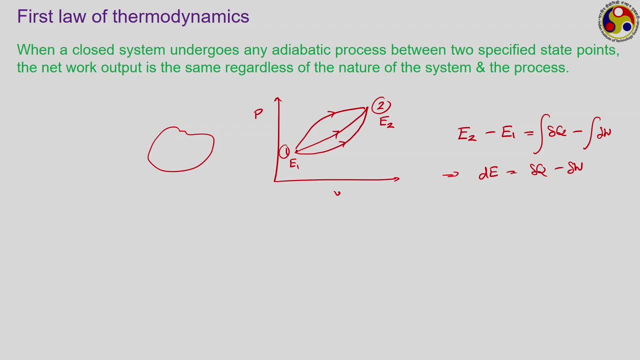 the system is positive. So the first law of thermodynamics: Thermodynamics gives us a way of measuring the magnitude of heat transfer. that is, from here we can write that del Q is equal to dE plus del W. So if we can measure the total, 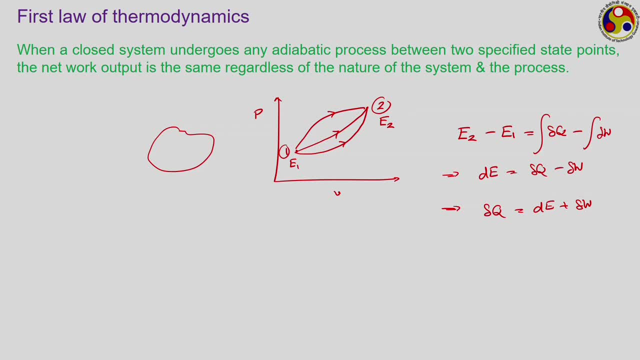 energy interaction, sorry, total work interaction, which is del W, and total change in the energy content of the system, then their combination is going to give you the total heat transfer. So, first law of thermodynamics: sorry. the zeroth law of thermodynamics gives us the 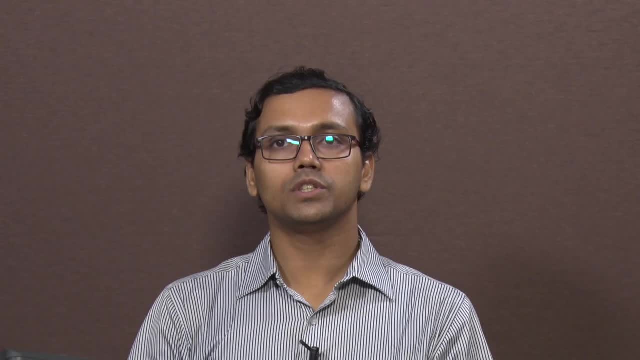 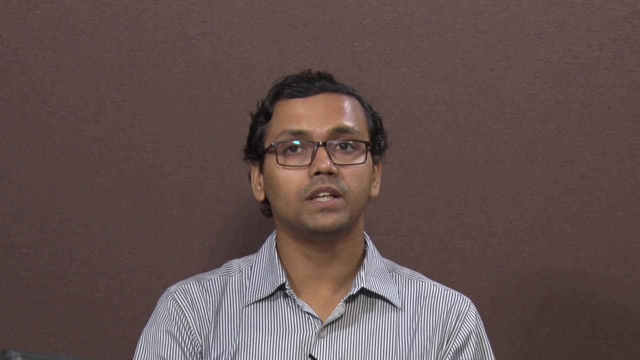 idea of temperature or concept of temperature? Who is going to give you the concept of temperature? Who will choose the property which determines whether heat transfer is possible or not? First, law of thermodynamics gives us a way of measuring the quantity of heat transfer. and then we 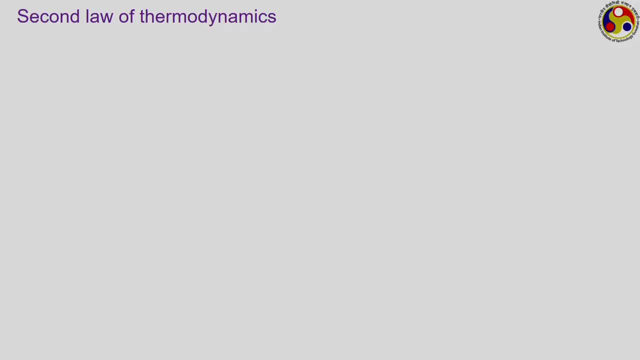 come to the second law of thermodynamics. Based on the first law, we can define different kind of systems. Now suppose if we define a system like this which is operating over a cycle- another important concept from the first law of thermodynamics. 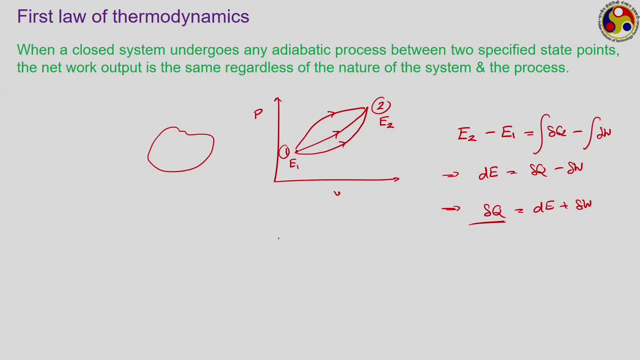 You must be knowing that the form that we have written that is for a cis individual process. So for an individual process we can always write: del Q minus del W is equal to dE. But if we are writing this over a cycle, then if we write cyclic integral of del Q, 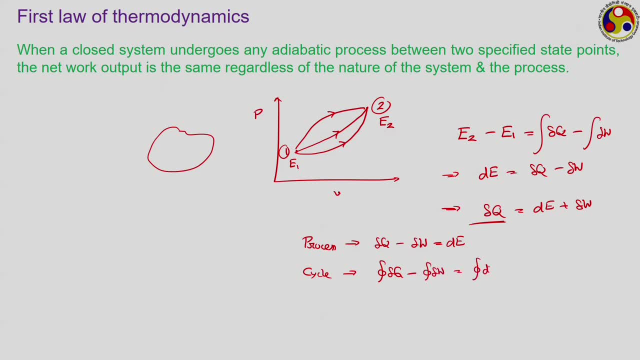 minus. cyclic integral of del W is equal to cyclic integral of dE. But cyclic integral of any property has to be equal to 0 because properties are state functions, So this is equal to 0.. Accordingly, over a cycle we get. cyclic integral of del Q is equal to: 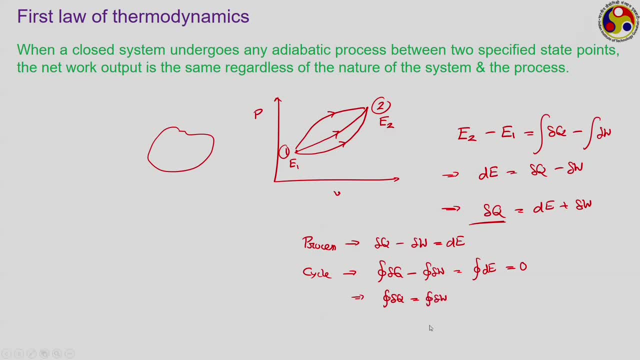 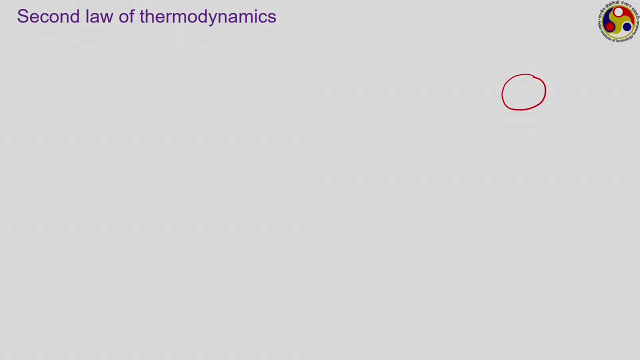 cyclic integral of del W. So over a cycle the total heat interaction has to be equal to total work interaction. Now let us talk about a process where we are supplying, say, Q, 1 amount of heat and this system is converting this entire to W amount of water. This entire process is a. 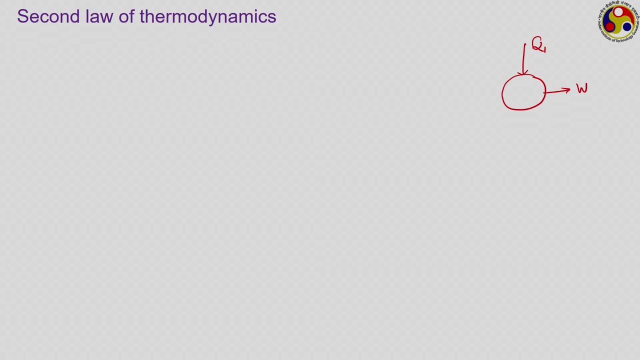 work. So here this is operating over a cycle. So here total cyclic integral of del Q is equal to Q1, cyclic integral of del W is equal to W, and as long as we are having Q1 equal to W, this is perfectly, is. it is not at all violating the first law of thermodynamics. 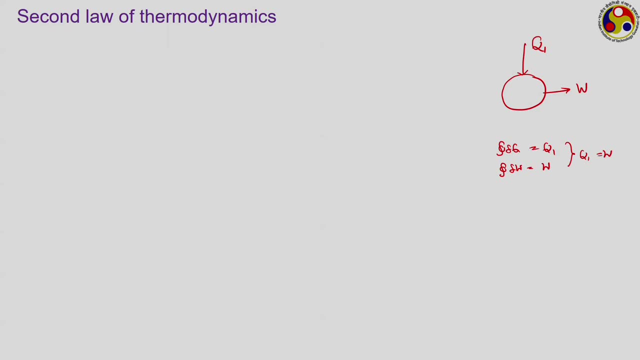 but any effort to create such a system always leads to failure, because this thing is not possible as per the second law of thermodynamics. There are two popular statements of the second law of thermodynamics, and the first one is associated with the scenario like this, which is the Kelvin-Planck statement. It says that 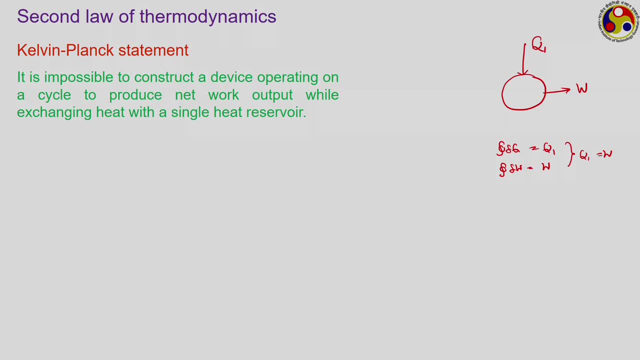 it is impossible to construct a device operating on a cycle to produce net work output while exchanging heat with a single heat reservoir Means the amount of heat it is receiving. only a part of that can be converted to work and rest, say, Q2 amount has to be rejected to the 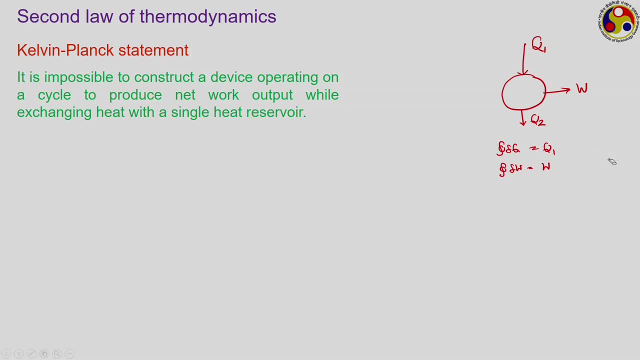 surrounding. Then in that case Total heat interaction is Q1-Q2, total work interaction remains W, and now we have Q1-Q2 is equal to W. this is definitely possible. So the second law of thermodynamics gives us an idea about the conversion of heat to work, at least the Kelvin-Planck statement. 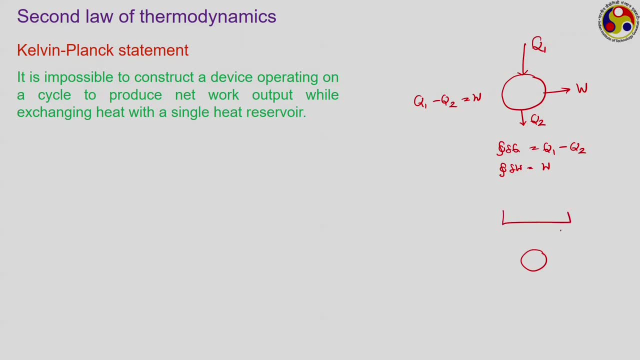 Let us consider another scenario. we have two bodies. one is at low temperature- T L, other is at a high temperature- T L. One is at low temperature- T L- and other is at high temperature- T H. Here T H is higher than T L. The system is drawing Q1 amount of heat. 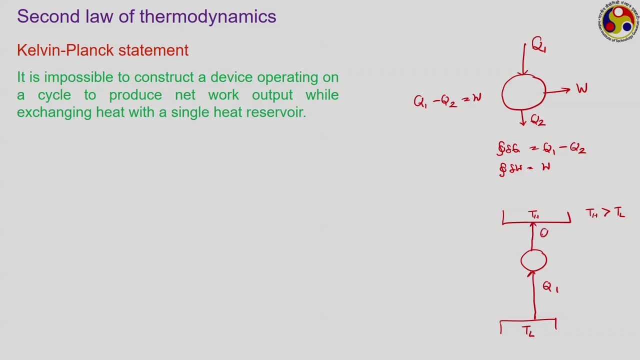 from this low temperature body and transferring the entire quantity to the high temperature body. So here they are. at the moment, total work interaction is 0,. total heat interaction- how we can write? System is receiving Q1, rejecting Q1, so that is equal to 0,. so the 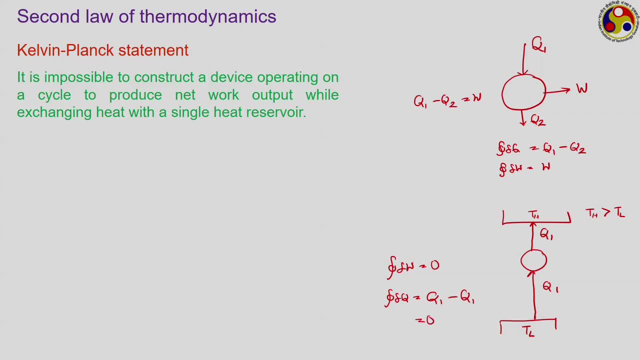 first law is definitely satisfied. But again, such kind of process is not possible. So the second law is not possible according to the Clausius statement of thermodynamics, which says that it is impossible to construct a device operating on a cycle to produce no effect other than transferring heat from a low temperature reservoir to a high temperature. 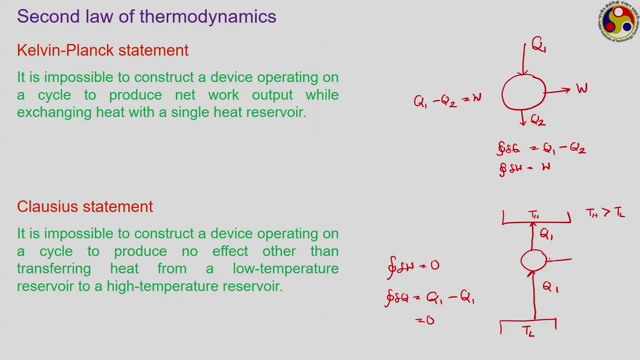 reservoir. That means to make this process done we have to give some work input to the system and accordingly Q2 amount of heat will be added to the high temperature body. In that case total work interaction is equal to minus W and total heat interaction is equal. 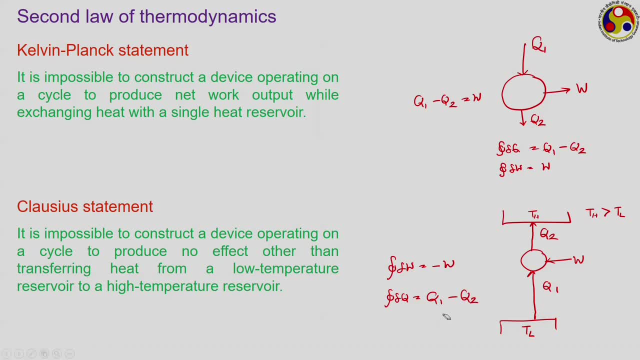 to Q1 minus Q2. and now, applying first law, we have Q1 minus Q2 is equal to minus W or Q2 is equal to Q1 plus W. now it is possible. So the second law of thermodynamics actually giving us the direction of heat transfer. So the zeroth law gives us the concept of 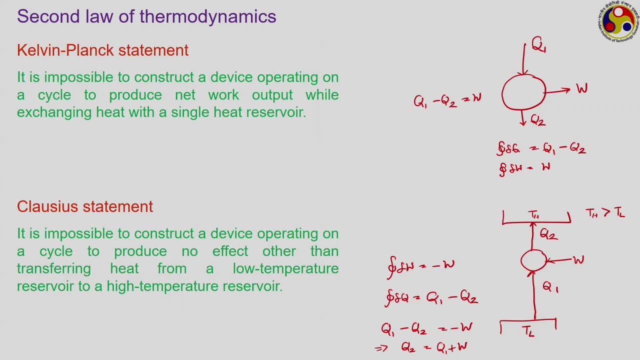 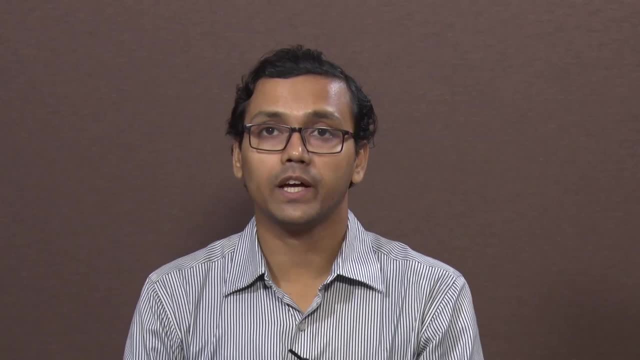 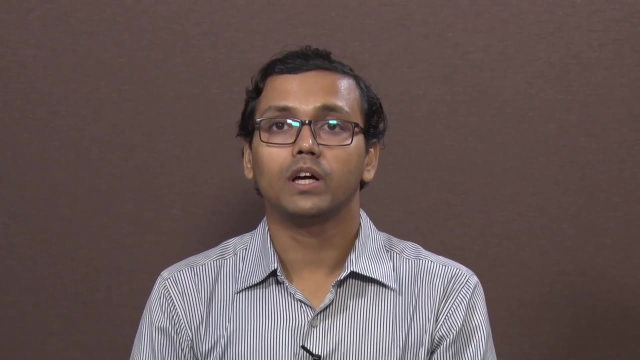 the property temperature which dominates the heat transfer. first law gives us a way of measuring the quantity of heat transfer, and second law tells us about the possible direction, or realistic direction, of heat transfer, But none of them are giving us any idea about the nature of the heat transfer itself or the modes of heat transfer. and that is precisely. 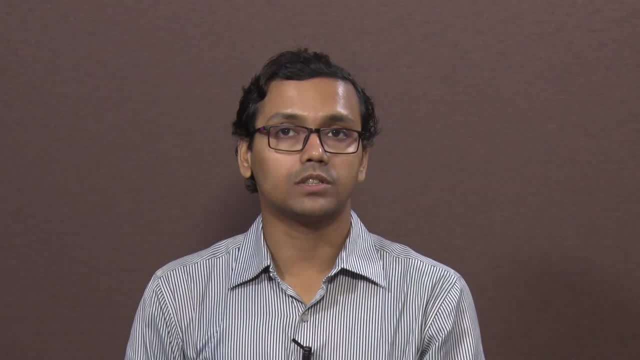 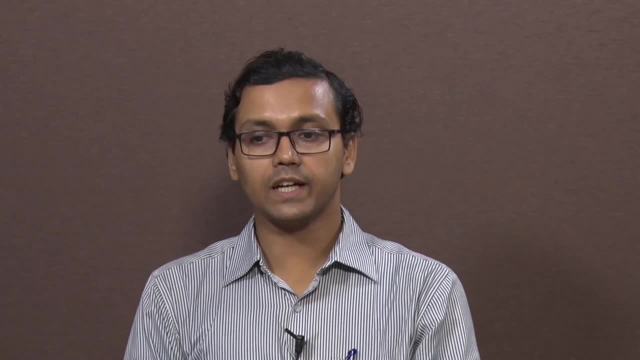 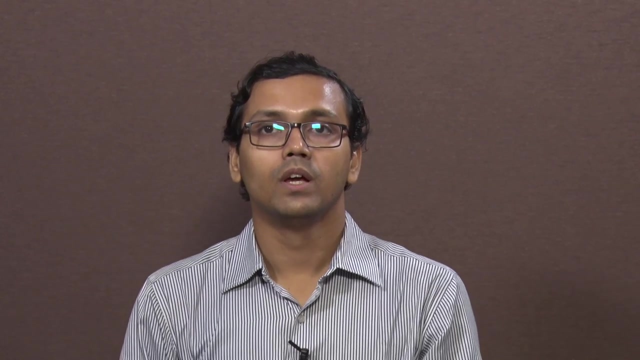 where the subject of heat transfer starts. Thermodynamics is never bothered about the nature of heat transfer or the nature of exact nature of interaction between system and surrounding it, just It takes the quantity heat as a gross or as a whole. It is in the subject of heat transfer. 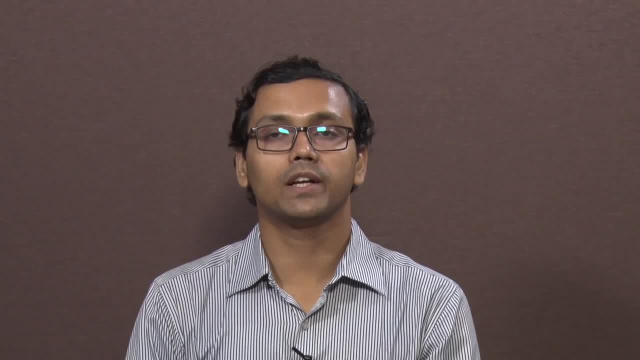 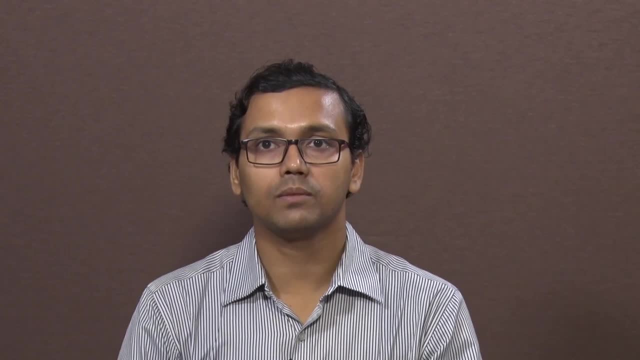 when you study exactly what is the mode of heat transfer? what are the factors that can contribute to this? what are the ways we can control the amount of heat transfer and also the rate of heat transfer? Like in thermodynamics, we can get the idea that Q amount of heat. 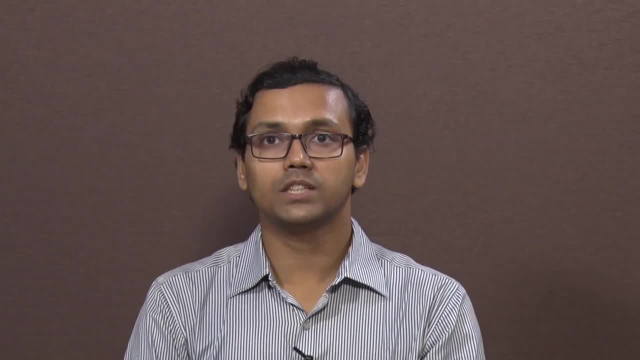 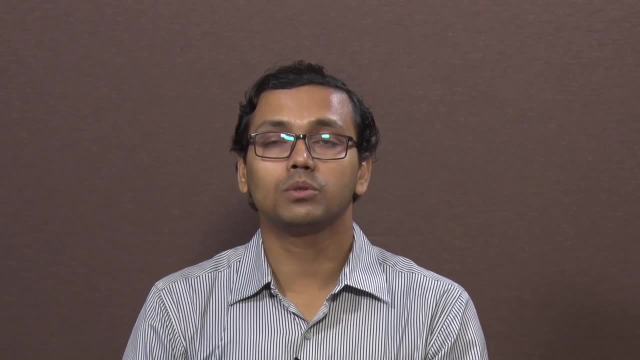 has been transferred from the system to the surrounding, but how much time it has taken place, over which it has taken place, or how much time is required? what is the rate of this heat transfer? None of this questions can be answered by thermodynamics and therefore. 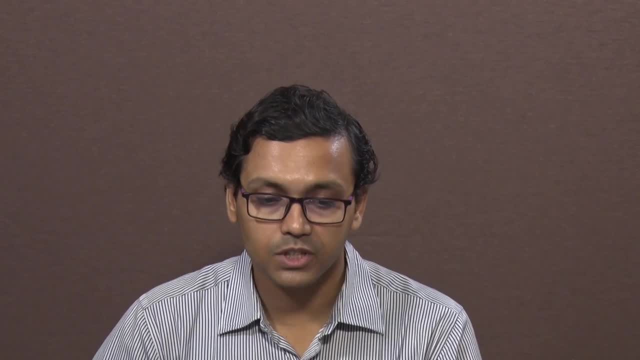 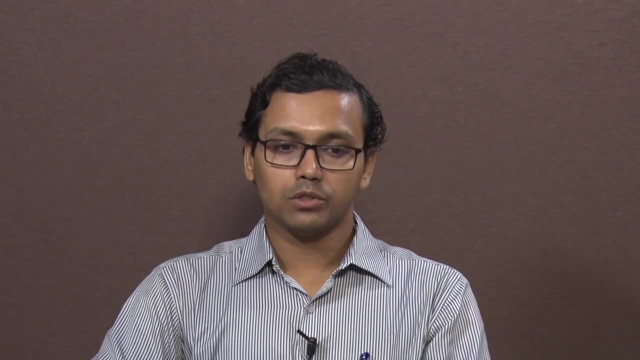 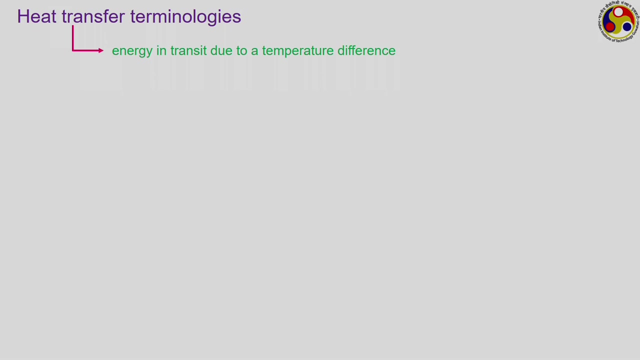 we need to study heat transfer precisely, from precisely, to know the answer to these questions. So some terminologies with which I would like to start the discussion of heat transfer we know from the knowledge of thermodynamics: is heat transfer? is the energy in transit due to the temperature difference? 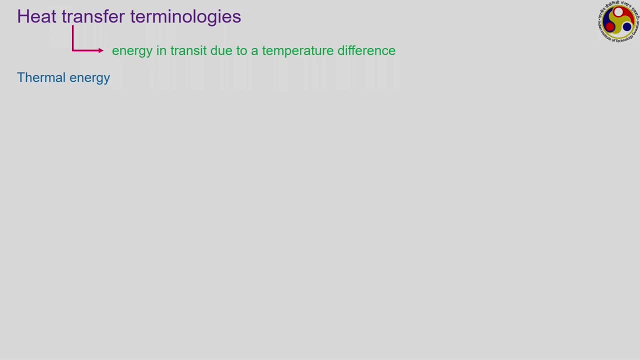 Now, the first term we shall be talking about is thermal energy. Thermal energy is just, in thermodynamics sense, that Q or del Q that I have just used, is the total amount of energy that has moved from system to surrounding or from surrounding to system because of some temperature difference. 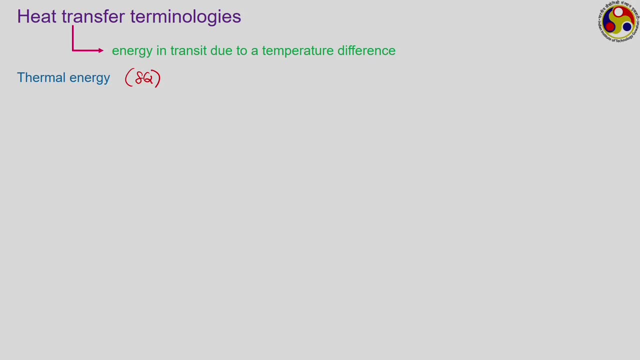 between system and surrounding. So del Q or Q is the symbol that will be used, and it is energy. only so corresponding SI unit can be joule. The next is temperature. the symbol T will be used. SI unit is Kelvin, but quite often 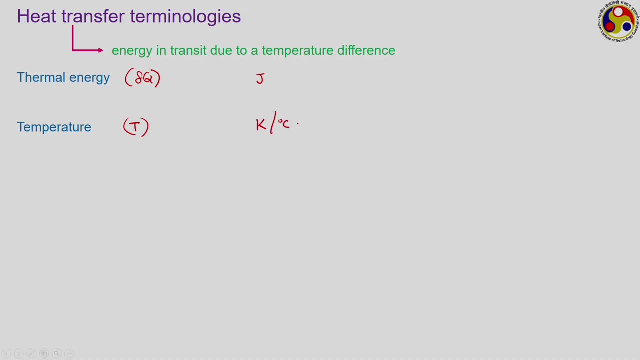 we may be using units like degree Celsius. similarly, with joule, we may have to move to units like kilo joule or mega joule. So temperature is again a thermodynamic property which gives us an idea about the total energy content of the system, or at least the level of molecular. 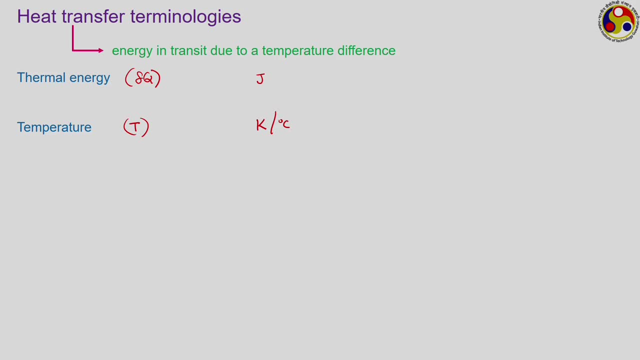 activity and also when we are talking about energy interaction between two systems, then the magnitude of temperature. So that decides the direction of heat transfer. Now comes the heat transfer which I was talking about. Heat transfer is again the energy in transit because of a temperature difference. 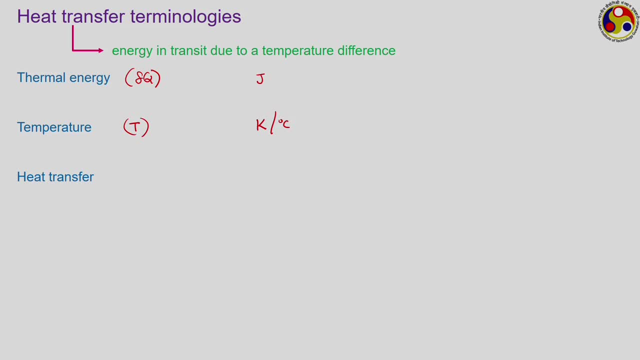 is nothing but the thermal energy. but the difference is that in heat transfer we are specifically talking about this del Q, whereas here the term thermal energy can refer to anything. it can refer to the total energy content of the system as well. Then let us use the symbol capital. 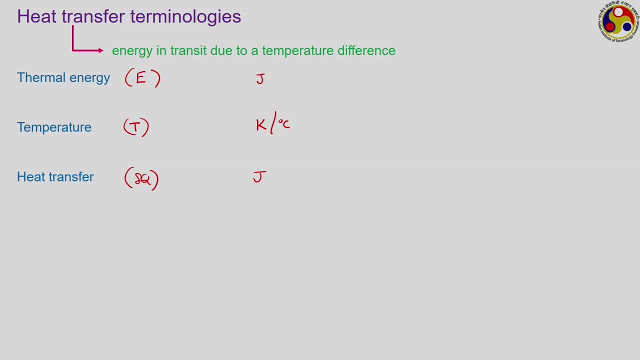 Capital E to denote the energy or the thermal energy which can primarily be associated with the total energy content of the system, whereas we are going to use this symbol Q or del Q to designate heat transfer. Then now these 3 quantities you have identified in thermodynamics: 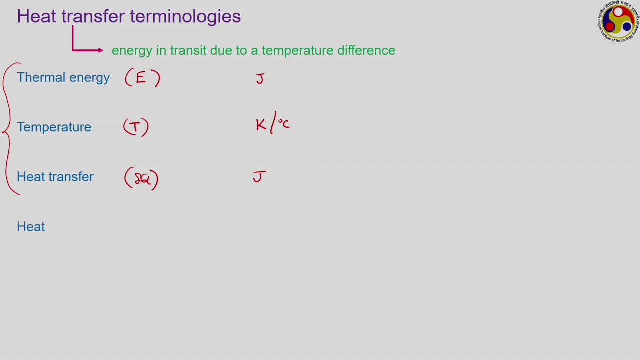 as well, but not this one, which is heat. Heat refers to the total quantity of energy that has been supplied over a period of time. Now, heat transfer, or rate of heat transfer, is a term which gives us an idea about the total energy interaction, but heat is the term that. 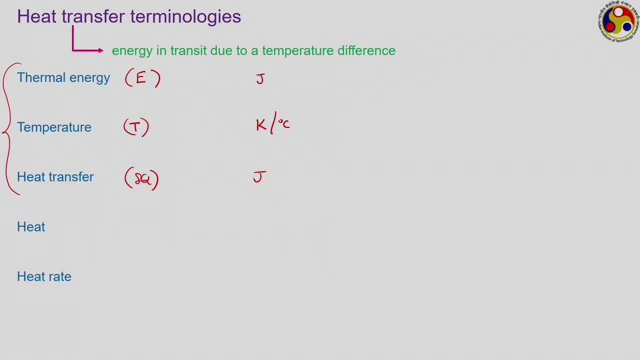 is primarily being used only in context with heat transfer. Heat rate exclusively used in case of heat transfer. it is- you can say it is, del, Q, dot. generally the dot symbol indicates the rate. unit can be watt. It is the rate of heat transfer. 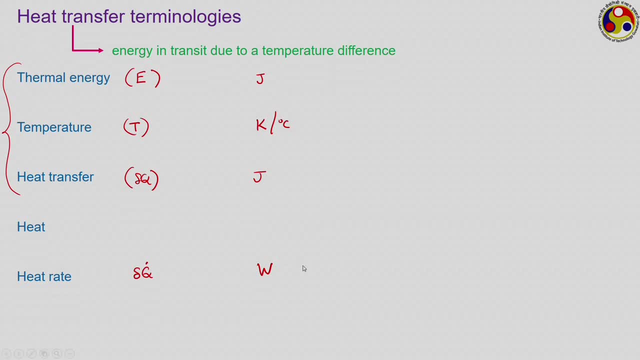 or heat transfer per unit time, And similarly another very common term, that is heat flux. Heat flux refers to rate of heat transfer per unit area. So quite often we use the symbol del, Q, dot and these 2 primes, This prime here, the dot. 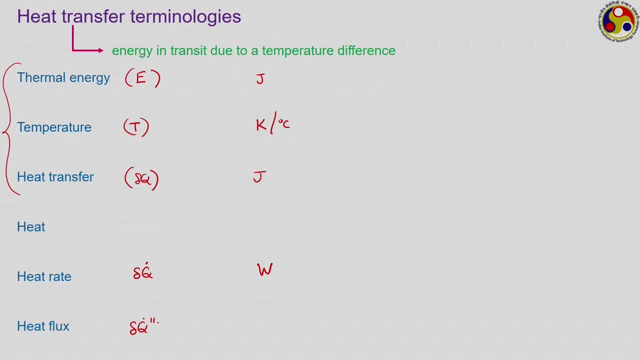 represents per unit time and these 2 small lines that I have drawn, the primes, each of them designates per unit length, So 2 lines designates per unit length. square or per unit area, So it is watt per meter square is the basic SI unit for heat flux. 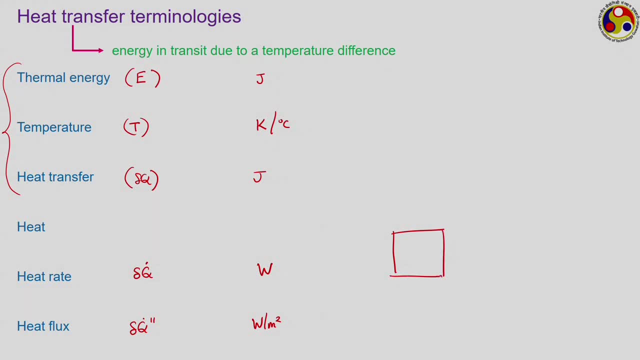 So like if we are talking about this is one area over which heat is transfer is taking place, then the total amount of energy that has left the system. if that energy is del Q, then del Q divided by the area of this one is going to give you the heat transfer. 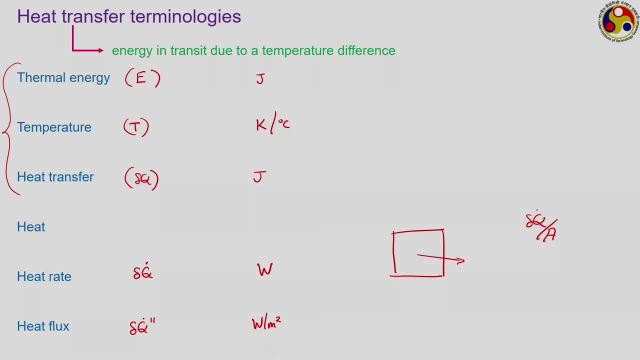 per unit area. and once you are talking about, once you are dividing this one by the time associated with this entire energy transaction, then we get this heat flux which you shall be using del, Q, dot, double prime. Sometimes the dot we can ignore also because in heat transfer we are primarily concerned. 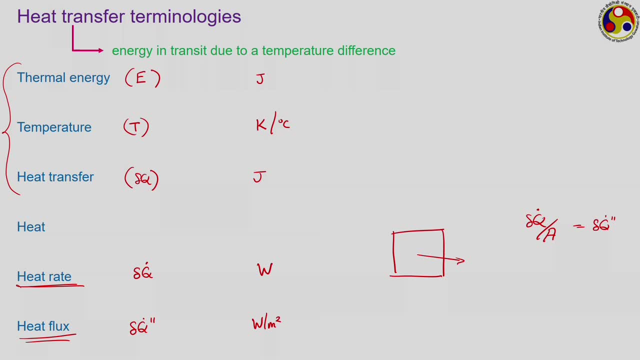 about the terms like rate or flux, which are always designated as per unit time. but this double prime is very important because we shall frequently be using per unit length or per unit area or maybe per unit volume. accordingly, we may have to use 1,, 2 or 3 lines. 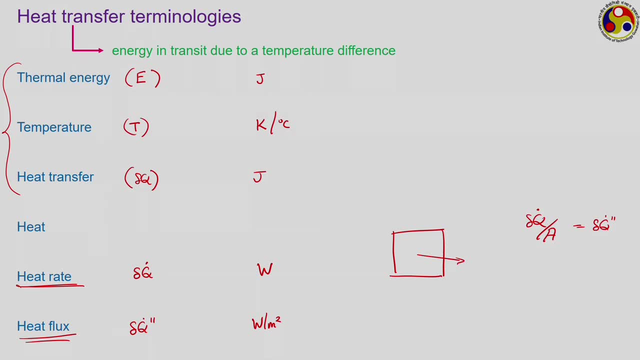 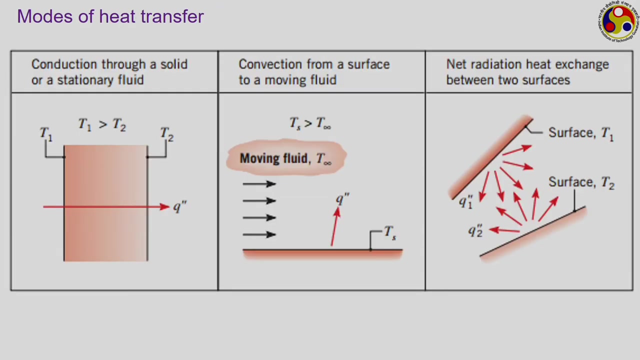 and if there are no lines that talks about the heat rate only. So the terms like heat transfer or thermal energy we are not going to use anymore. we shall primarily be using heat or heat rate or heat flux. Now, from your school level knowledge, you know that there are primarily 3 modes of heat transfer. 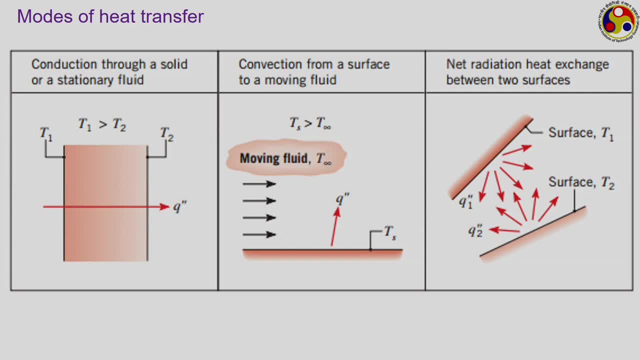 conduction, convection and radiation. or, as the conventional scientist suggested, there are only 2 fundamental modes: conduction and radiation, because convection is only a combination of conduction and advection or flow. In fact, the term convection, convection comes from there. only Convection is often referred as conduction plus advection. 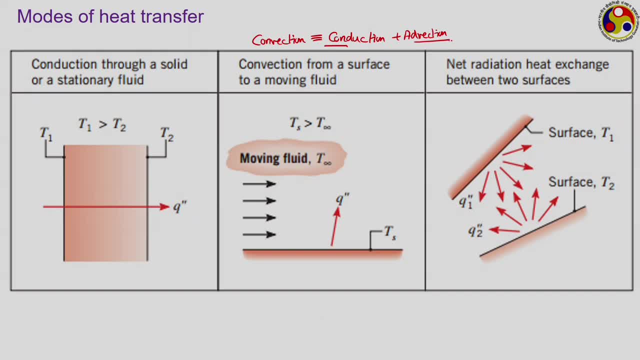 So take Con from there and vection from there. that gives us convection. Now, conduction is associated with the energy transfer because of the temperature imbalance from one part of the system to the other part. Any solid, liquid or gaseous substance can participate. 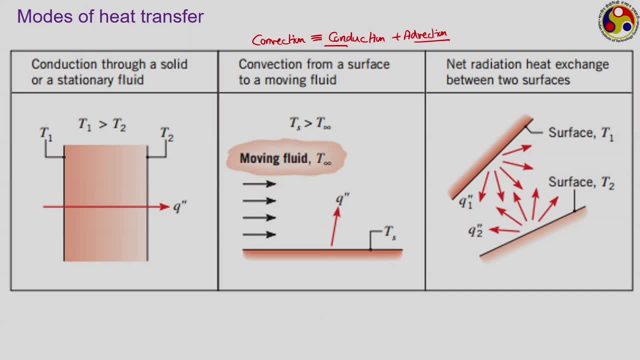 in conduction, heat transfer, though it is mentioned here as only solid or stationary fluid, but conduction is a fundamental phenomenon and any system can participate in this. It may be more pronounced in case of solids and very insignificant in case of gaseous, but conduction 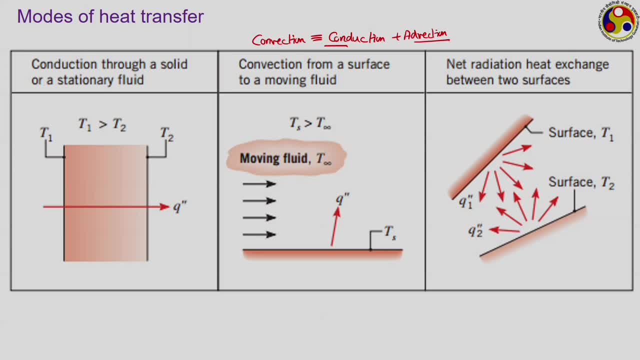 is always there. Whenever we have temperature gradient across a particular system or across the same substance- solid, fluid or gaseous- Then there will always be conduction, Whereas radiation is the heat exchange between two surfaces in the mode of electromagnetic waves, and it can happen at the absence of any intermediate. 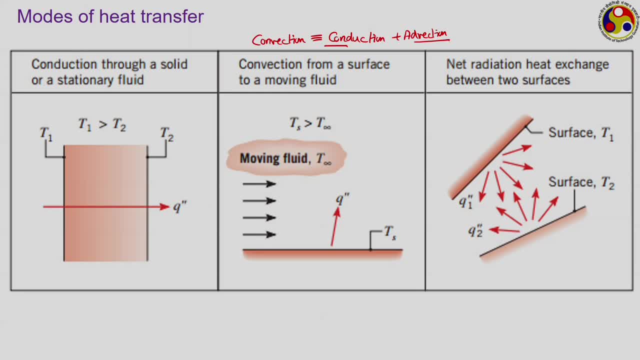 medium as well, But convection is primarily associated with the interface of a solid and a fluid. Whenever a fluid is flowing over a solid surface, it can take away some energy of the solid surface by virtue of its flow And accordingly it can be converted to a 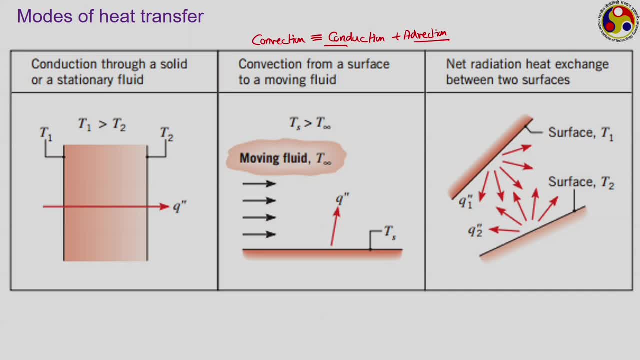 solid. So that is the main point, So that is the main point, So that is the main point. So finally, we get the convective mode of heat transfer. You can realise this. there are several ways you can realise this. Let us say, I have this particular file with me. 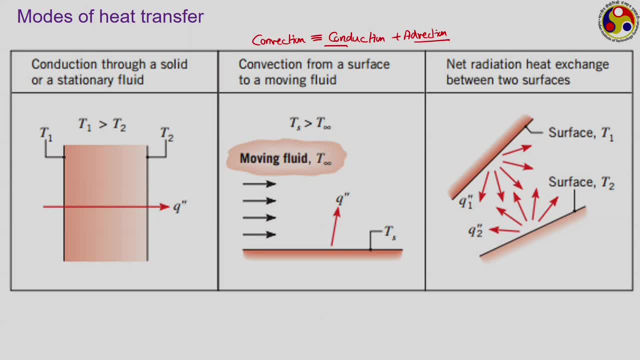 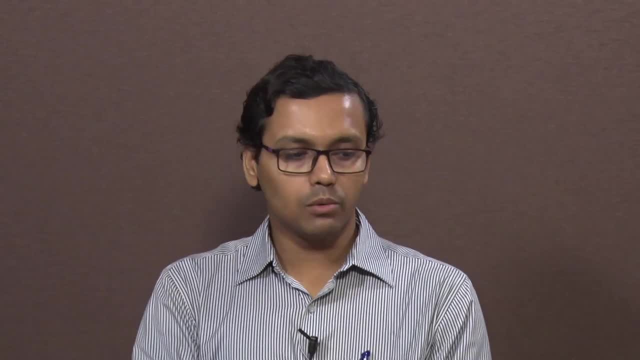 and I am standing in front of a big class. There are 50 students sitting in chairs in front of me. Now I want to transfer this particular file to the last student sitting at the edge. So from here we get a convective mode of heat transfer. Now let us do one. 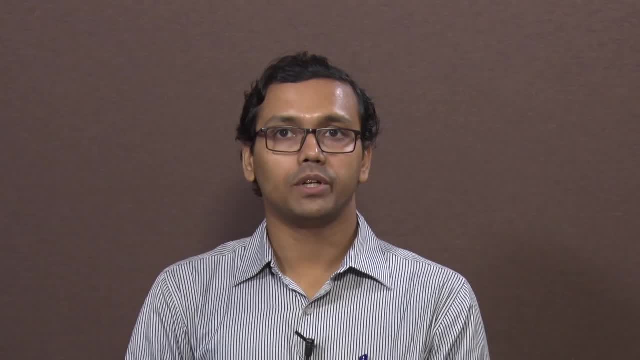 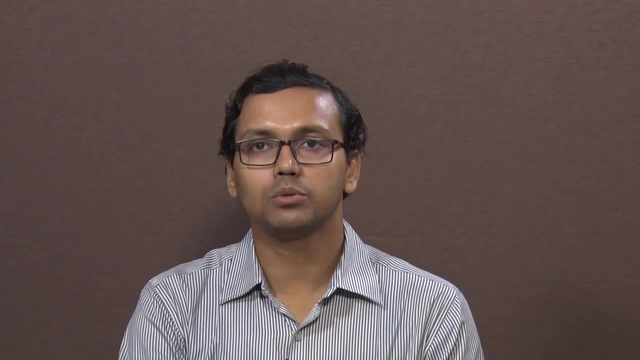 end or sitting at the back. Then there are 3 ways I can do it. one is I can give the file to the first student sitting in the front row. he will pass it over to the second student. he will pass it over to. 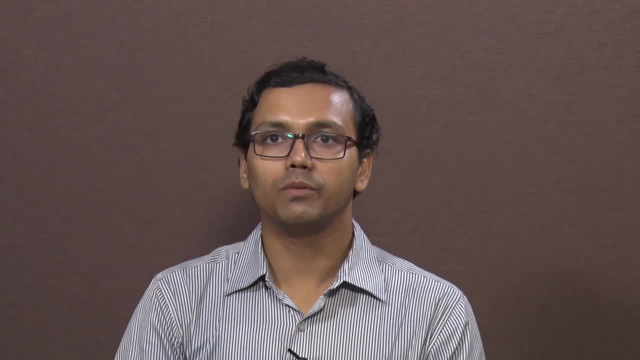 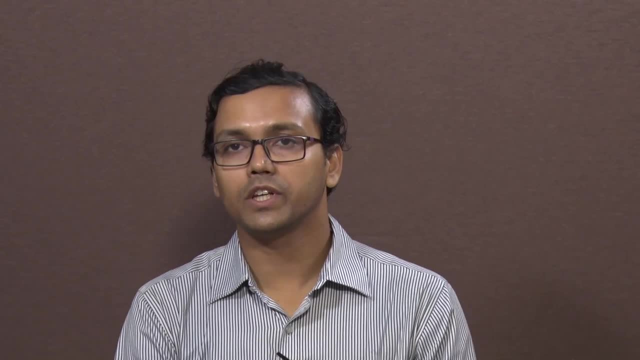 the third student and this way it will pass to all the 50 students to reach the last student. This is how conduction happens: energy is transmitted from one molecule to the next one, to the next one, to the next one, till the smallest energy level or lowest energy level. 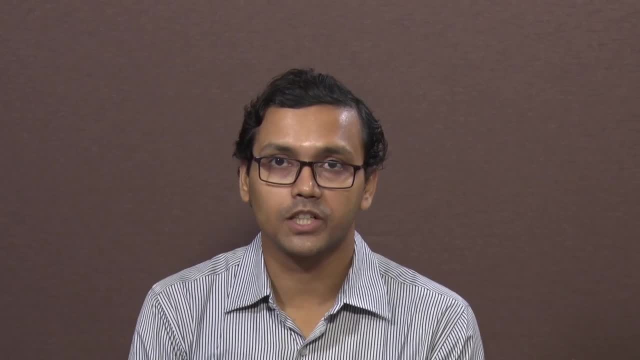 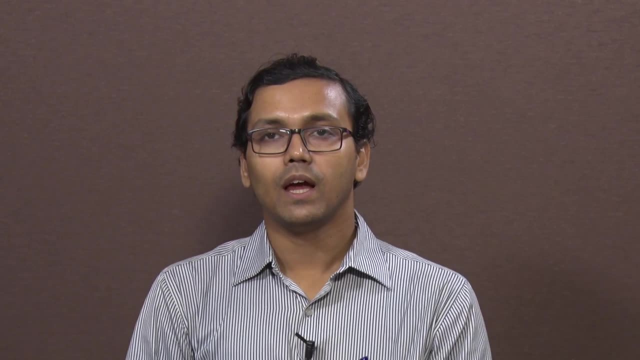 from the starting from the highest energy level. this is conduction. Second case is convection. convection always starts with the conduction, so it is something like I hand over the file to the first student, so that is a kind of conduction. 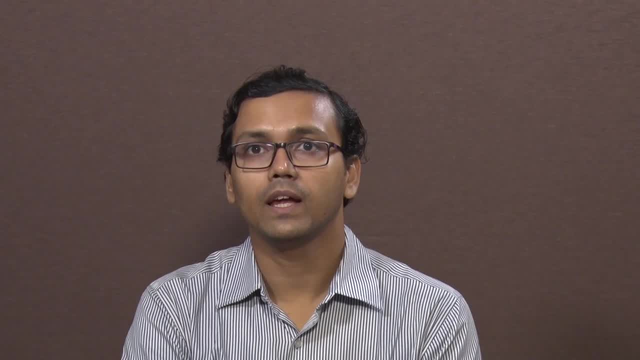 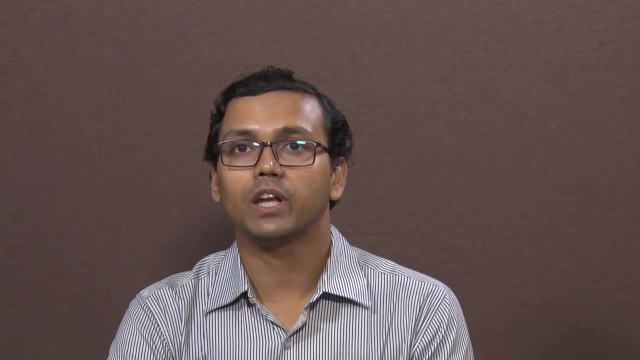 Now the first student physically moves to the last student, who is sitting at the back, and hand over the file to him. So, as he is handing over the file to the last student, that is again an instance of conduction. but in between, what has happened? that is that advection. 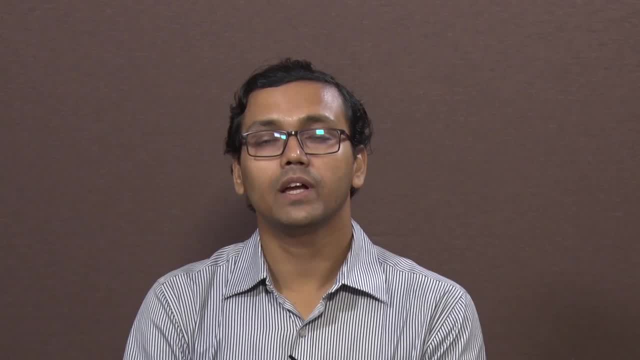 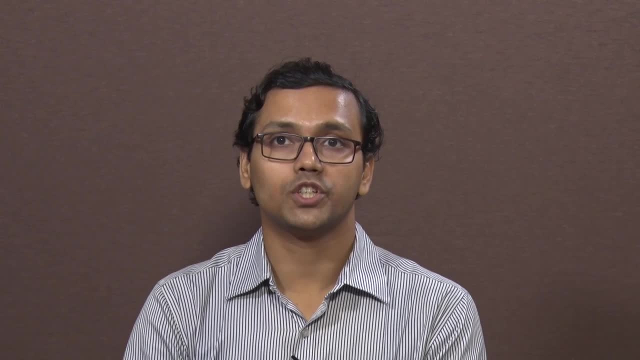 The student has physically moved. The student has physically moved and that is the carrier has physically moved from one position to another position and accordingly we have got the energy transport. so that is convection, and convection is always have both conduction and flow associated with this. 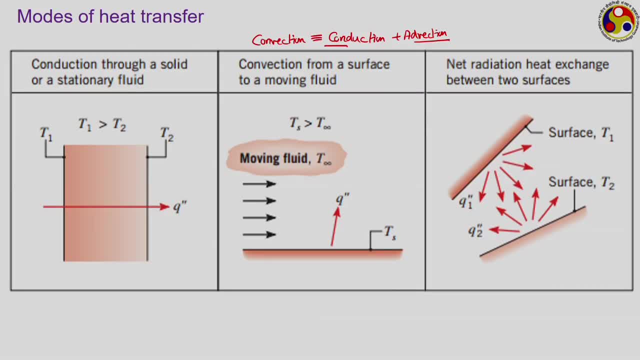 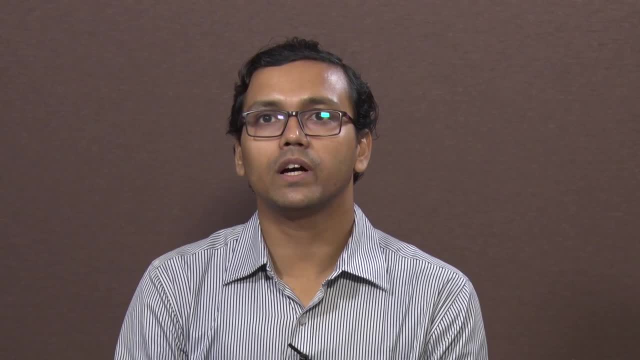 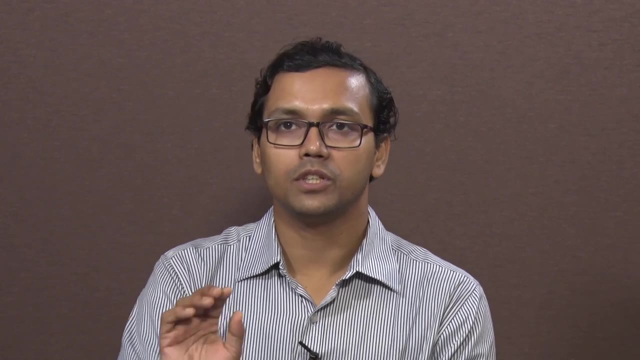 Then what is the third mode? that is, radiation. radiation is somehow I throw the file and it reaches the last student. Then I am completely ignoring the presence of all the 49 students sitting in front of them, I am completely ignoring the medium in between and I am able to reach the last students. 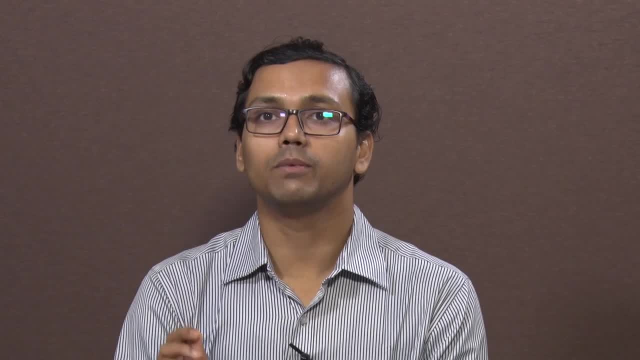 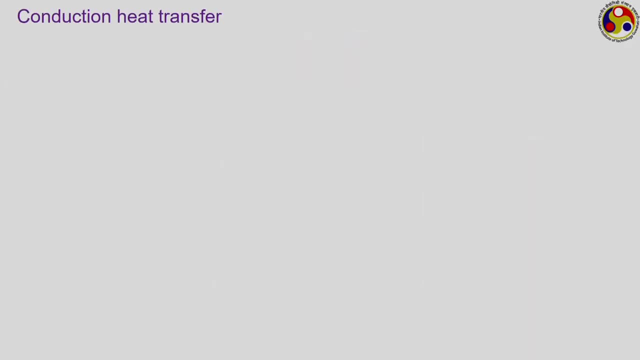 Of course, I have to provide sufficient amount of energy so that it is able to reach the last student. Accordingly, we can have radiation mode of heat transfer. A very brief review of each of them: conduction heat transfer refers to the transfer of energy. 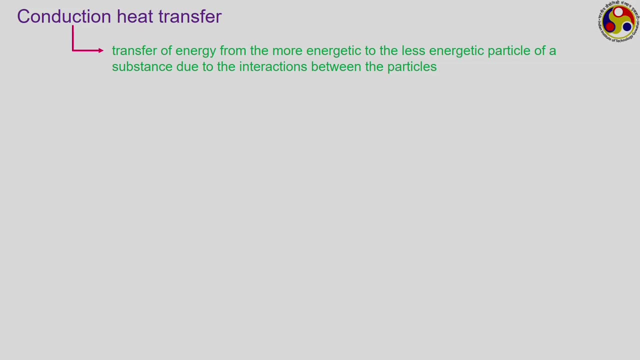 from a more energetic to the less energetic particles of a substance due to the interaction between the particles, just like the example shown here, Suppose. let us talk about a system of gases. Let us talk about a system of gases Where one side of the system is kept at the temperature T1, other side at temperature T2. 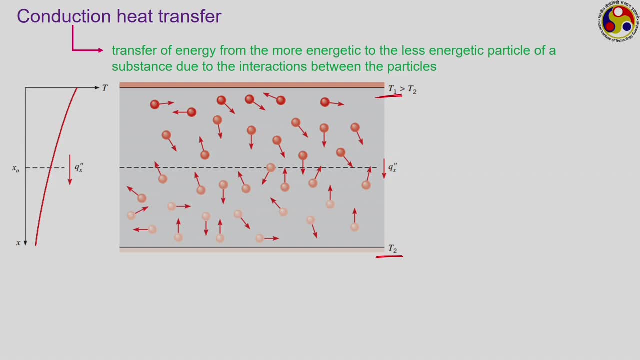 and T1 is higher than T2.. Then the molecules of gases which are close to the surface at T1, which are somewhere here they are expected to be at a higher energy level compared to the molecules which are here close to the low temperature wall. that is the temperature gradient acting here the 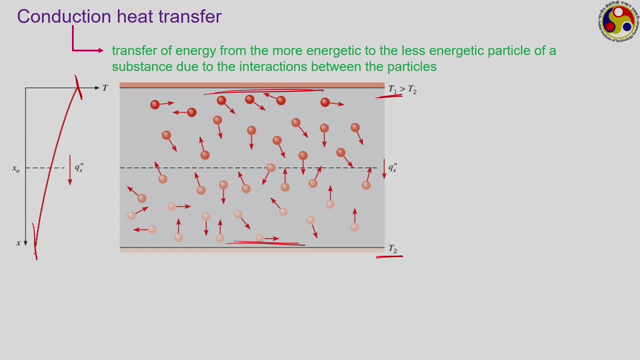 temperature is high here. the temperature is low Now because of this temperature gradient. Now because of the higher energy content of the particles which are in this zone. there are 2 ways energy can get transmitted. Because of their higher energy content, they will be having higher kinetic energy, so they 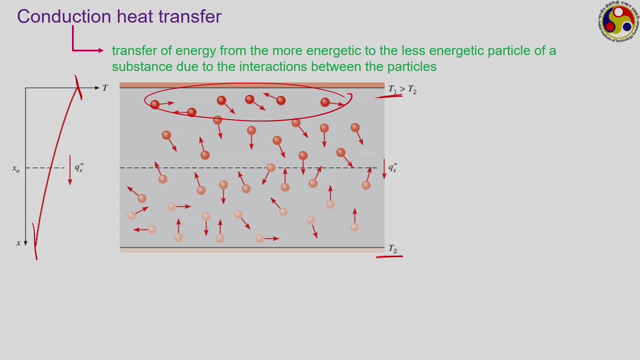 will be having much more movement compared to the low energy particles and, as they are moving over the domain, they will collide with the other particles and whenever such a collision happens, if it is colliding with a less energy particle, it will transfer a part of its momentum to the less energy particle. 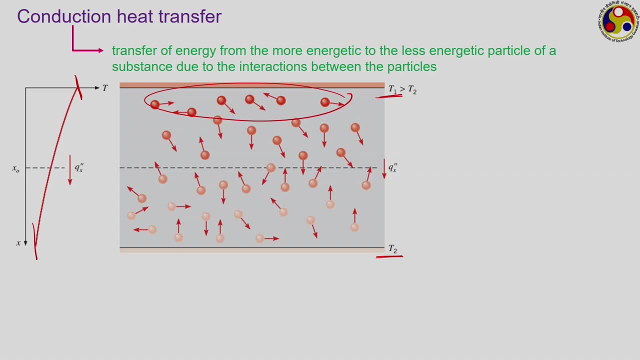 Accordingly, the lesser energy particle will have an uplift in its own energy content. that means an increase in its own temperature. So that is one mode, which is because of the molecular activity or collision of the molecules. There is a second one also, if we take any plane within this domain, like the dotted line. 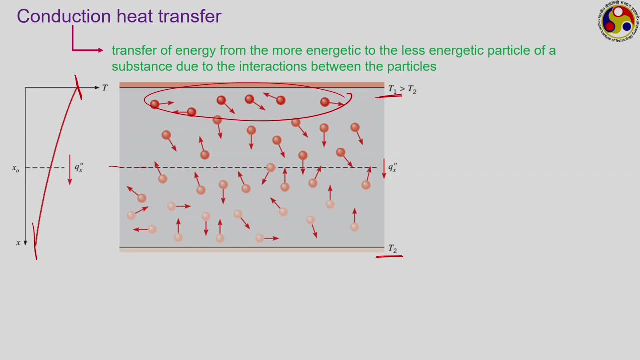 this black dotted line shown here the because of the higher energy content of the particles or molecules. So from the top of this or which are above this dotted line compared to the molecules below this, the number of particles crossing this line from top to bottom will be higher. 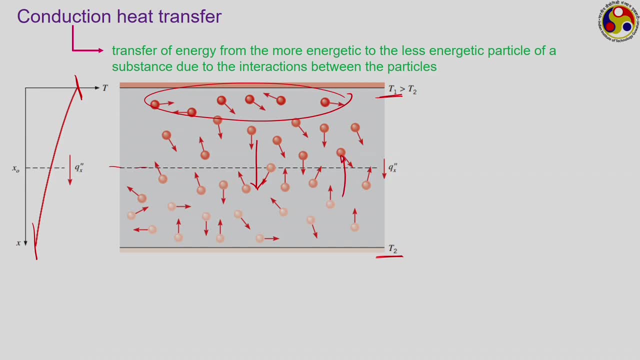 compared to the number of particles crossing this from bottom to top. Accordingly, there is a higher amount of energy transmitted from top to bottom and accordingly we can have energy transmission. So this is what we have in case of conduction 1. So in case of conduction, at least associate the gases where we have. we can see there. 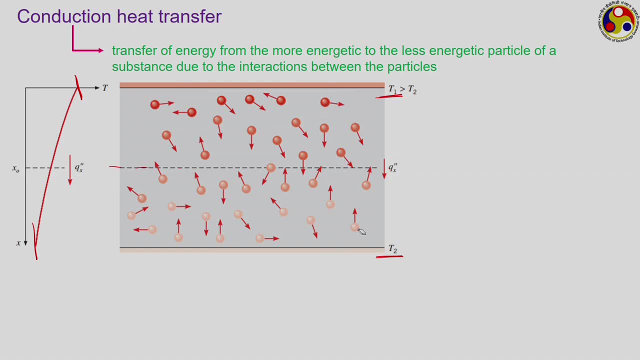 are two primary mechanism going on. one is the collision of molecules and second is the advection or physical movement of these molecules. When you go to liquids there, the liquid molecules are not allowed to move such freely, So the collision is dominant. but liquid molecules also can move to certain degree. 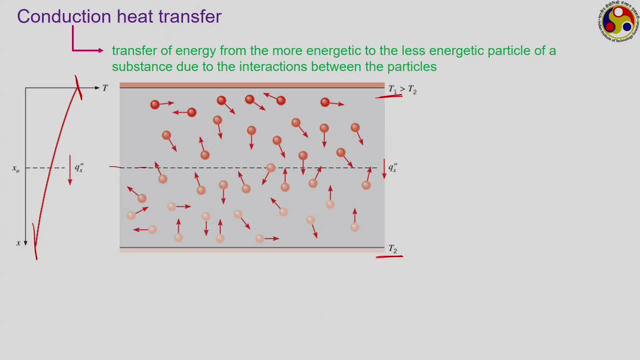 And when you finally move to the solids. in case of solids, generally, molecules are arranged in a particular lattice structure, So they are not allowed to move at all, but they can keep on vibrating at their own position and because of their vibration they keep on transferring it to the neighboring particles. 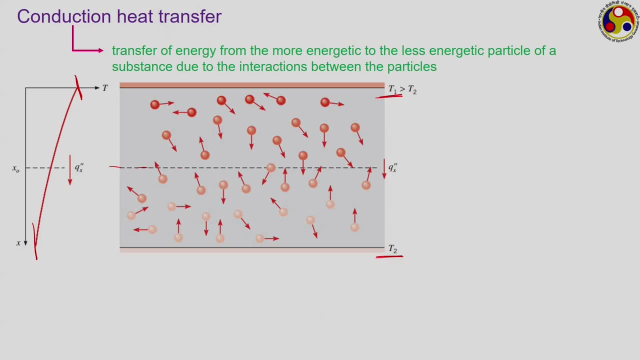 just like the example of student sitting in a class and passing on the file that I mentioned, And accordingly it will be able to transfer energy from one end of the lattice structure to other end. So there the collision or vibrational energy based transfer, is more dominant. there is 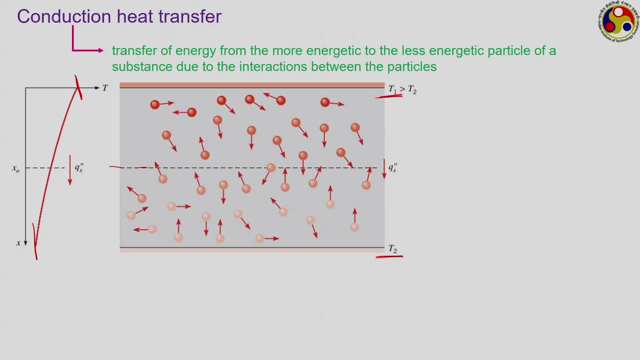 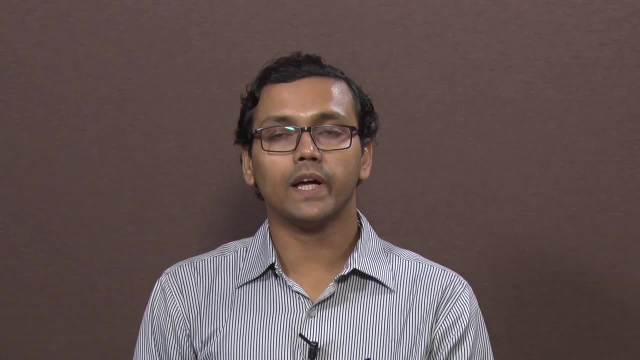 hardly any molecular movement in case of solids 2.. So in the case of gases the molecular movement is the most dominant one, And also for solids. we can have two kinds of solids. If we are talking about non-conductors, then the one that I mentioned that is predominant. 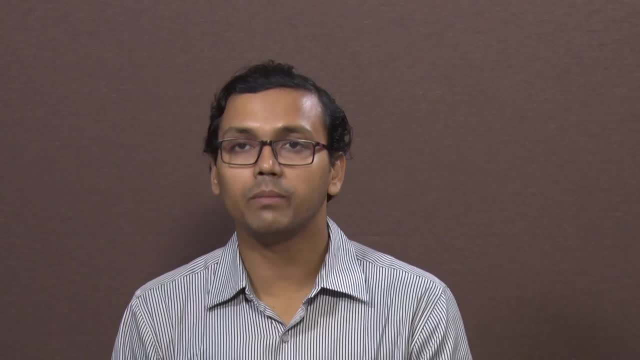 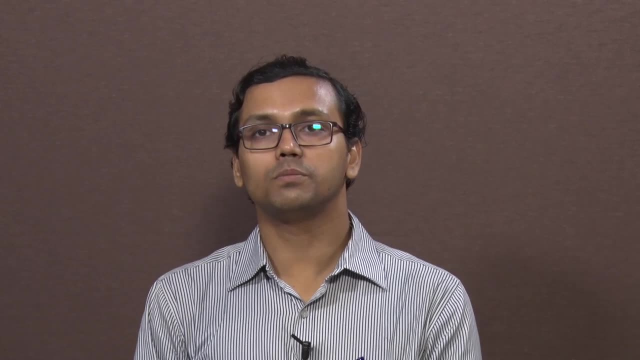 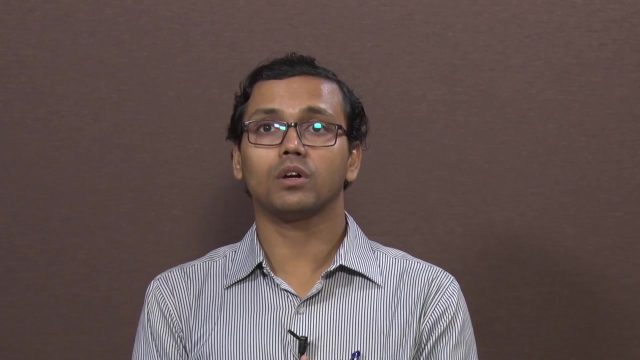 that is, the vibrational energy being transmitted to neighboring molecules. But for conductors, which can have significant amount of free electrons, we can also have energy transmission because of the movement of the electrons. So for conductors we can have solid conductors, we can have energy transmission or conduction. 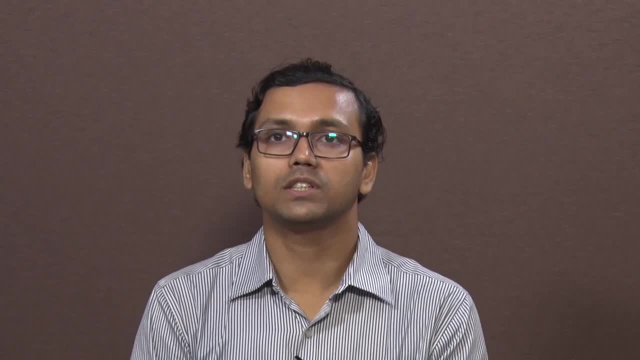 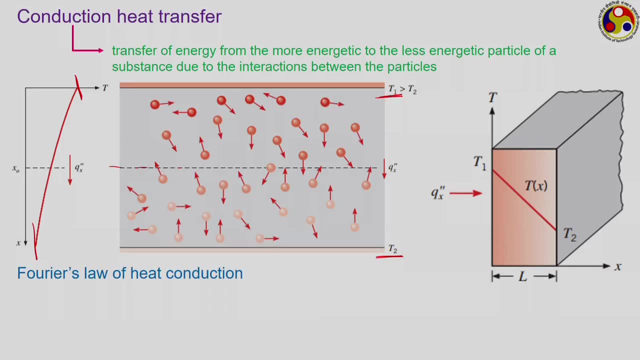 energy transmission By both molecular vibration as well as the transmission of free electrons. So to understand the mechanism of energy transmission, let us say through a solid by conduction. say: here the temperature is T1,, here the temperature is T2 and the length of the domain is L. then 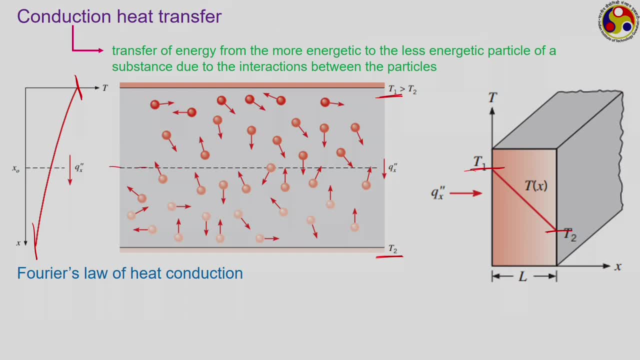 there is a temperature gradient acting across this and the fundamental law which gives us an idea about this particular law: 3.. So for the amount of heat transmitted in this direction, from the wall at temperature T1 to the wall at temperature T2, is a Fourier's law of heat conduction which says that the 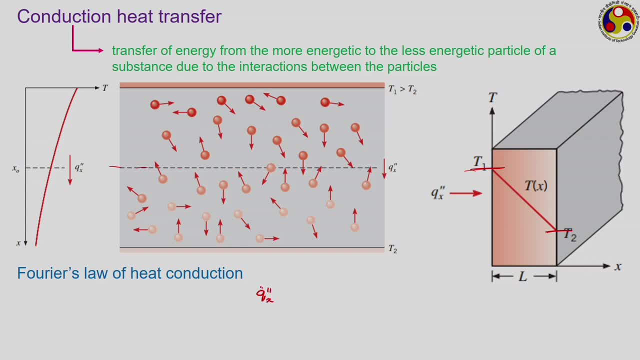 heat flux: q, dot, x double prime- let us put the dot to indicate the rate- is proportional to the temperature gradient which is acting in the x direction. This is the most basic relation or basic form of the Fourier's law of heat conduction. In the next week we shall be talking in detail about energy transmission. 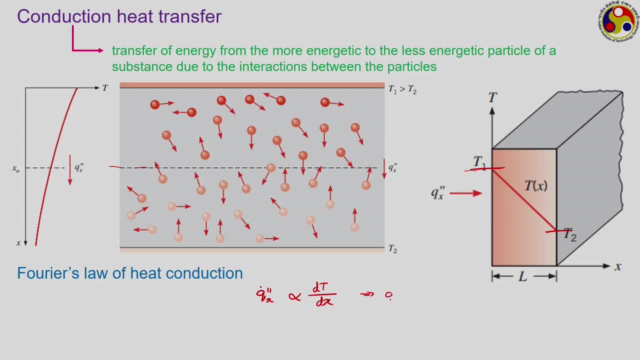 Thank you. Let us see what is the heat flux in its more generalized form. So if we want to convert this one to an equality, the conduction heat flux in the x direction will be equal to k, dT, dx, where k is some constant of proportionality which is called the thermal. 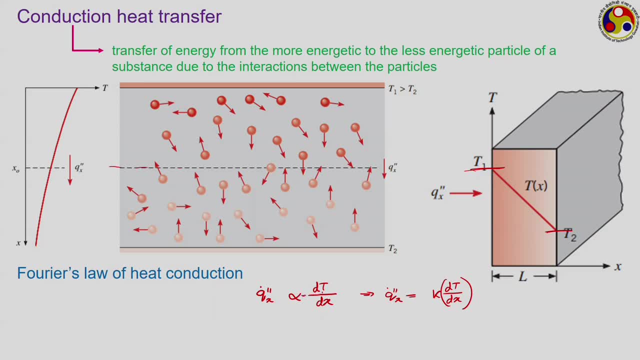 conductivity. it is a property of the material and actually we should put a minus sign here, because heat is flowing in the direction of reducing temperature, so in the direction of increasing x. T is, as x is increasing, The heat flux is reduced. So you see what is the heat flux. 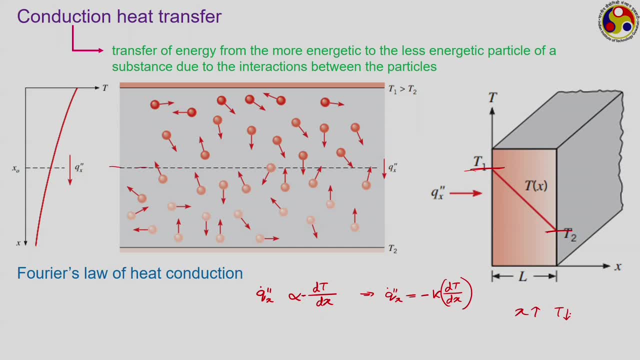 T is decreasing. So to have a positive value of dT dx, we should have the minus sign for this. So Fourier's law of heat conduction is the fundamental equation with which conduction heat transfer starts. Second fundamental mode is the radiation heat transfer which talks. 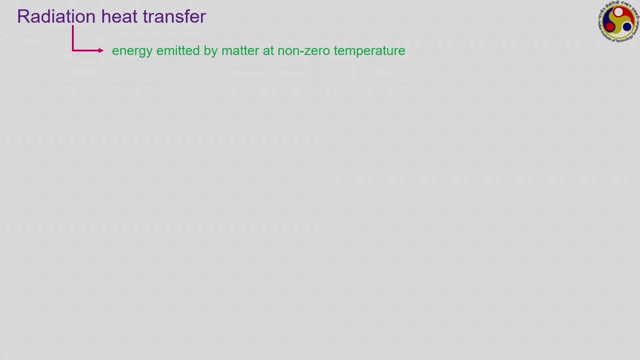 about the energy emitted by any matter which is maintained at a temperature higher than zero. Here the mode of emission or mode of energy transmission are electromagnetic waves, and it is completely independent of any medium. Even if any medium is present, from the source to the destination, it can completely eliminate the presence of the medium, and it is the 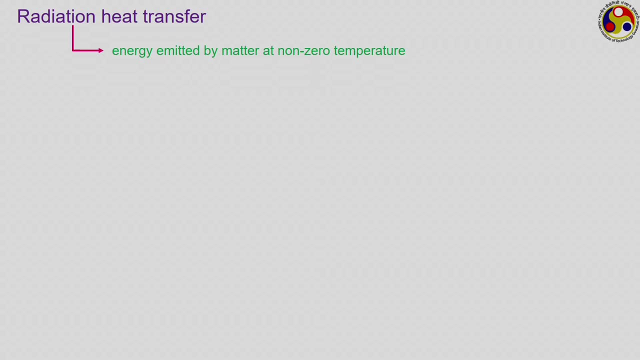 it is best when the medium is vacuum. Basically there is no medium at all. The Stephen Boltzmann law of radiation is a fundamental equation which gives us an idea about the radiative mode of heat transfer, where which talks about, say, for a perfect substance, the total heat. 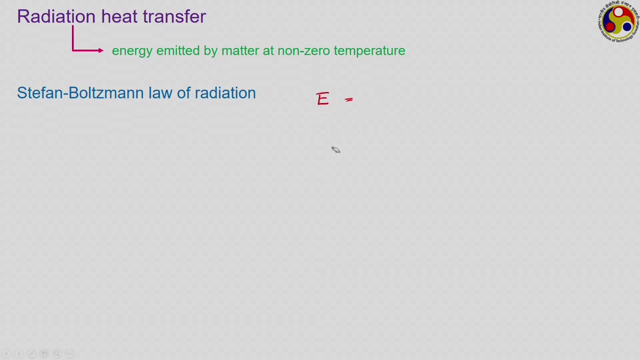 transfer. The total amount of energy transmitted can be written as: a total amount of energy emitted by radiation is proportional to T to the power 4, where T is the absolute temperature or it is equal to some constant of proportionality into sigma to the power 4, sigma into T to. 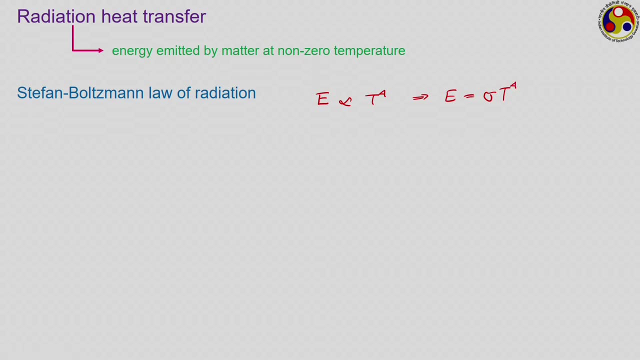 the power 4, where sigma is called the Stephen Boltzmann constant. This is for the ideal substances or black bodies for real substances. So that is why we put generally put it like this, We put a subscript b For real substances. we generally have some an term, epsilon, which 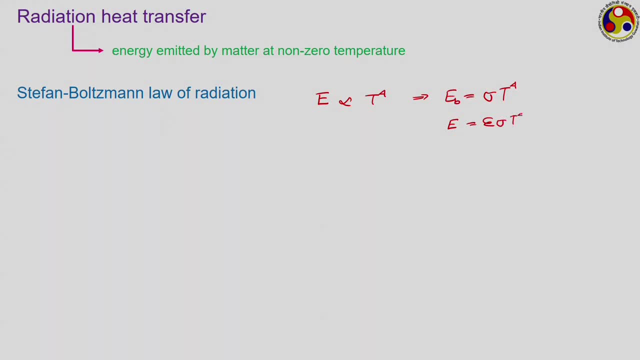 is called emissivity, coming into picture, epsilon, into sigma, into T, to the power 4.. For the moment you just take the relation. the details of this one I shall be coming later on- Like the Fourier's law of heat conduction mentioned in the previous slide, 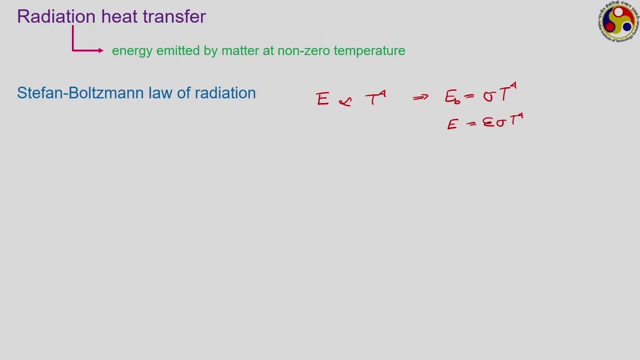 that is a phenomenological law, that it does not have any mathematical background. it has come just from observation. But, Stephen Boltzmann, law of radiation can be proved from mathematical, mathematical law. So that is the mathematical point of view which we shall be doing in the concerned module. 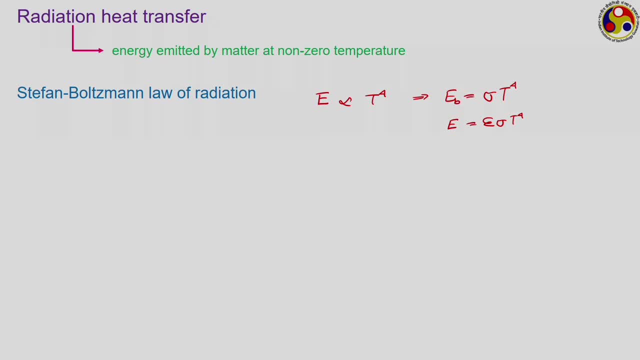 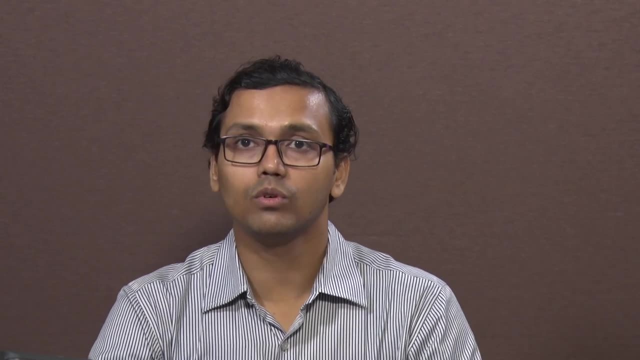 For the moment you can just have the relation, that is, the total amount of radiation energy emitted by a substance maintained at absolute temperature. capital T is given as epsilon sigma into T to the power 4, where epsilon is called the emissivity and its value can. 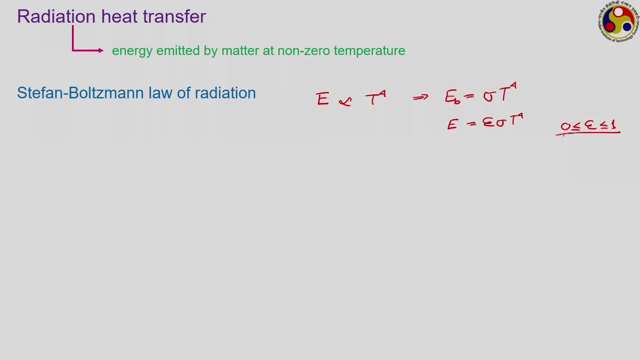 range between 0 to 1.. We shall be having detailed discussion about the nature of this emissivity, different types of emissivities and also the difference between black bodies and real substances. Thank you. 1 Now because of radiation. while a particle, or I should say a surface, can emit radiation, 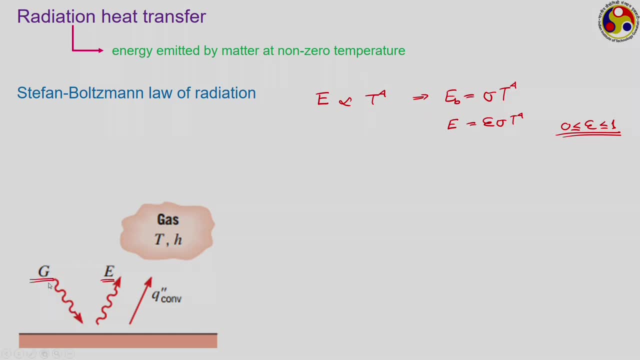 like this one, it can also receive a radiation from its surrounding, So, accordingly, this capital G is a symbol generally is associated with a term called irradiation. Irradiation refers to the amount of radiation energy received by a surface from its surrounding, So, as the 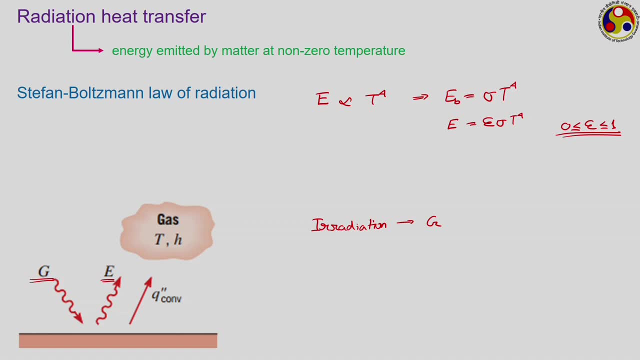 surface is giving E amount of energy. it is also receiving G amount of energy and if there is some convection happening because of some gaseous medium flowing over the surface, then we can easily write an energy balance for the surface shown here. It is receiving G. 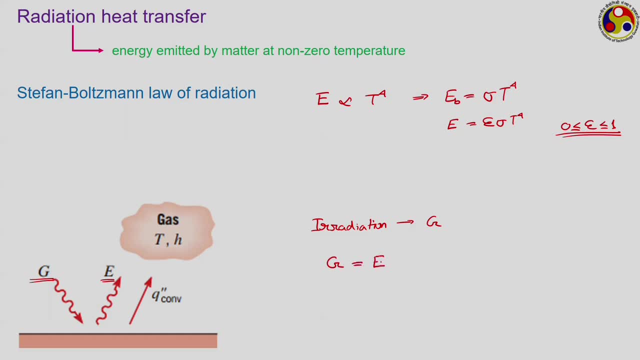 amount of energy, and under steady state this should be equal to total amount of radiation energy emitted by this, plus total amount of convection energy lost by this. So here all this G and E. they can be written in flux mode Or they can also be written in heat rate mode. We shall be discussing in detail about each. 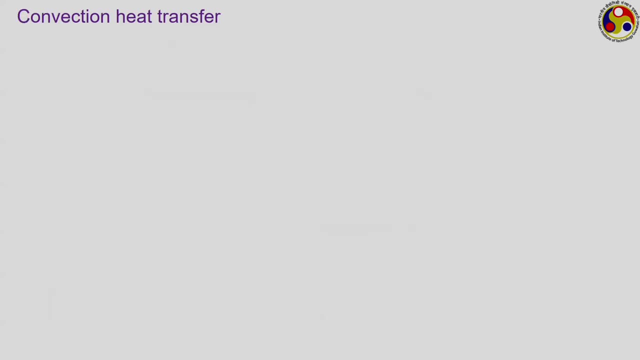 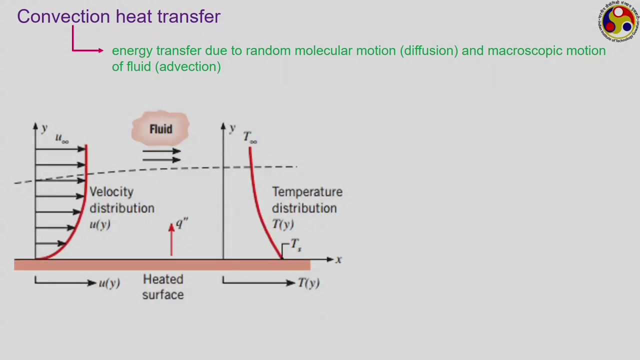 of them later on in week number 9.. The third mode of heat transfer is the convective heat transfer, which talks about the energy transfer due to random molecular motion, which is diffusion, and microscopic motion of fluid, which is advection. We are particularly concerned about convective heat transfer at the interface. 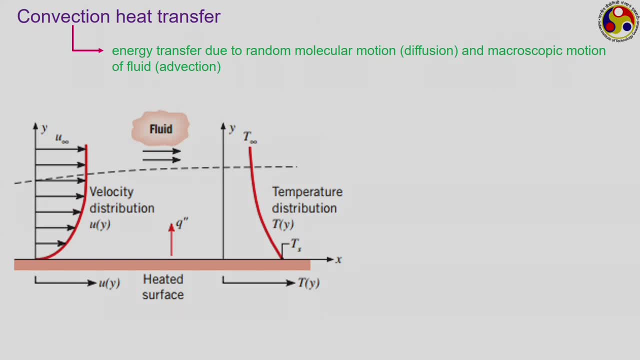 of a solid and a flowing fluid, Just like the situation shown here. we have a heated solid plate, It is maintained at certain temperature and a fluid is flowing over this. As the fluid is flowing over this, it will be picked up energy from this. that is, the fluid molecules. 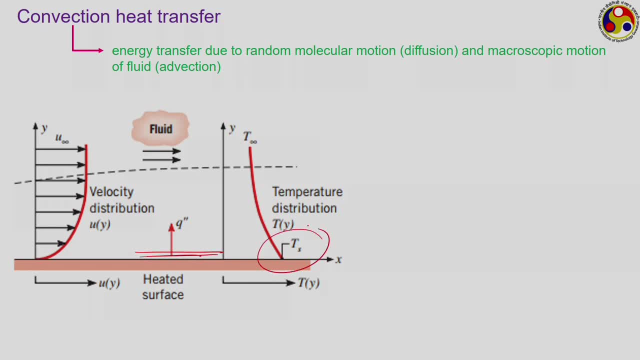 which are very close to the surface, They will try to attain the solid surface temperature, that is, Ts, where the fluid itself may be coming with some free stream temperature: T infinity. So as we are moving away from this, in this direction, the temperature of the fluid will 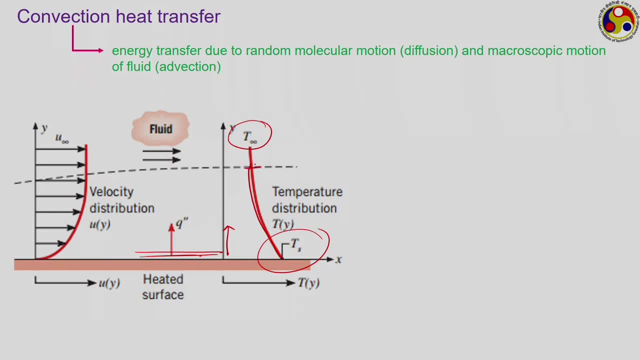 keep on reducing. Finally, it will reach this free stream temperature, thereby creating a connection to the thermal boundary layer, This particular zone of rapid temperature gradient, which is called the thermal boundary layer. Convection is a very involved subject: The total convective heat transfer associated. 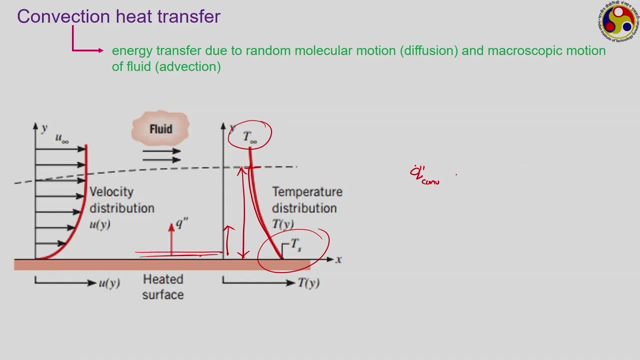 with this situation is generally found to be: the corresponding convective heat flux is found to be proportional to the effective temperature difference, where Ts is the surface temperature and t- infinity- is the final temperature. There are two regions in here. The top one is the end of the sphere and the bottom one is the end of the sphere. The left one is 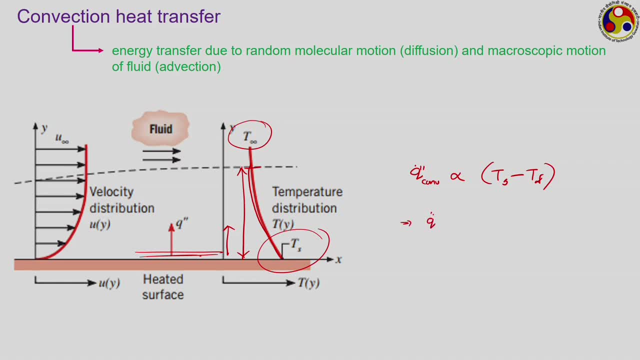 the end of the sphere and the bottom one is the end of the sphere. So this is the end of the final temperature of the fluid. or, converting this to equality, we can write this: convective heat transfer or convective heat flux is equal to some h into Ts-T infinity. 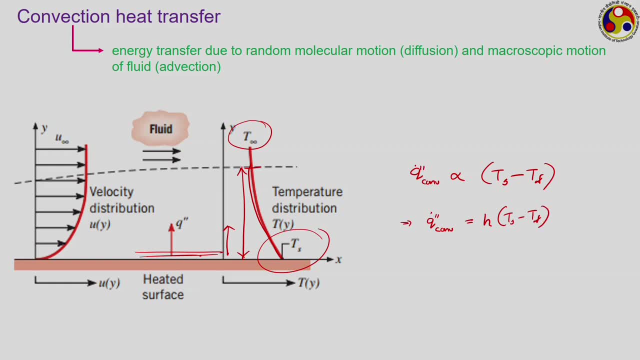 I have earlier used this small h to indicate specific enthalpy, but in this course we are not going to talk about enthalpy anymore and therefore I shall be using this small h as this constant of proportionality, which is also called the convective heat transfer coefficient. 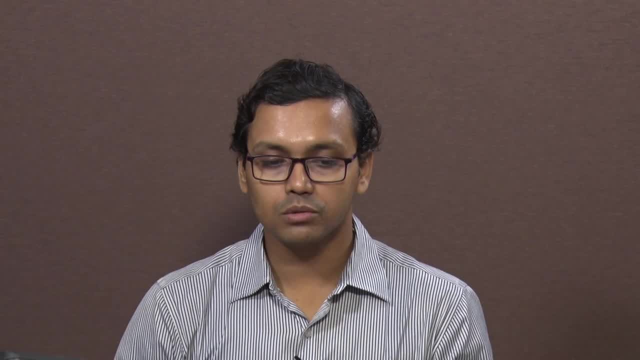 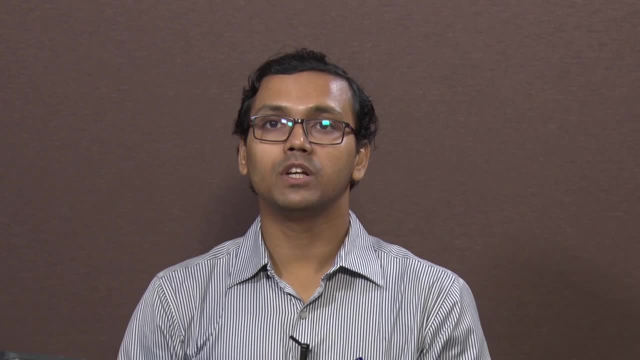 Whereas this course we are going to talk only about conduction and radiation, so we are not going to discuss anything about the convective heat transfer. but this convective heat flux equation may be repeatedly coming to picture, So we have to understand that the convective heat transfer will be coming into equation.